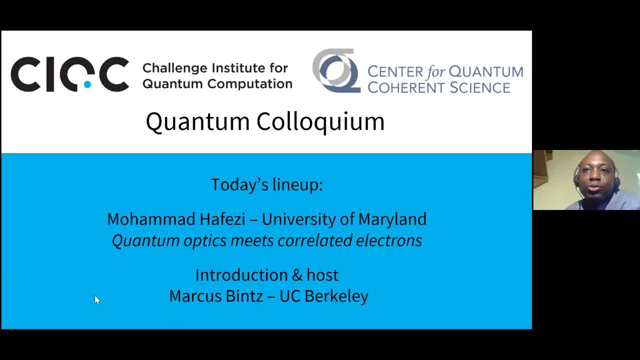 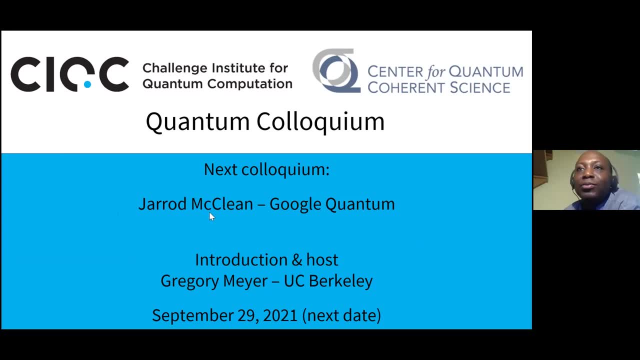 Research Young Investigator Award. So just a quick reminder for next week. So the colloquium next week will be by Gerard McLean from Google Quantum and the introduction will be done by Gregory Ayer. So I will just quickly also remind us of the structure of the colloquium. So the first 20 minutes 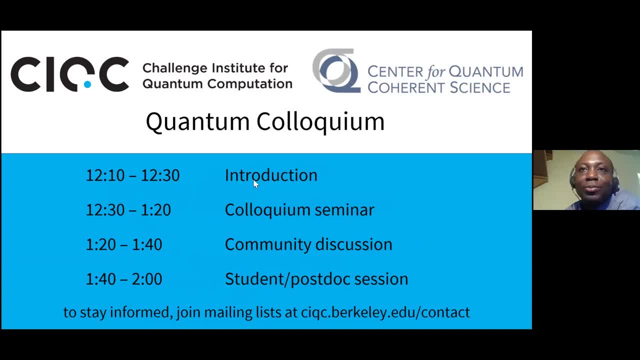 will be an introduction to the notion that we need for Mohamed's talk. So that will be done by Marcus, as I said, And then the seminar and we'll have after that a discussion for about 20 minutes. So, very importantly, after this discussion, the student and postdoc will remain. We stay here with 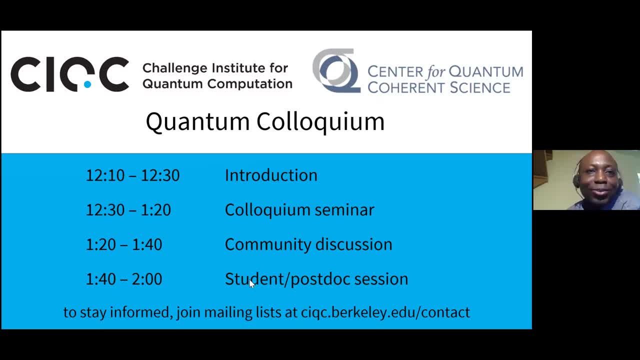 Mohamed for more discussion, And at that point I will ask that the PI leave the Zoom call. Okay, so with that. so the floor is yours, Marcus. are you here? Yeah, I'm here, Thank you. Yes, Great, Let's see if we can properly share screen. 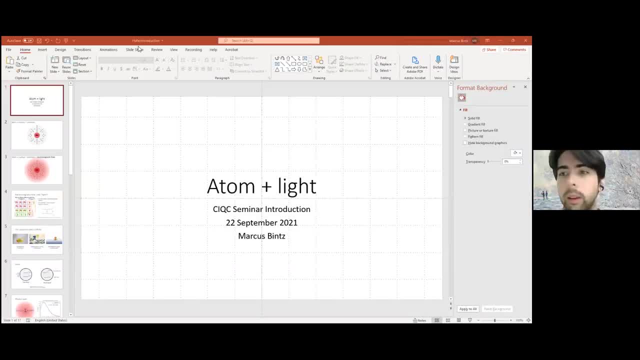 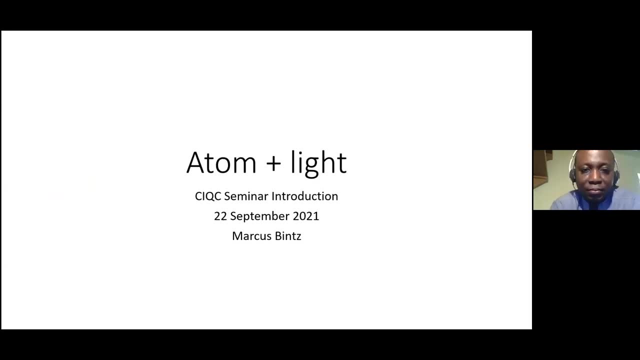 It was working earlier and I hope it's still working now. It seems to be Okay. Yeah, so, as Bobakar has told us, Professor Hafezi will be discussing some applications of quantum optics techniques to strongly correlated electron systems. So for this. 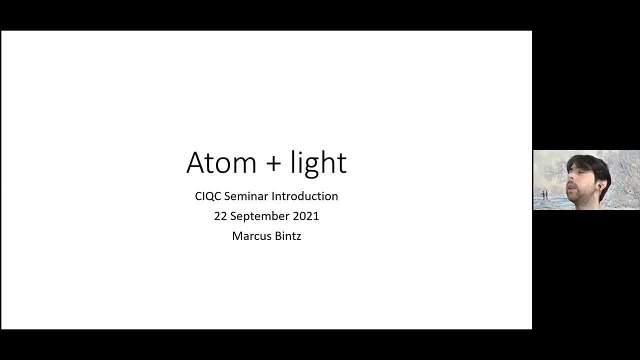 introduction, since I think, looking at the past CIQC talks, there hasn't been too much on this quantum optics topic. I think that's sort of I wanted to give a bit of a blitz overview of some of the issues that we'll be looking at in the next slides. So so I think that's sort of I wanted to give a bit of a blitz overview of some of the 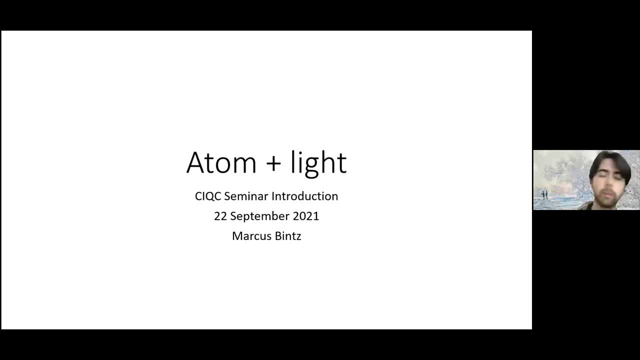 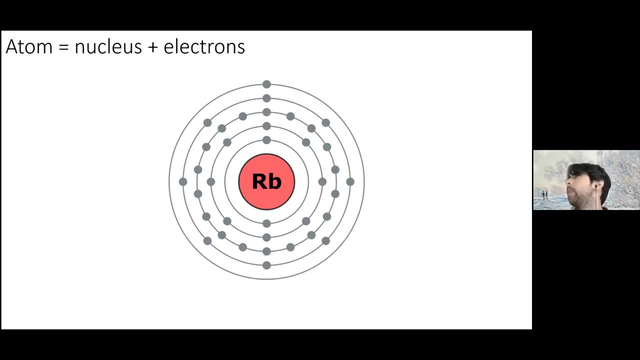 essential ideas and techniques that have come from this field over the past almost century now. So one motivation to think about quantum optics is the fact that in the world we live in all of the materials that we would build a quantum computer out of, or, you know, even something. 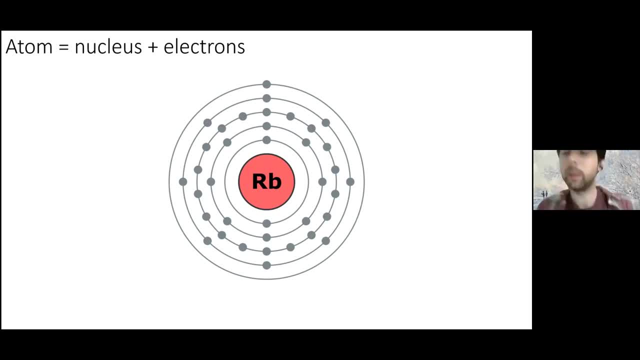 much simpler, like a chair there tend to be made out of atoms or, you know, more generally, out of some nucleon electrons, and pictured here is a rubidium atom which is neutral. it has no net charge and so it's thought to be. you know, it's generally regarded as something that's you know. 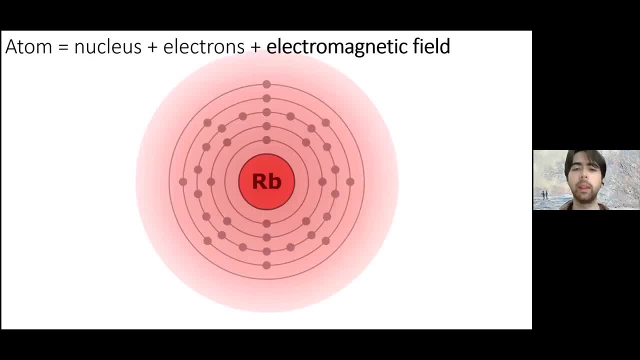 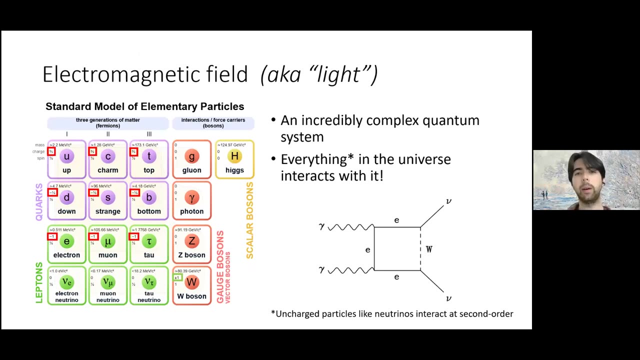 very weakly coupled to the environment. Nevertheless, you know, any atom is is not just its nucleus and the electrons attached to it, but also the electromagnetic field that binds the the whole thing together. And the thing about the electromagnetic field is that it's not always nuclear, it's not always neutral. You know, if you look at the 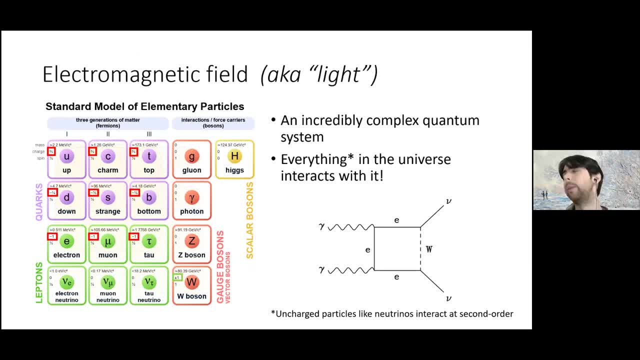 as I said, an incredibly complex quantum system pervading all of the space around us. It's, you know, some huge assortment of quantum modes that are, you know, very complicated And everything in the universe interacts with it. you know, either because 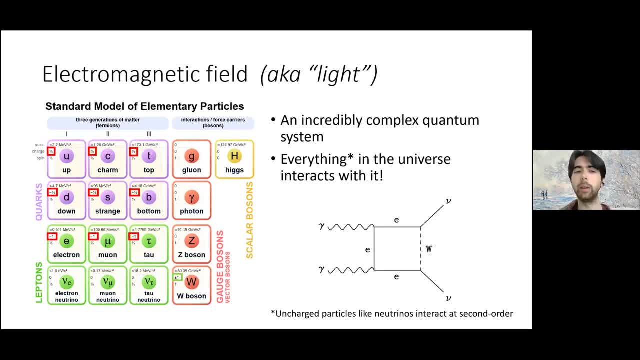 it has some direct electric charge, like you know, a fundamental electron or a quark inside a nucleus, so basically all material stuff. but even more exotic particles that particle physicists think about, like neutrinos, will also, even if somewhat indirectly, interact with. 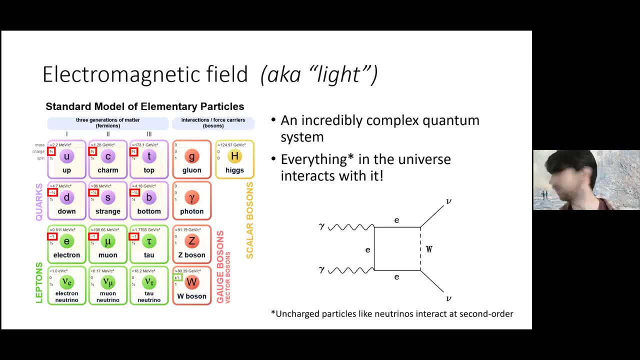 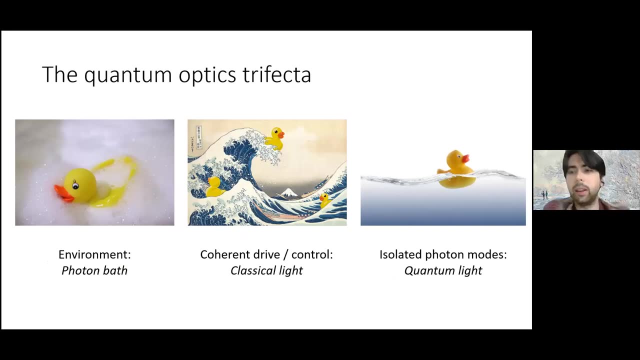 the electromagnetic field. So there's this giant quantum system that is just out there and we should try at some level to think about. you know how it affects the more controlled stuff that we normally prefer to think about. So there's kind of, I think. 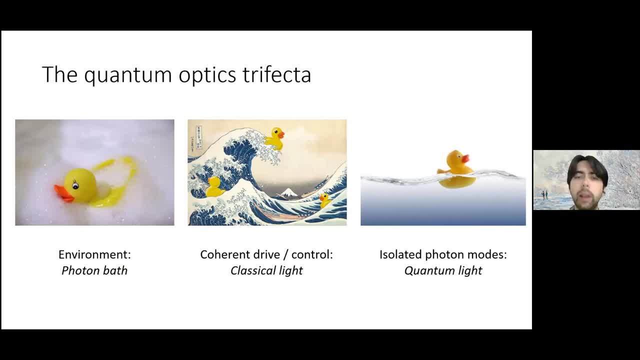 three main themes of the way that this electromagnetic field can influence your system, your material system. The first is by acting as some environment for the system under consideration, and this is like a photon bath. You have this huge set of modes and you know there will be some. 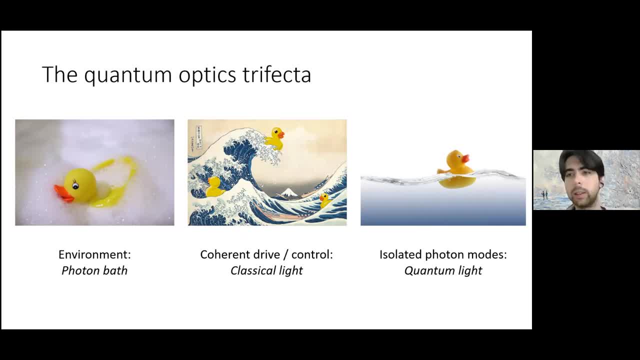 interaction between them. The second idea is to use just some classical light, So to kind of forget about the quantum nature of the electromagnetic field and just realize it's some tool that you can use to control or drive your system. And then the last thing, and probably 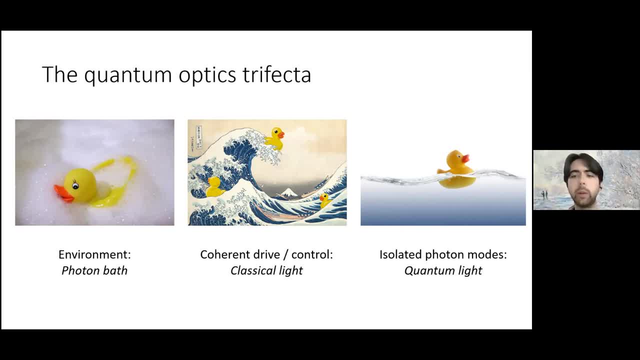 the most interesting is to actually sort of directly make use of the quantum nature of light and try and isolate from this huge, many body quantum field some very well-controlled, isolated single photon modes. So these are the three general things that I'd like to give some simple introduction to in this part. 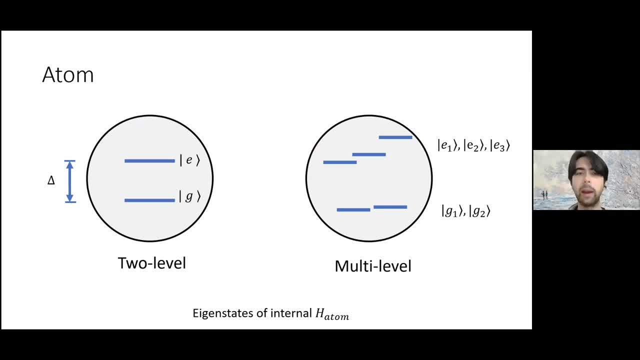 So first, before going into that, let me go back away from the electromagnetic field, just to the atom, And I'm going to work with a very simple abstraction of any atom or any qubit really, where either I'll have some two-level system where the lower energy state I'll label by G for ground. 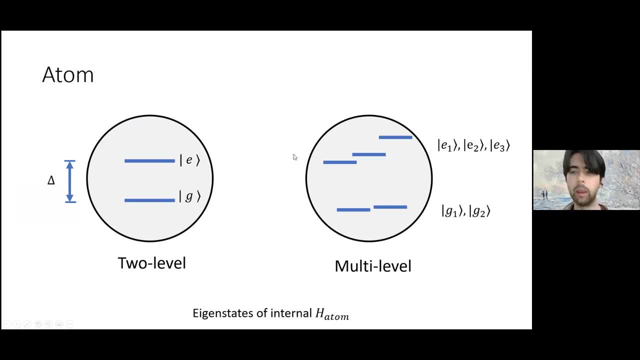 and the higher energy level, one E for excited or, you know, maybe some more complex multi-level system. So I'm going to basically totally forget about any internal properties of the atom or the material and just assume that I can have direct access to the eigenstates of that interaction. 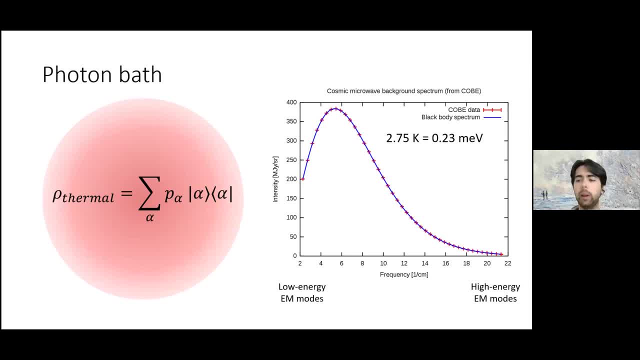 So the first thing to try and add on to the simple internal atom picture is the photon matrix. So when you think, one way to think about the nature of the electromagnetic field is that it's some, typically some thermal distribution of many different modes. So the direct nature of 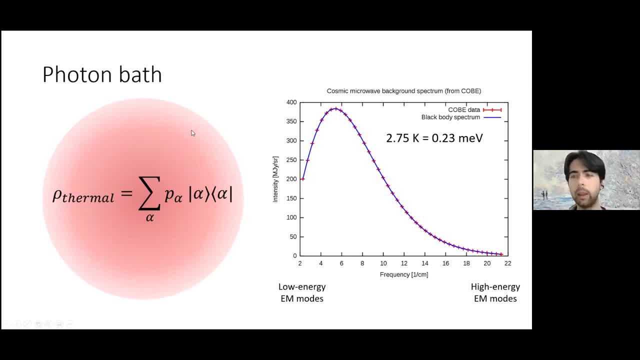 these modes isn't really super important here. It's just some quantum mechanical system with several, with many, many, infinitely many energy eigenstates And the density matrix for that system is some incoherent superposition overall, All of those with some probability. 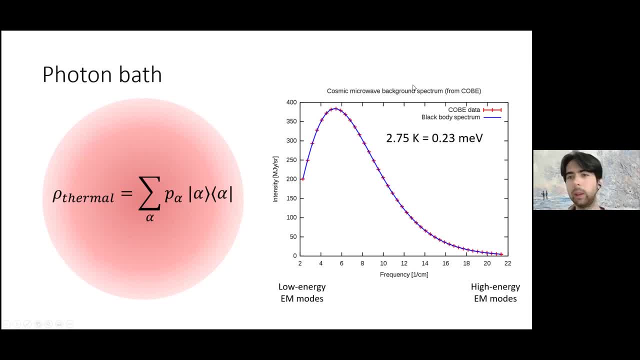 So, for example, the background radiation of the universe is in the microwave part of the spectrum And if you look at how the energy is distributed between the lower energy modes of the electromagnetic field and the higher energy modes of the electromagnetic field, it forms this very 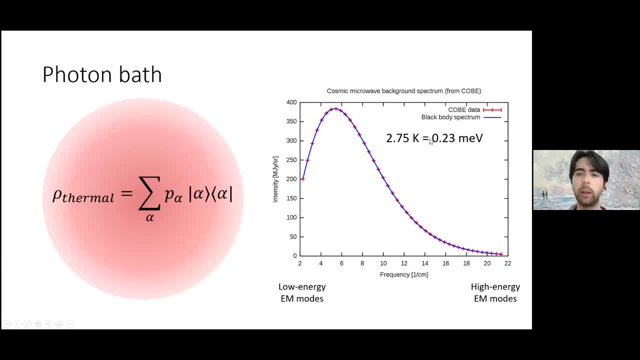 characteristic Planck distribution that peaks around 2.75 Kelvin or 0.23 millielectrons volts. so this is kind of the very baseline cold temperature of the universe around us, minus anything like the sun or the earth that adds additional heat and into the electromagnetic field. 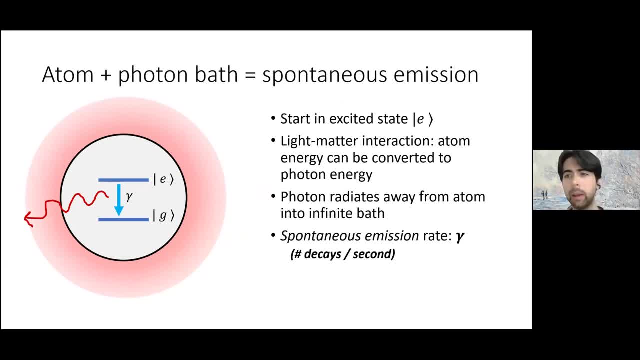 so what happens when you add this photon bath onto your simple atomic system? the sort of first, most important thing that happens is spontaneous emission. so if you have your quantum system, your atom, starting in the excited state, the light matter, interaction between the atom and the photon will allow energy to be converted from this internal excited state of the atom into 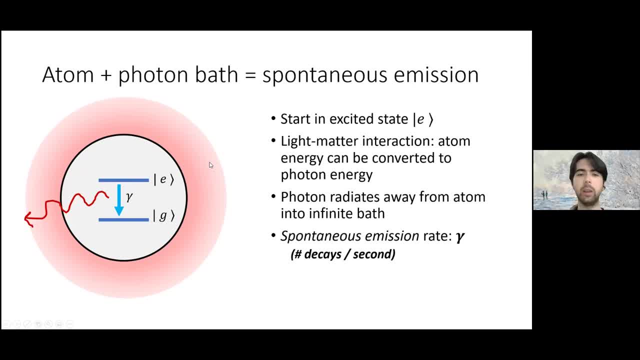 photon energy, because the bath is so huge that light energy will just immediately be radiated away and the atom no longer has access to it. so this is known as a spontaneous emission. so at some rate your atom will, due to the coupling to the bath, just decay from the e state. 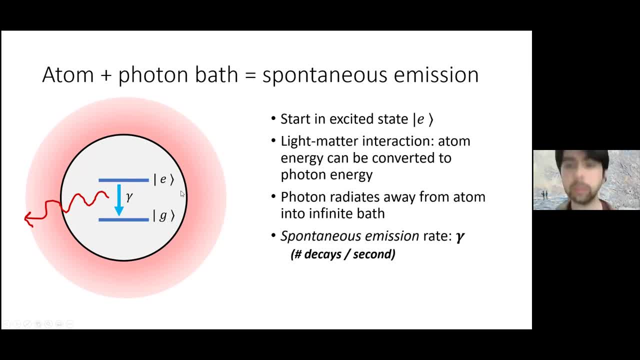 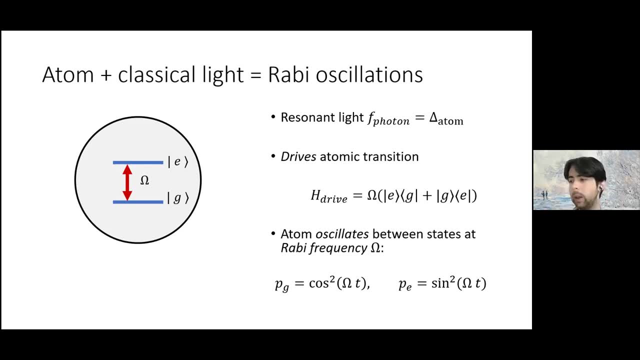 to the g state, and this rate is typically denoted gamma. okay, so that's, i think, all i want to say about the photon bath for now. so maybe a little more interesting is what to what classical light does. so here it's again. i'm not really thinking too directly about, you know, the electric or the 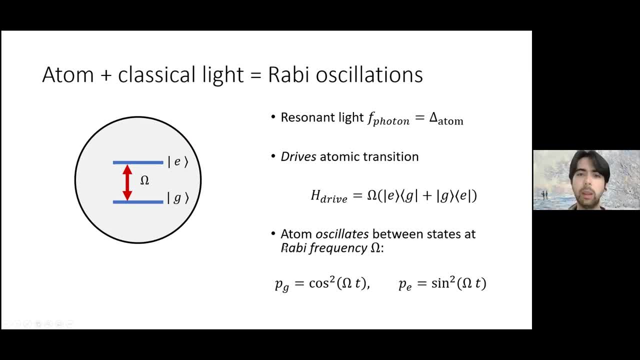 magnetic idea of the en field. it's just, i have the ability to apply some light that is at a frequency that's resonant with the transition between the ground and the excited states of the atom, and if you apply this resonant light to the system, it will. 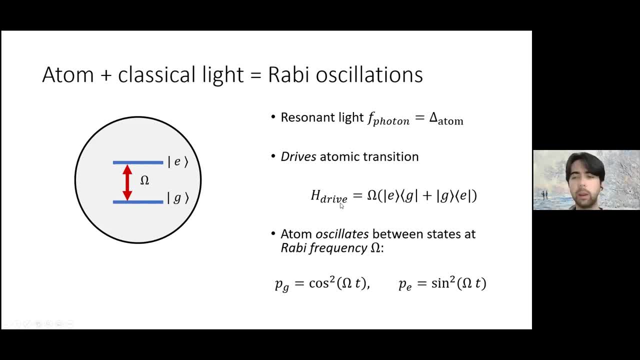 drive, the, the atom. so you can think of this as adding to your the hamiltonian that governs the dynamics of the system, some just simple drive term. so here you'll notice there's no information about, like what the state of the, the light is at all, it's just. 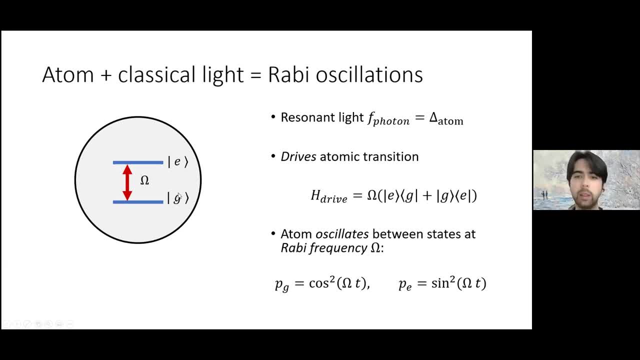 some external field that i'm adding that causes the system to oscillate at some set frequency, omega, between the ground and the excited state. So if you track the, say, probability to of the atom to be in the ground or excited state over time, it will, you know just. 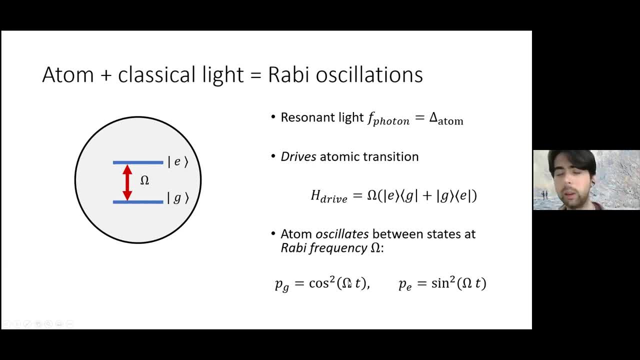 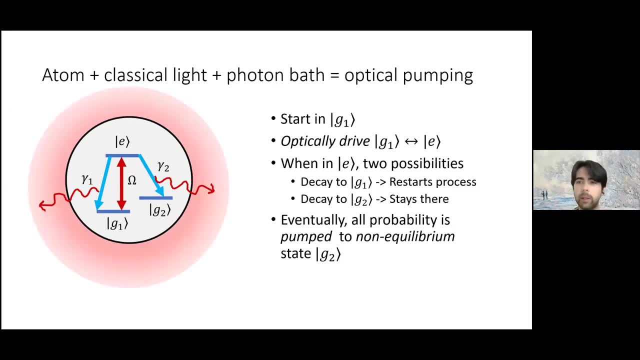 oscillate at this Rabi frequency. so you'll get these, you know, very characteristic cosine squared and sine squared oscillation, oscillations of the probability. All right, now we're going to add back in our photon bath ingredient and we can do something interesting with this. So, in addition to 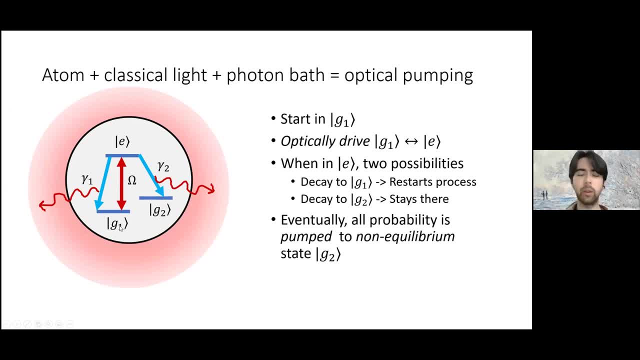 having the atom and the drive and the photon bath. I'll also consider a slightly more complicated atom that has two low energy states and one higher energy excited state. So using these three very simple ingredients you can do something pretty cool called optical pumping. So the idea of this, 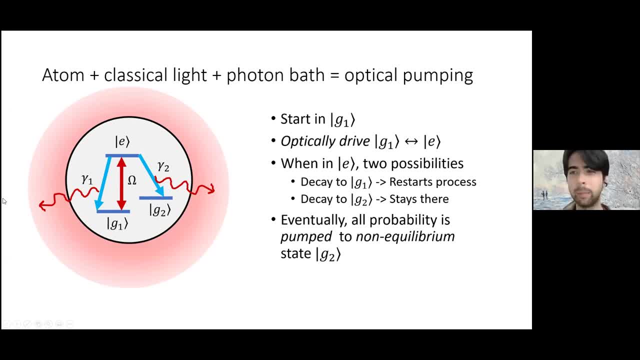 is the following: you and it. like I'm not really saying anything about quantum mechanics at all here, you'll notice. So if I start in this very lowest energy state of the atom g1 and I apply this optical drive omega, so like before, you know, without talking about the photon bath, it would just oscillate. 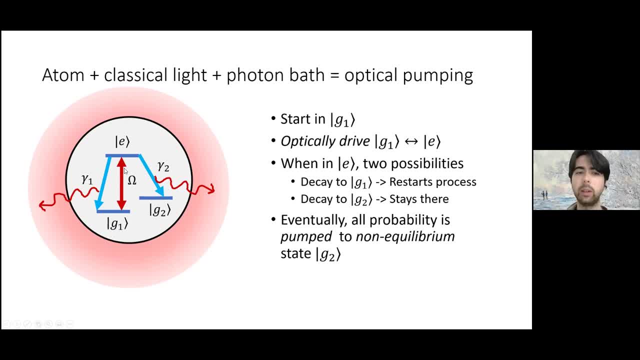 back and forth forever between this g1 and the c, just going back and forth. But because of the photon bath this e state is not stable. it can radiate away the photon and it has two sort of paths. it can decay. One possibility is you pump the atom up from the g state to the e state and then it decays back. 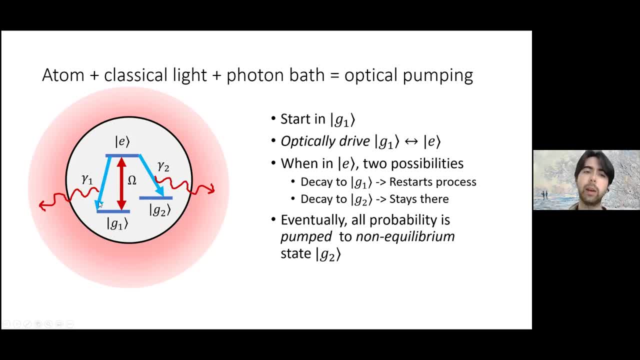 down to the g state, g1 state along this path and you basically restart the process. So nothing really interesting has happened. you've just started here, oscillated for a while and then decayed back down to where you started. Something that's more interesting is if you is, if you. 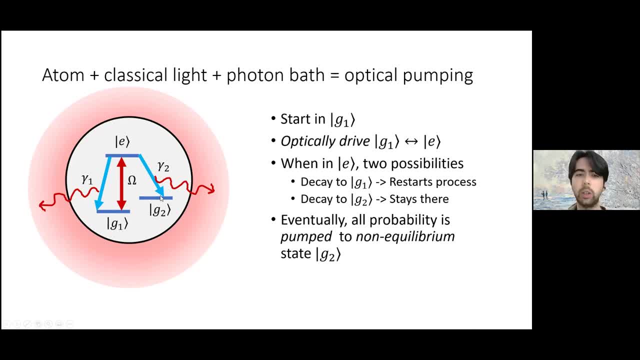 oscillate up to the e state and then decay down into the g2 state. So now, because there's no draw i that goes between the g2 and the e state, you'll just stay in this g2 state for a very, very long time. Eventually you'll decay back down into the g1 state, but usually the rate at which that happens, 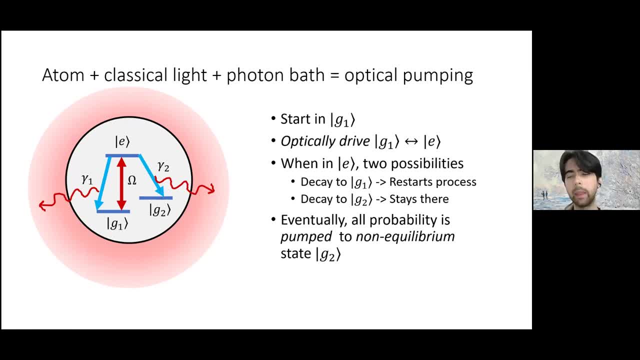 is much, much slower than anything else in your system. I believe in Dan Stamperkern's CIQC colloquium a few months ago he mentioned that in rubidium, for example, one of these low at lying hyperfine levels lives for hundreds of thousands of years. 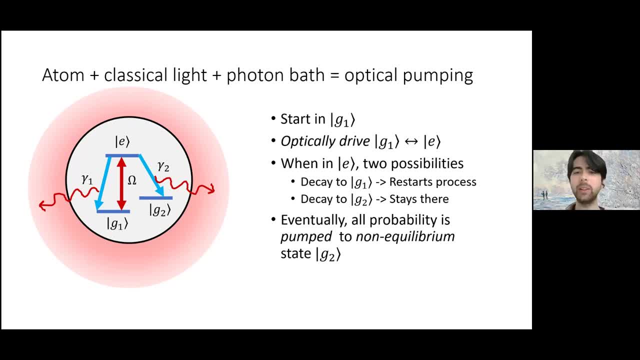 So it's possible essentially to put to pump all of the probability of what of what state your atom is into this non-equilibrium state g2.. So this is you know. in this case that's you know. it's just some other internal eigenstate of the atom, but I believe Muhammad will tell us maybe. 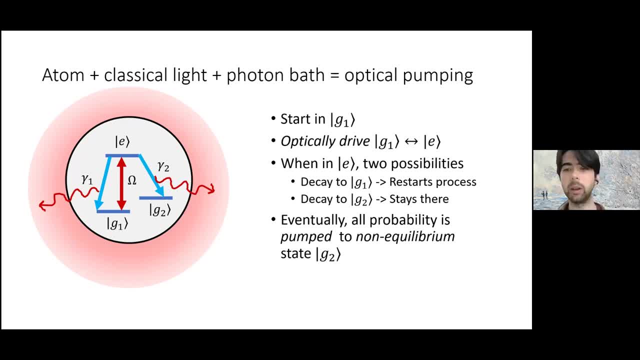 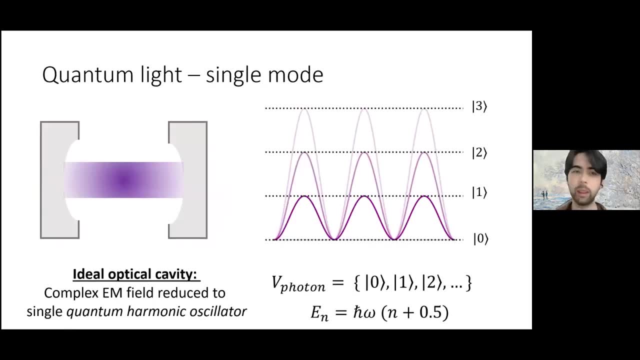 some cool ways to use optical pumping to prepare more interesting non-equilibrium states, but this is kind of the essential idea. Okay, next up is to move away from kind of ignoring everything about what the light field is and kind of reduce the complex electromagnetic field down into a very 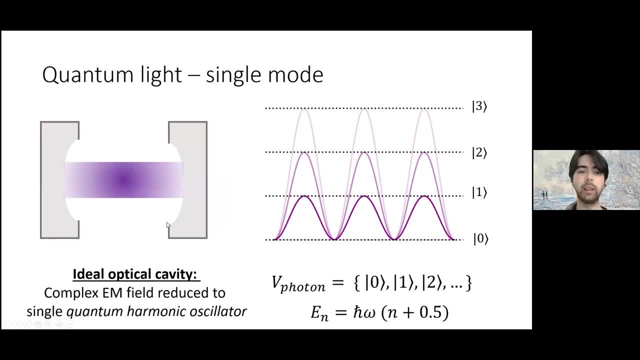 simple quantum system that we can actually understand and just reduce it into a single quantum harmonic oscillator. So the idea of this is basically that we're going that physically you would have two very highly reflective mirrors. So you would have two very highly reflective mirrors. 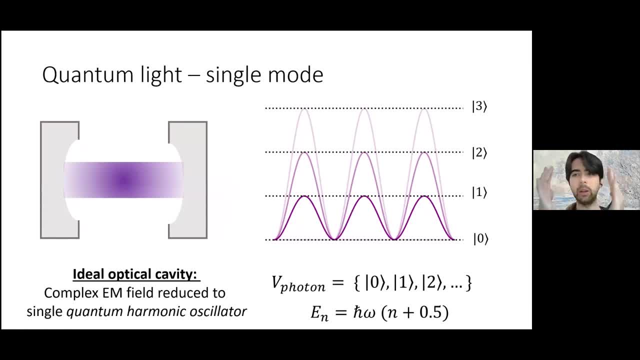 And these highly reflective mirrors will apply a boundary condition for the electric field and the result of that is that there's only a very few like isolated set of ways that it can oscillate up and down. So that's kind of illustrated here on the right. So it you can have oscillations at this. 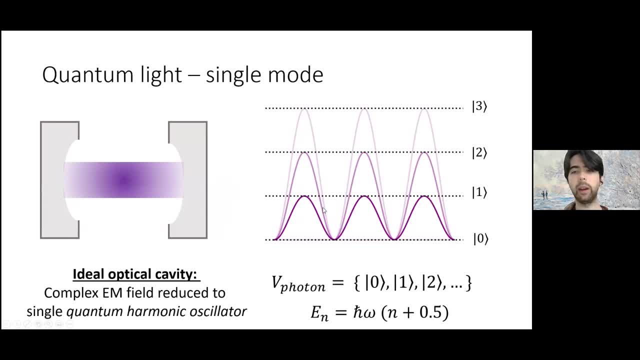 very particular pattern and you can have either one of those oscillations or two or three, So this just essentially tells you how many photons are in the cavity. This is kind of what people mean in this context when they talk about photons- is just reduce the complex electromagnetic field into a very simple single mode system, and 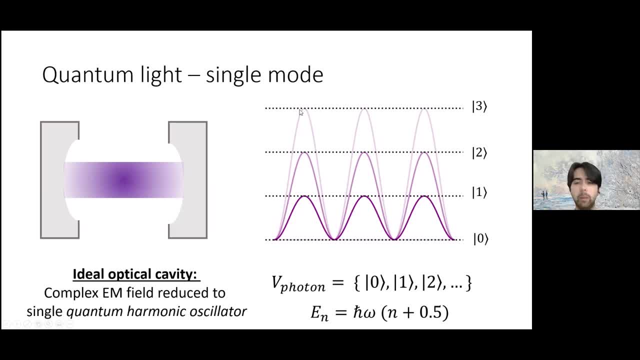 just how many photons are in that mode. So the Hilbert space of this is just some labeled by zero, one, two, all the way up to as many as you'd like, and the energies of each of these modes is just proportional to however many photons are in the 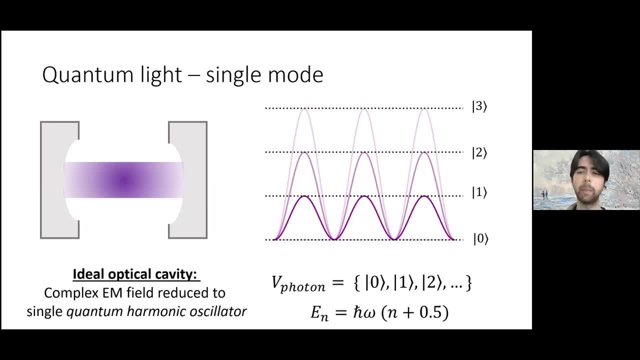 cavity. Okay, so this on its own is not too interesting. Well, there are things that are cool about this, so you can. I won't discuss this in any detail, but basically, anything that you would imagine wanting to do with a simple quantum harmonic oscillator, you can do with this photon cavity mode. 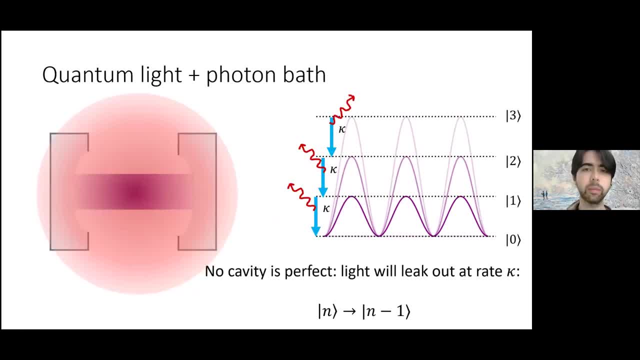 So yeah, you can look into that if you're interested, but I won't dwell on it. So what happens? so you know, I said that we've reduced the complex electromagnetic field down to the single mode, but that's not entirely true. right, it's still out there and no cavity is going to be perfect. So 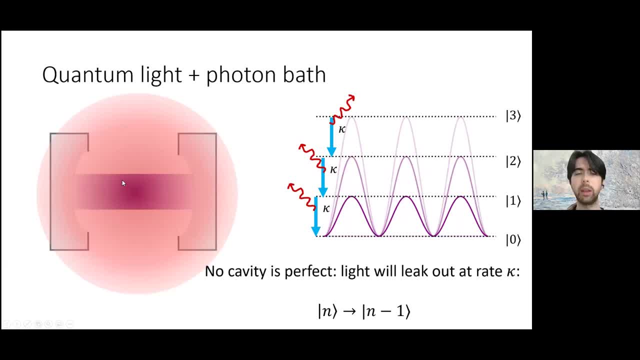 this very simple harmonic oscillator mode is also going to be coupled to the great photon bath of the universe and kind of the dominant contribution of that is going to be some leakage rate, denoted kappa, where at some frequency, if I start with my cavity mode, some state n with n photons in the cavity, one of those will just leak out. it'll. 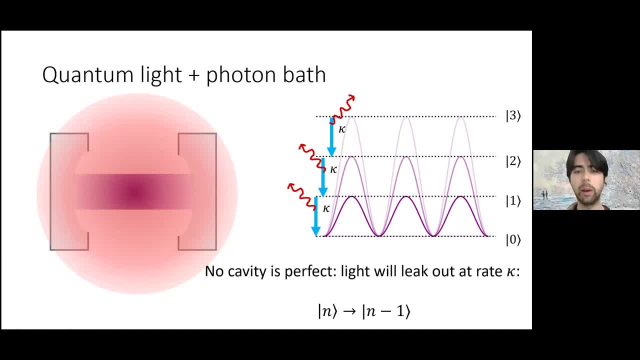 exit the cavity and go off into the great beyond and we'll lose track of that energy. Okay, so yeah, if you, it'll just kind of exponentially decay away, with some discrete photon character on top. Now we're going to do put our put in our last ingredient, which is the atom. 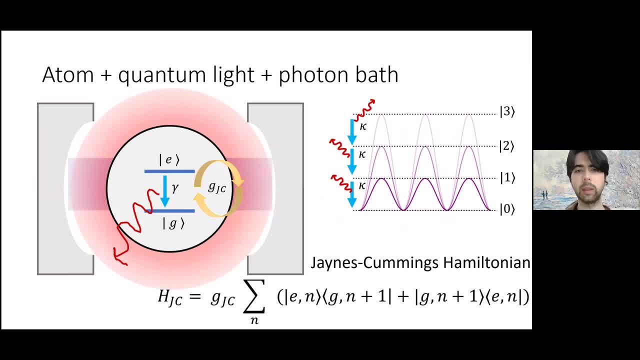 So how? so now we have of sort of three very simple things: The atom with its two internal levels, the cavity mode with its infinite tower of states, and the photon bath. So the only thing that I haven't told you about yet is how the atom and the photon mode are going to interact. 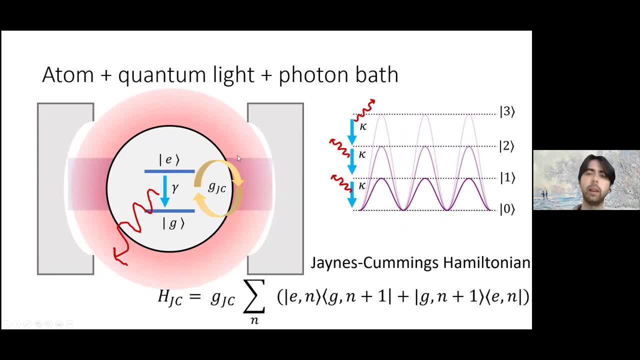 And the way that these interact is through the James Cumming Hamiltonian, where, if the cavity frequency is matches is resonant with the energy spacing between the E and the G levels, you can coherently transfer energy between the atom and between the cavity. 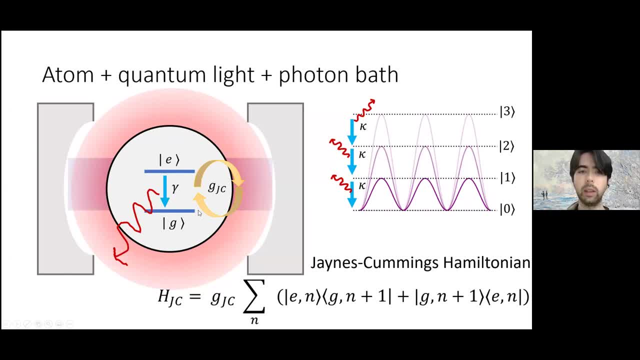 So what this looks like is kind of written down here. So if I say, start with the atom in the excited state and with N photons in the cavity, it can coherently move into have the atom being in the ground state and there'll be an additional photon in the cavity. 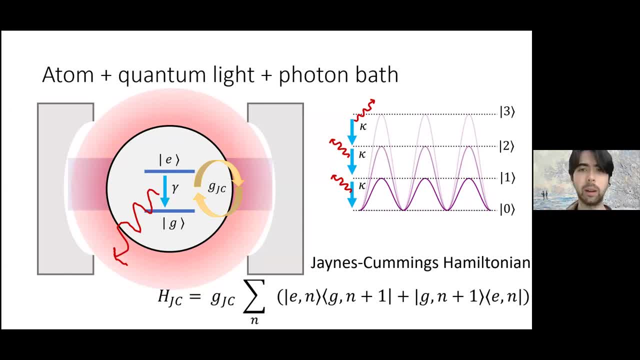 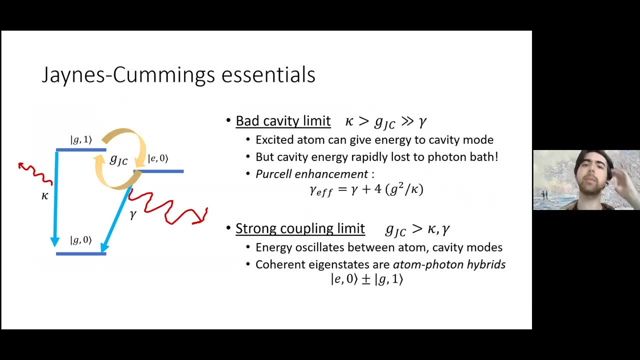 and back and forth. Okay, So this illustration is now starting to get a little overloaded, So let me just simplify it down to, I think, the very essential physics, which is this sort of three level: James Cumming, Hamiltonian, Okay, And this is basically the last thing I want to talk about. 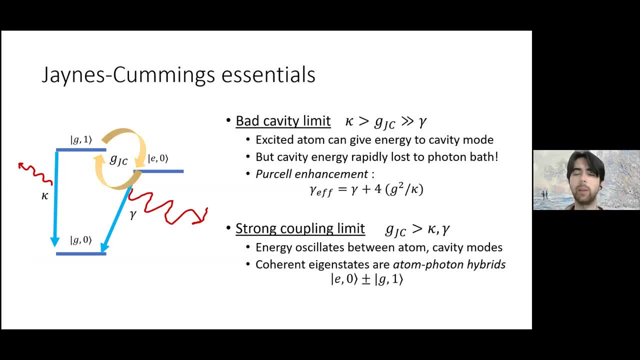 So you know I'll try and slow down here, since I think I might've gone a little too fast. So just to reiterate the most important states in the system, where I have the atom and I have the cavity mode is the lowest energy state of all. 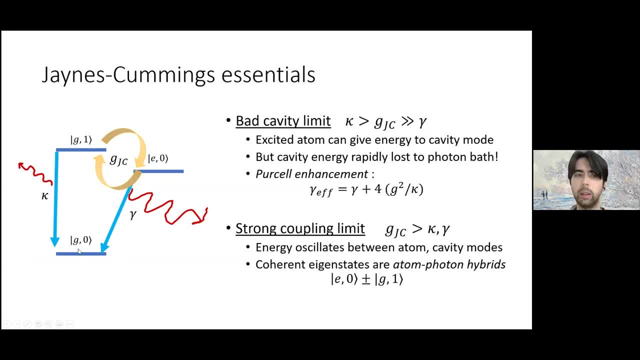 is if the atom is in the ground state and there's no photons in the cavity That's labeled by this G zero state here. Okay, Next up, there's two ways that I can add energy into the system. I can either excite the atom from the G state. 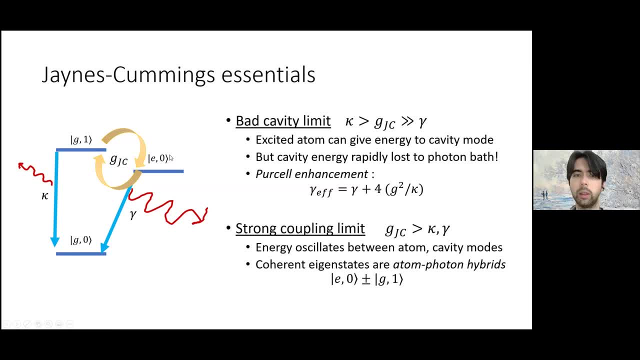 to the E state like this, but keep no photon modes in the cavity. So that's this E zero state. Alternatively, I can keep the atom in its ground state and then I can add one photon to the cavity and that's this G one state. 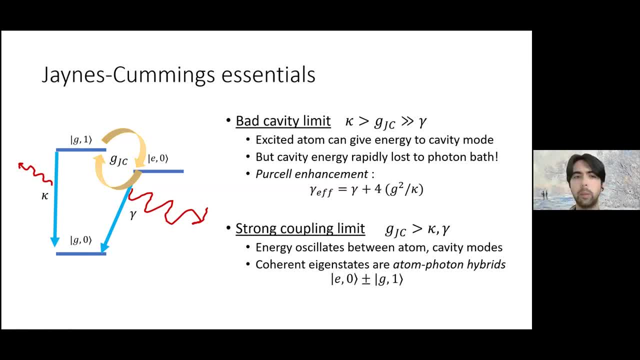 So these are the three lowest energy states of the system. Of course, on top of either of these two, I can keep adding more and more and more photons in, but you know that's like you won't gain any additional very cool physics from that. 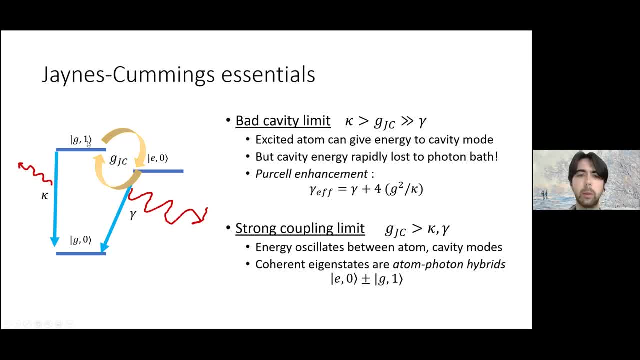 So let me just focus on these two. So and yeah, so these are the three levels. And then what is the dynamics of the system look like? So the coherent part of the dynamics is just this, James Cummings: oscillation between the atom and the ground state. 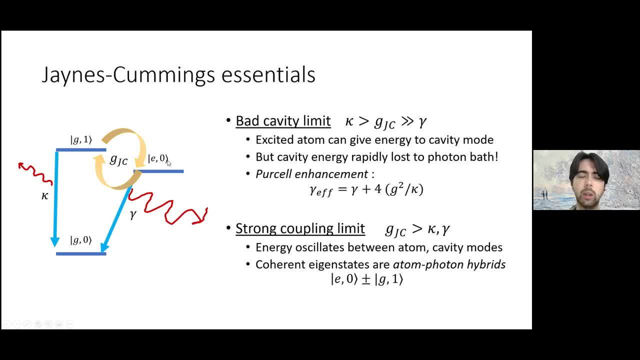 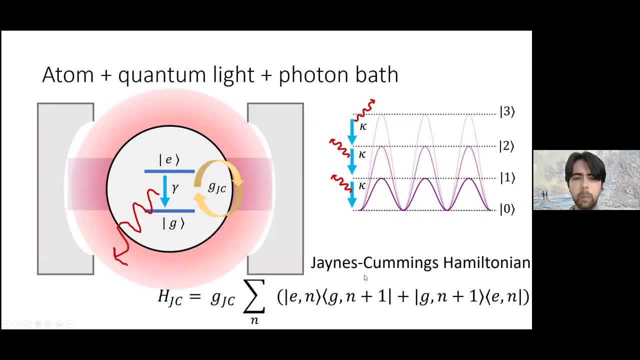 and the one in the single photon mode, and the atom and the excited state and then zero photon. So this is just some coherent term that I wrote on the previous slide. Just listening here- And then the modes, and then both of these can decay. 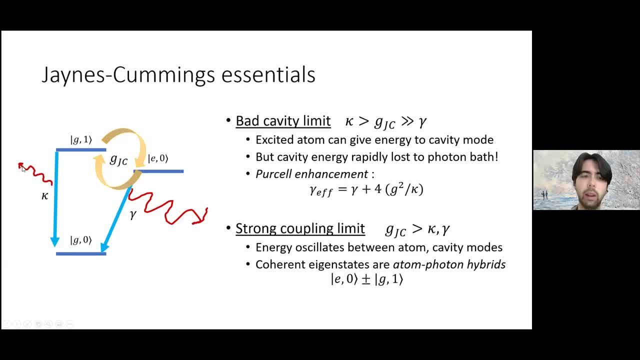 So there's G one state state: the photon can leak out of the cavity at this rate kappa, And in the atom excited state, and if there's no photons in the cavity, the atom can decay with rate gamma. So there's two, I think, interesting limits that people generally think about in this setup. 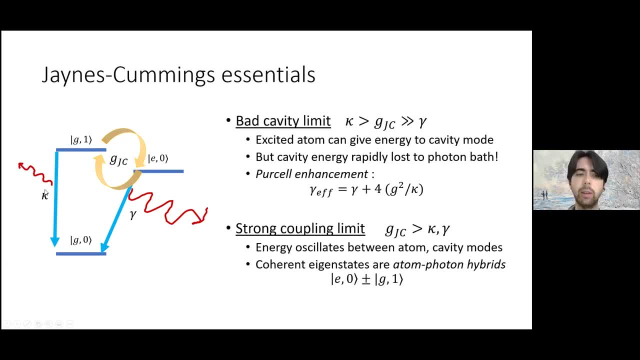 One is the so-called bad cavity limit, where the cavity is very, very leaky. Nevertheless, the atom is still coupled to the cavity mode. So the excited. if you start with an atom in this excited state, it can coherently give its energy up to the 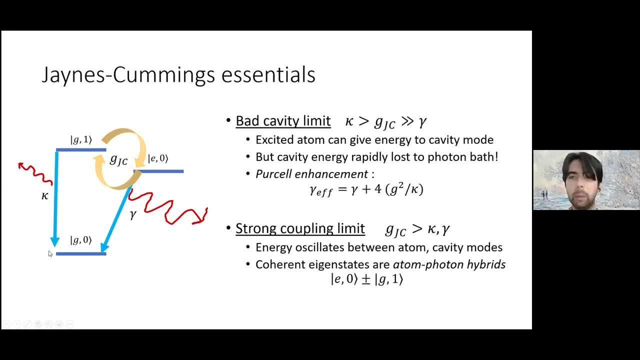 cavity and enter into this state, But then this will just rapidly decay. So this leads to what's known as the Purcell effect, where when you place an atom in a cavity, the spontaneous emission rate of the atom to decay will increase by this factor that is proportional to g squared over kappa. 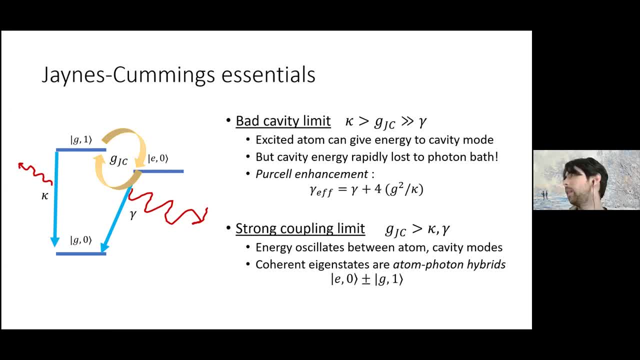 So one application of that is that if you have, say, a spin system and you want all of your spins to be in their lowest energy state, just like the isolated downstate of all the spins, if you put the spins in some kind of microwave cavity you can actually accelerate that process. 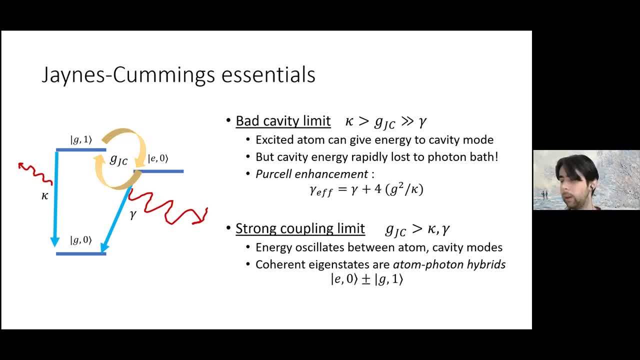 So you can more rapidly cool the spins. Additionally, in this spontaneous emission process you emit typically a single photon. So if you're trying to build a single photon source for some kind of quantum information platform, then it's possible to emit a single photon. And if you're trying to build a single photon source for some kind of quantum information platform, then it's possible to emit a single photon. 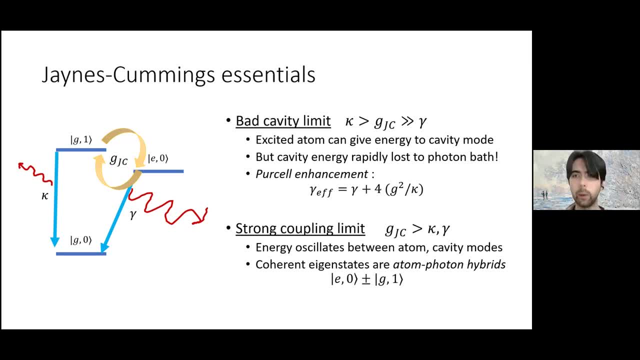 Adding a cavity can be a way to potentially enhance the rate at which you can produce these single photons. Maybe more interesting is the strong coupling limit, where this coherent term is fairly larger than either of these and it'll actually have coherent oscillations that go back and forth between these for a while. 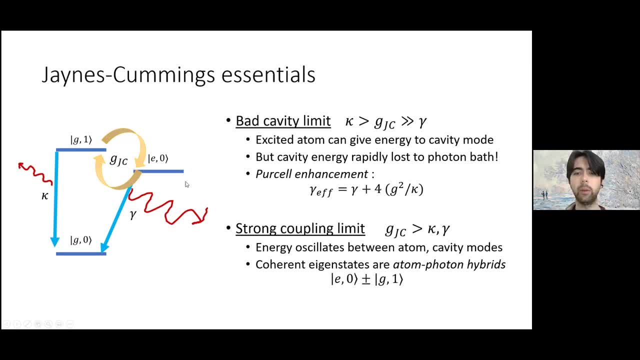 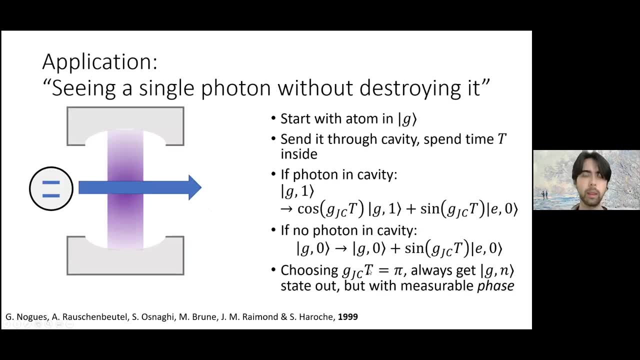 So in this case, the eigenstates of the system are atom-photon hybrids, where they'll either have the same number of atoms or they'll have identical numbers, and so they'll look like that. And finally, let me mention one application of this simple idea, which is how to see a single photon. 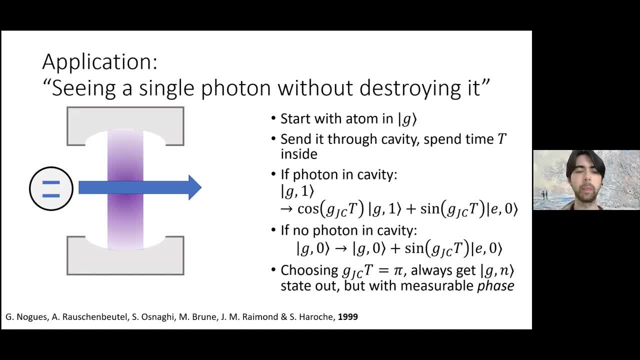 in the cavity mode without actually destroying the photon. So if you start with an atom- and this is an idea that goes back to the Hirosh group in 1999, so this is 20 years ago now- So if I start with an atom in its lower energy state, the g state, and I'll send it through the cavity, so it spends some time in a gas chamber. 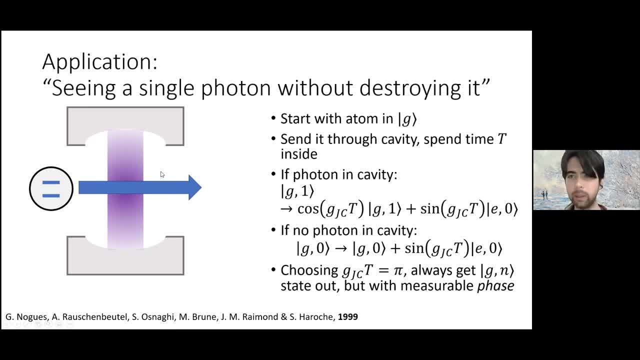 some time t in there. if the photon is in the cavity, this hybridization will lead to- i start with the ground state and one photon in the cavity, it'll lead to this final state. oh sorry, there's a typo for the no photon term. uh, this second term should not be there if there's no photon in the 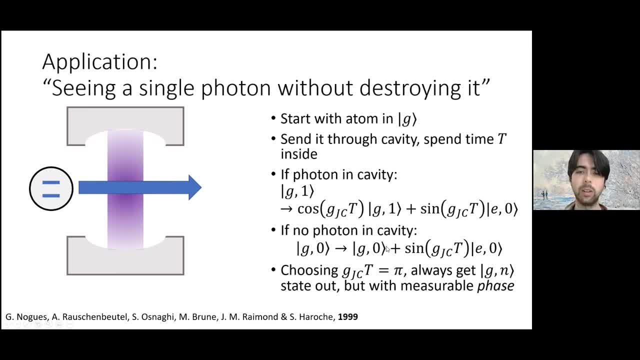 cavity, nothing happens. you just go from the g zero state to the g zero state. sorry about that. um, so if i particularly time the speed at which the atom moves through the cavity, so that this james cummings coupling times the time spent in the cavity is, uh, equal to pi, then 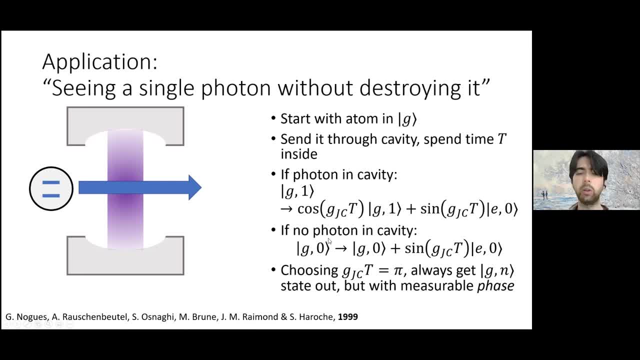 at the end i will always get g1 to g1 or d2, g0 to g0, but the g1 term will pick up a minus one phase and that's measurable. so by doing some interferometry on the the phase of the atom wave function, at the end you can actually measure how many photons are in the cavity. 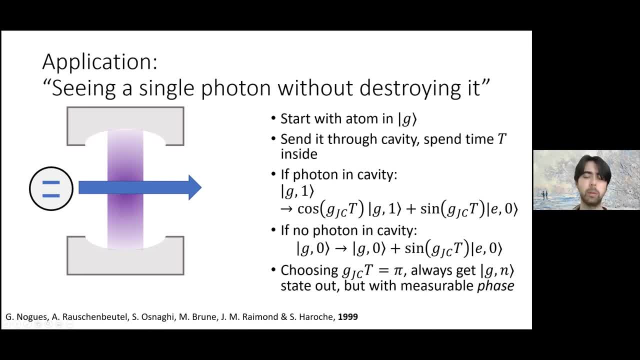 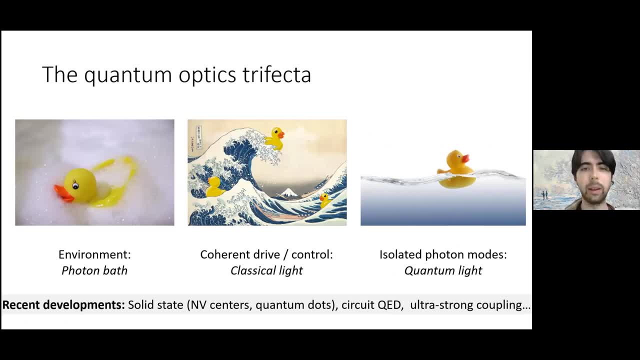 without actually affecting how many photons are in the cavity, which is pretty cool. okay, so i think that that's uh the end of my introduction. pretty much so. um, going back to this, there's, in this realm of quantum optics, sort of three ways that you can imagine, uh, interfacing light. 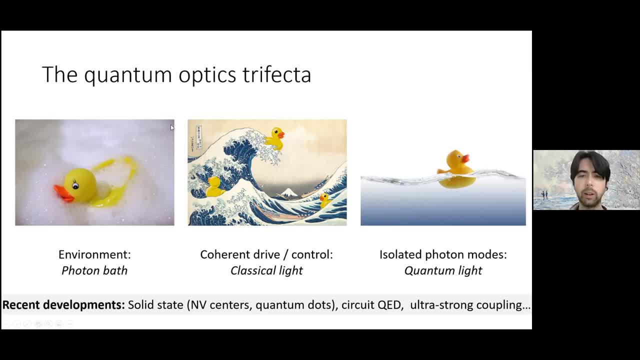 with your system. one is through the systems coupling to the general photon path, which leads to some leakage of energy or preparation of non-equilibrium states. the other is, yeah, by this classical drive. and then the last is by isolating a single special photon mode and using this quantum. 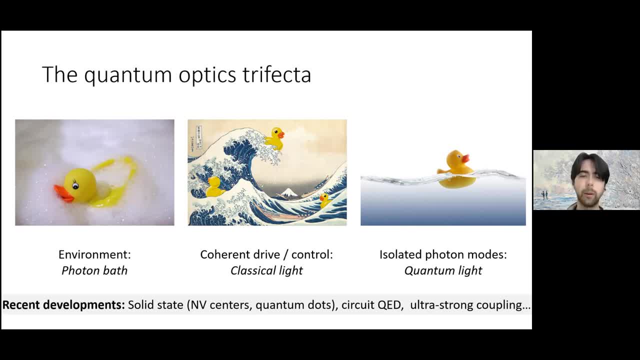 light. um, i should say that you know. of course people have continued to pursue this field since this 1999 experiment i mentioned in some interesting recent developments along these lines are replacing your atom with a solid state system, like a quantum docked or a nitrogen vacancy. 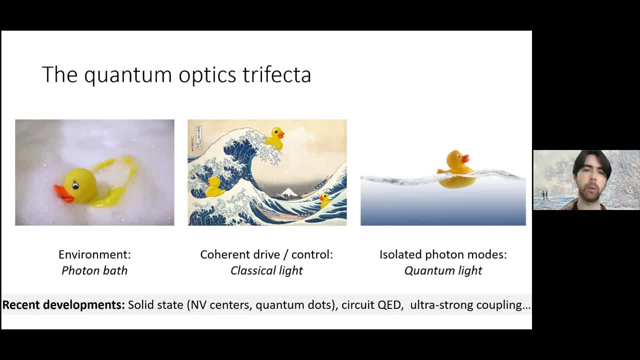 center in diamond. the whole uh field of circuit, quantum electrodynamics, is sort of very closely related to this picture. where the atom is is now a, a, a transmon, an artificial system, and instead of having the actual mirror cavity system it's more like a radio line. but 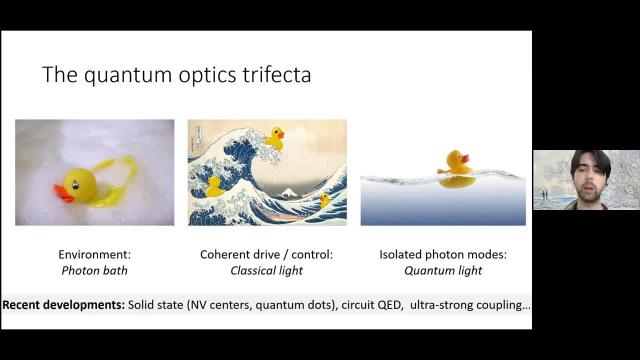 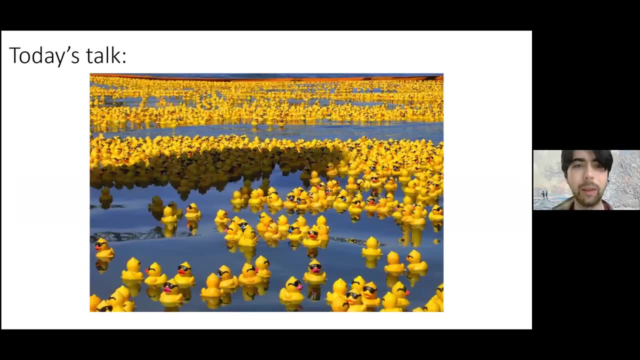 it's still the same sort of spin plus harmonic oscillator picture and, of course, yeah. so i think that's all to say and let's bring it now into uh today's talk. so muhammad will be telling us uh about what happens when you add quantum light to uh the mini body system. yeah, thank you, marcus. so 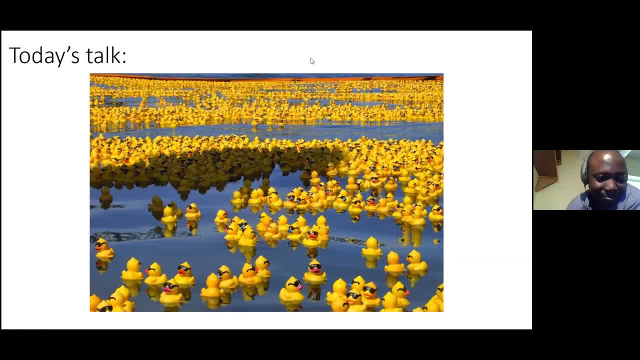 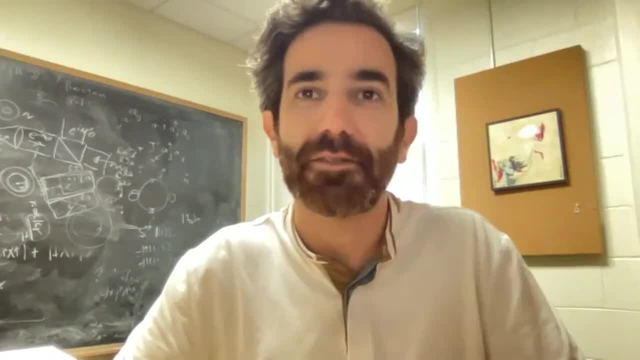 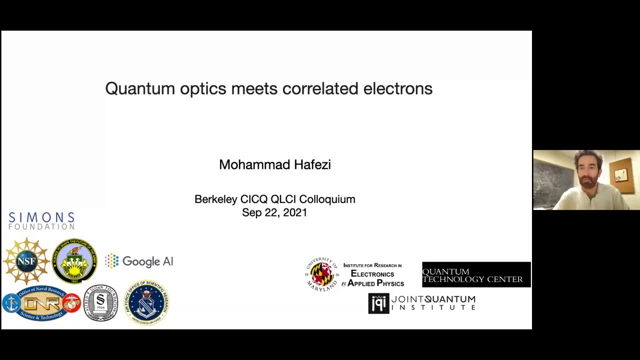 muhammad, take it away. thank you for the introduction, thanks for the invitation and especially thanks, marcus, for a very nice intro to the field. can you see my slide, the right one? yes, you can, okay, um so, uh, let's uh, now that we learned all the preliminary and basic. 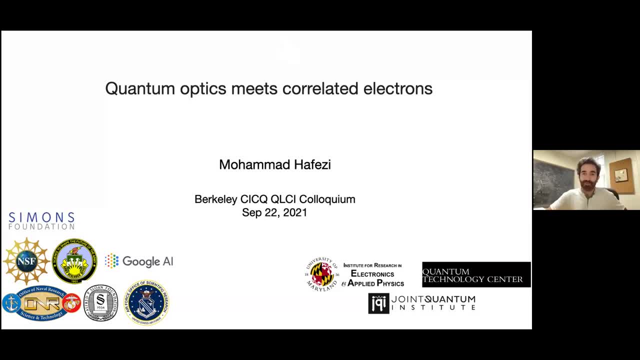 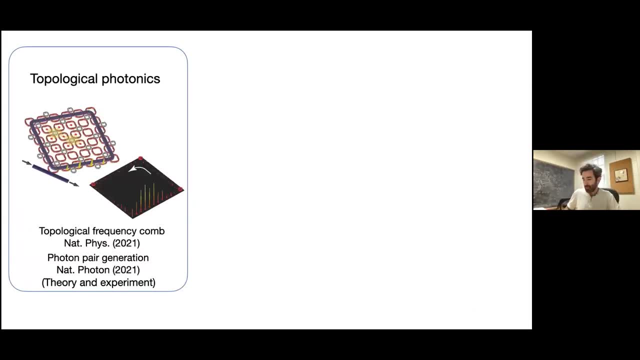 things that we need for this talk. let's jump to our talk. so, um, this doesn't work, so i just want to also, before uh, jumping into the specific talk, introduce what we are doing in my research group. there are basically three main topics that we are working on. one is topological. 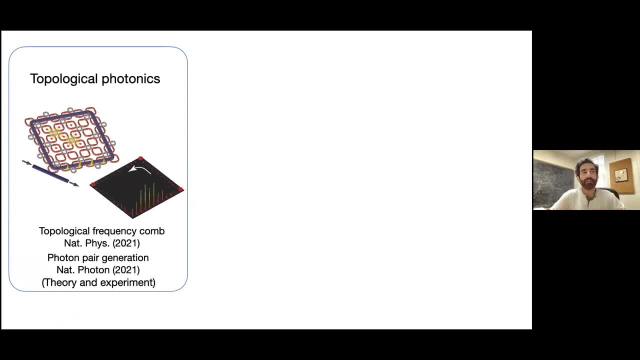 photonics. the idea is how to explore interesting topological effects in uh photonic systems and more recently we have realized that we can actually use these robust systems to make maybe useful uh structures, uh like frequency comb and photon pair generation on chip. pubocar is an expert in this topic, so i hope he will bring also some other speakers to talk about. 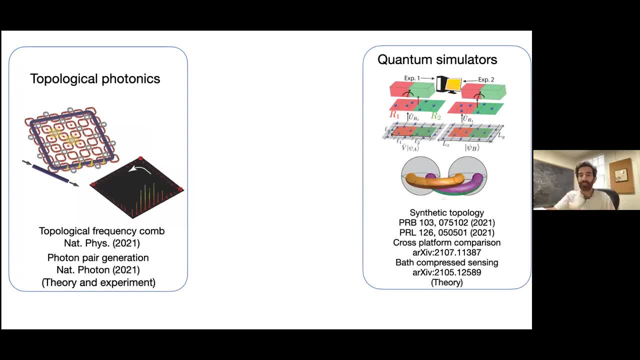 that. and there is another topic which is actually very related to uh, qlci, uh that you have, uh, which is the idea of quantum energy temperature, how to apply quantum energy to quantum energy levels, brains from quantum memory and nonlinear fraternal spans with amo simulators, how we can efficiently measure the system, how we can efficiently implement. 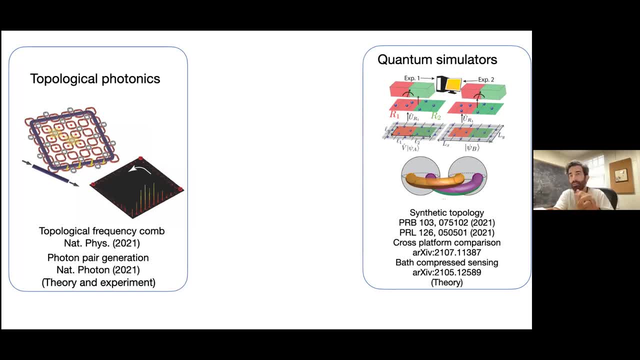 certain Hamiltonians and interesting models, et cetera. In particular, we had some results on how to engineer synthetic topologies. after the system is done, basically in post-processing, I give you a wave function, for example on a disk. Can I post-process it in such a way that? 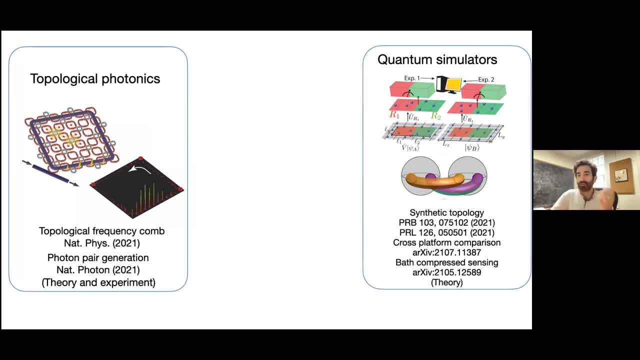 as if the wave function was living on a torus or with something that has a handle. And can we use this to measure many-body properties like fractional channel number, et cetera, where we don't have access to put the system on a torus or to put the system on a cylinder? Most of 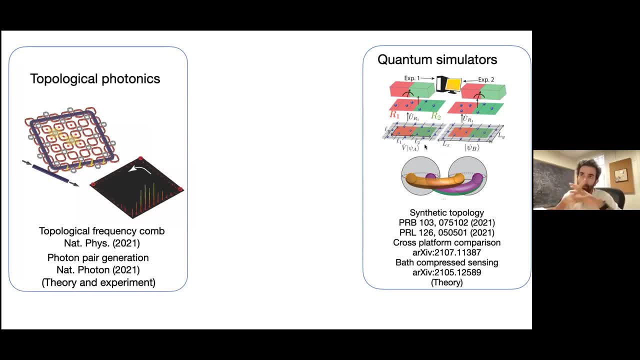 the platforms- as you know, they work on a flat surface- And then how we can measure the bath efficiency, et cetera. So if you're interested in these topics, please ask questions later after the talk and we can chat about it. The subject of this talk is 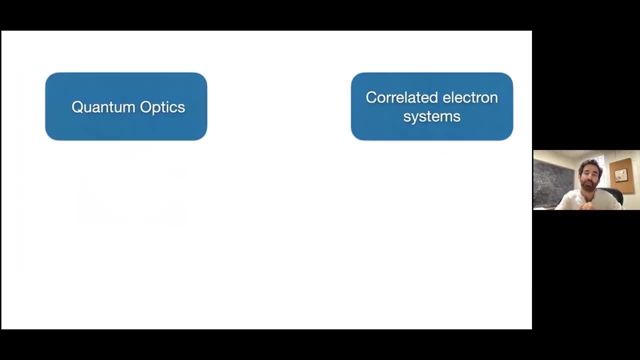 quantum optics of correlated electrons And, thanks to Marcus, now we know what are some of the tools in the toolbox of quantum optics. So the whole idea is that can we use this quantum optical toolbox on correlated electronic systems? The opposite of this has to do with the fact that 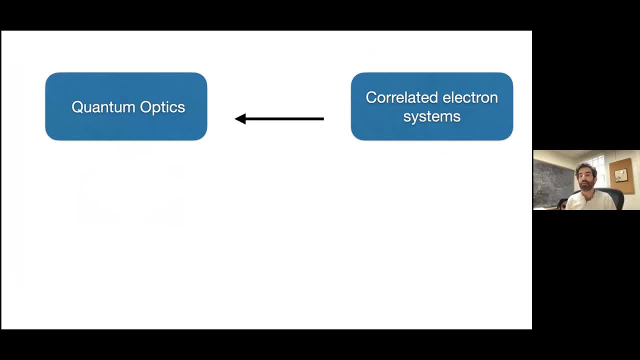 as you know, quantum optics has been going on for a long time, in particular in the context of cold-atom systems, that we had these interesting Hamiltonian models like Bose-Hubbard model, vortex states, fractional quantum Hall states, et cetera. how we can implement it in an AMO system. 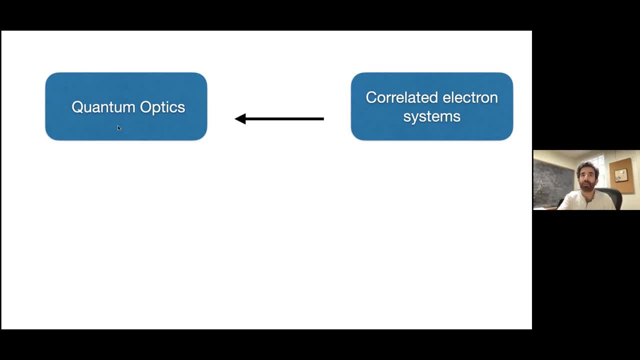 using quantum optical toolbox. Now this is the other way around, that we want to use quantum optical toolbox on correlated electronic system And, in particular, can we use these techniques, both theoretically and mathematically, to measure the path efficiency of quantum optical systems? 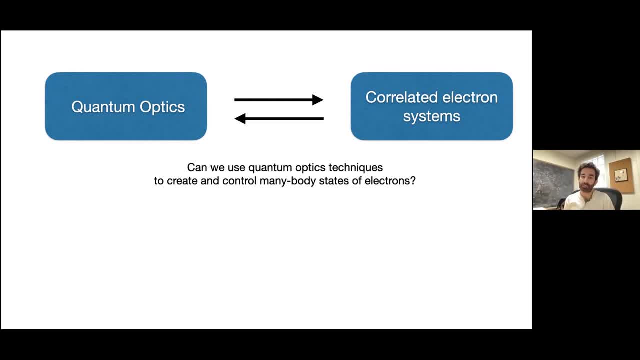 So to me, we have to look at the actual working environment of quantum optical systems. So, as a result, you can get a lot of really very interesting results here. So to me- this is the other thing that I would like to think about- This- is one of the things that the students on the class are going to see us doing, which is looking at what are we able to do to control quantum optical systems. Can we use quantum optical instincts? So the first point that I would like to, as a matter of fact, explain is: you know, quantum optical systems. 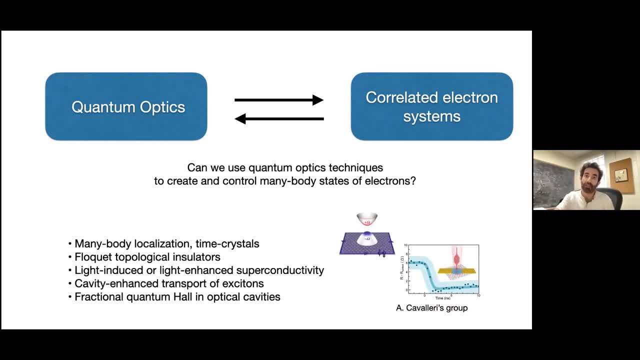 uh, correlated the state of electrons, and this is already an ongoing work. it's not that we just came up with this idea last night. there are many works that can fit in this category, for example, uh, the works that norman company has been doing on many body localization time. crystal is actually an. 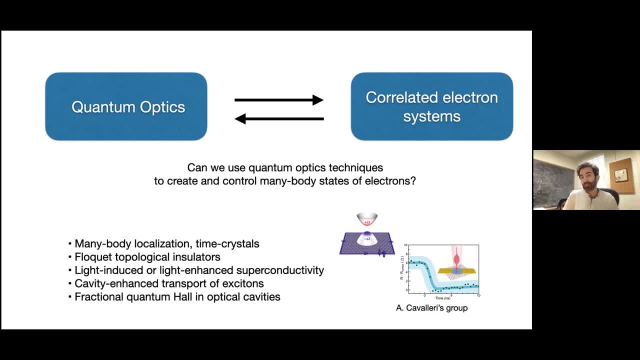 example of this flow ketopological insulator that i start with an inset system that is not insulating. i shine light and then couple some of the levels and then turn it into a topological insulator. the more recent experiments on light induced or light enhanced superconductivity. 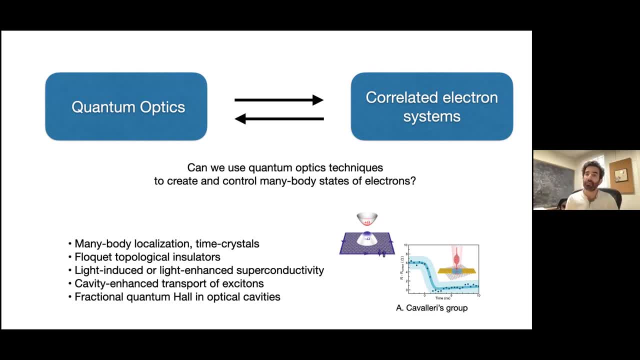 and these are some uh, some figures from uh andrea cavalieri's group, where uh you shine light and uh you are. it seems that we are actually inducing superconductivity with just light cavity enhanced transport. if you have bunch of, if you have some complicated molecule, you don't have any transport, or your. 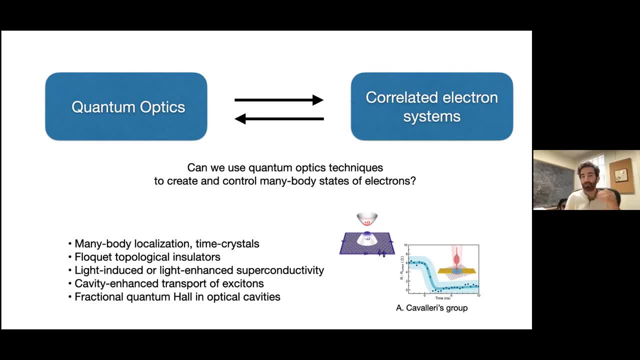 transport is very limited. but now you put it, you put the cavity around it. can we enhance the transport? and there was some recent experiment in thomas thomas everson's lab- and fractional quantum hall state in optical cavity, instead of putting the two level system that marcus was talking about. 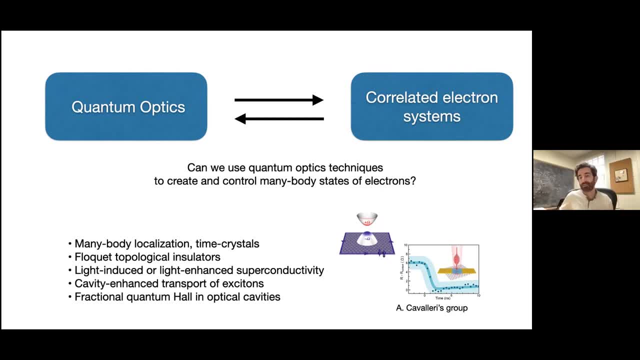 now, if you put a fractional quantum state, a correlated state of electrons, in a cavity, what can we do with it and what can we learn from it? so now, going uh from correlated electrons to atomic uh, to amo was with atomic precision. we could implement both howard model with atomic precision going this way. 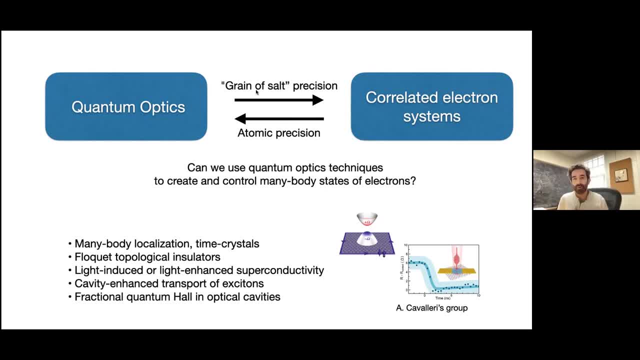 it's basically grain of salt precision, because you have now to deal with a correlated uh matter. you have to deal with the real electronic system, with disorder, with a, with a complicated band structure, etc. etc. so these stories are going to be way more complicated and experiment and theories. 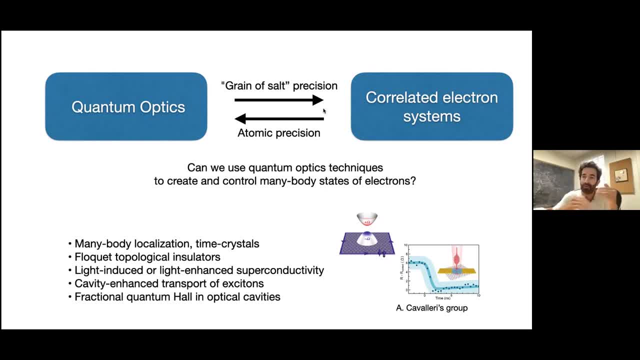 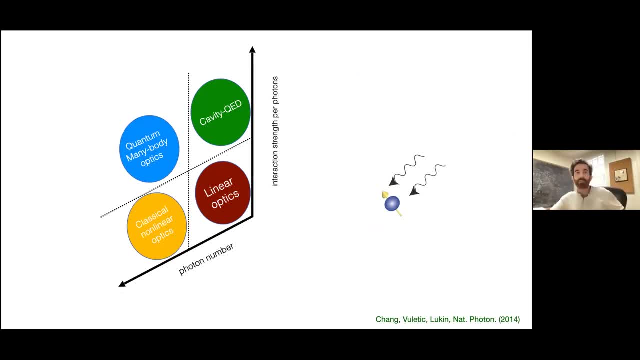 should really come from one side to the other and then maybe, hopefully, at some point they meet each other. so, since this is a colloquium, i want to give like a broad spect, uh, the broad view of where this uh fits in the, uh, in the quantum optics language. and, thanks to marcus, 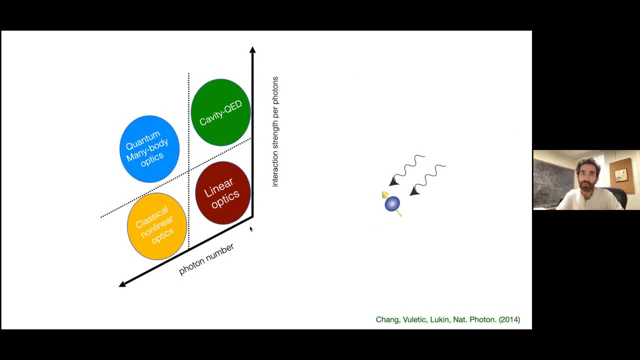 we're already halfway through that. so, um, i was inspired actually by this review that uh, derek chang, uh uh, misha, lukin and vlad and volodya wrote a while ago on on how to see quantum optics in different regimes. one axis is photon number, the other axis is interaction strength. 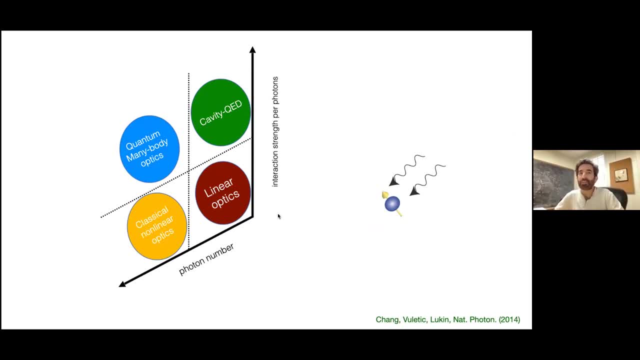 per photons. so, uh, this in the free space would be basically, uh, fine structure factor, how strongly light can interact with it with the two level system. so if you, if you're in free space and you have a small number of photons, then you're in the linear optics regime, if you, if you. 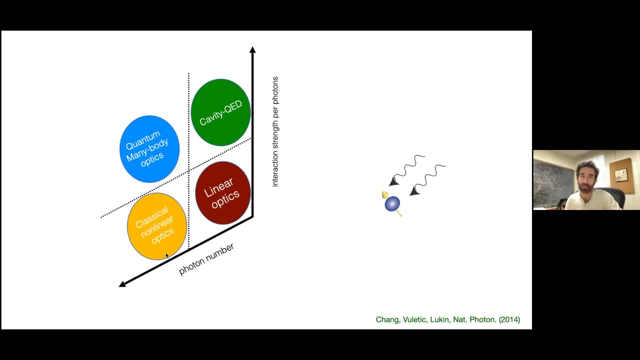 increase the number of photons while keeping the strength of interaction small. then you go to classical nonlinear optics like solitons, things like that. now, if you put the photon in a cavity such that this photon can talk to the atom many times before it leaves the cavity, then you increase. 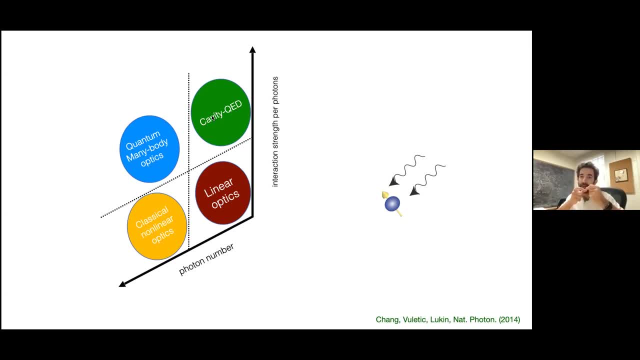 that probability of interacting with a single atom by the number of round trips. people usually call it finesse and you go to the regime of cavity qed that we just heard about now. if you put many photons in that system, then we can talk about many photons that are strongly interacting with. 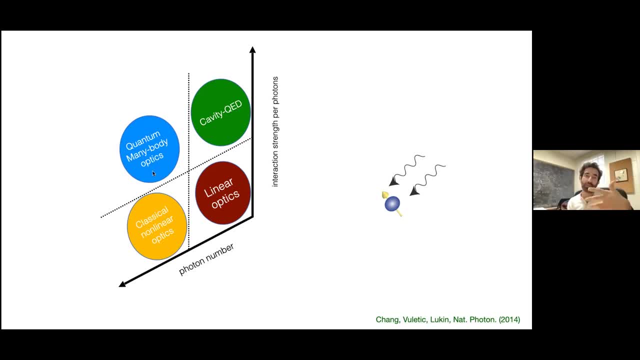 each other, and the most recent example was, uh creation of a mod insulator of photons, uh in in chicago. so the way that to do it is that you put the atom in the cavity and and the only shape that i could find was a duck. uh, in my keynote- and i think marcus was- was inspired by this for the 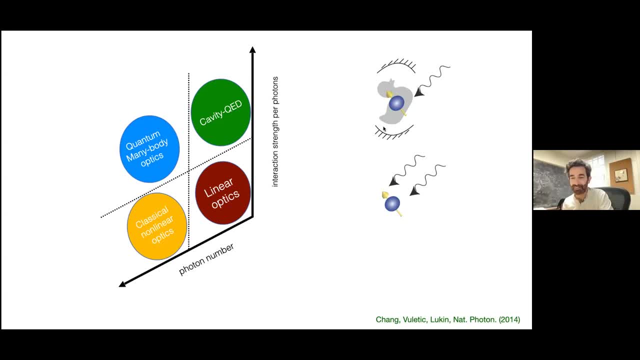 other way around, that he used the duck uh as the as the preferred uh way of uh showing uh, an arbitrary mode of light. so now the idea here is that we have yet another axis that might have been overlooked, and that's the correlation between electrons. so if the uh electrons are local, say uh, it's in a quantum dot or a or a nv centers or any color. 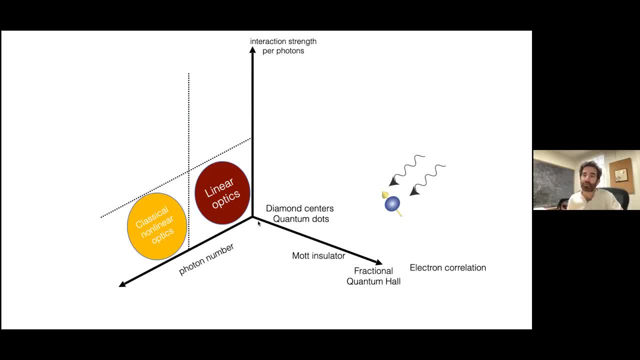 centers in diamond, then the electronic correlation length or uh are local, uh and and weak. there is no uh correlation, it's just a two-level uh system like a hydrogen atom. but then when we can go to the regime that electrons are strongly correlated, strongly interacting with each other, 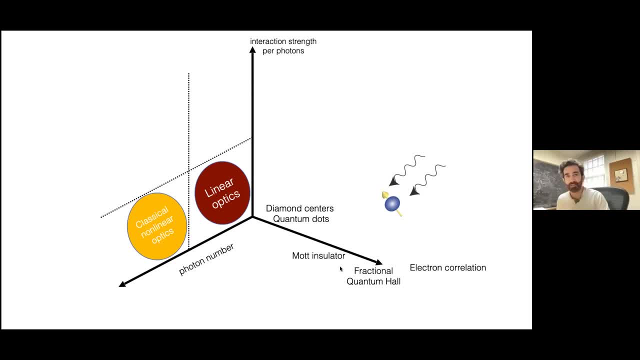 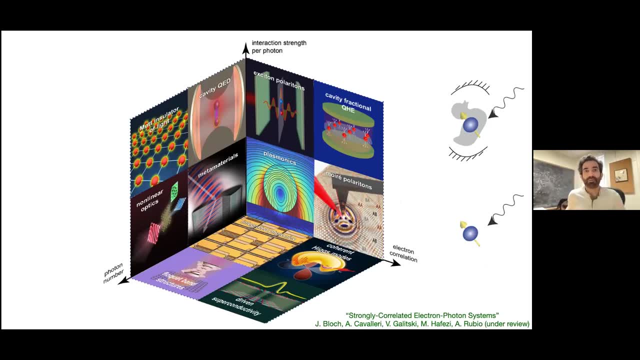 you can have martin insulators, fractional quantum, hollow states of electrons, etc. what happens when light interact with these material and then, and then we can tile uh, this three-dimensional system, by different examples. of course it's it's hard to show different examples in 3d uh. so in this perspective that hopefully will come out soon, 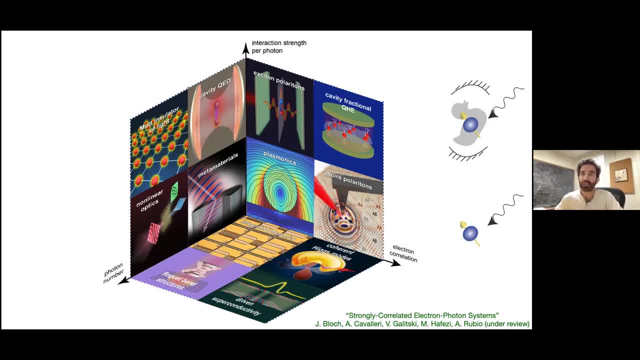 we, we try to uh, look at different regimes. for example, if i have a classical light and no correlation or weak coloration correlation in the system- let's say graphene and i shine strong light- then i get to look at topology layer insulator. so this is one way of classically 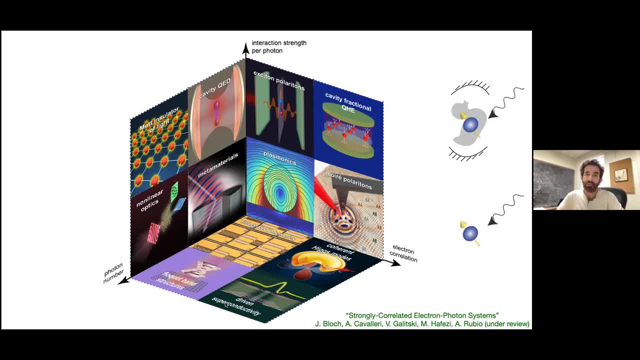 changing the hamiltonian of the system. now if we go to a correlated system, then we can think of uh changing the super conducting uh behavior in the system. so again, the number of photons is large, the correlation is now large and we are in this region or we can go to another regime that we have. 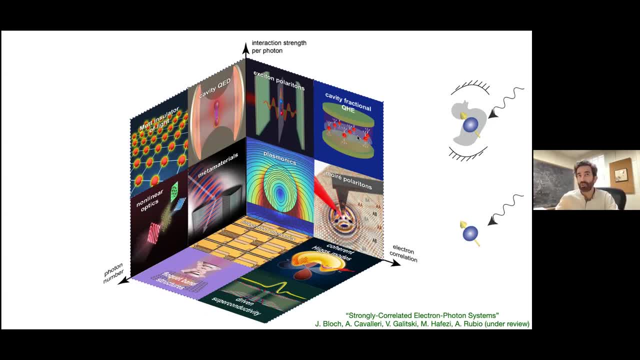 correlated electronic states. they are strongly interacting with each other and like a fraction of quantum holostate and then put them in a cavity and study them. if they are weakly interacting with each other, then that would be the story of exciton polarity in in gallium arsenide system. so this this: 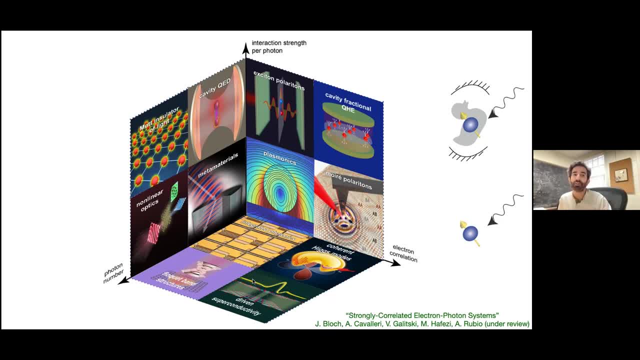 these kind of regimes are are the interest of, is of our interest in. so basically using light to manipulate, uh the band structure or the interaction of the system, and also look at using these cavity qed tools, uh to manipulate and control the state of the system. so, with this very broad overview, i 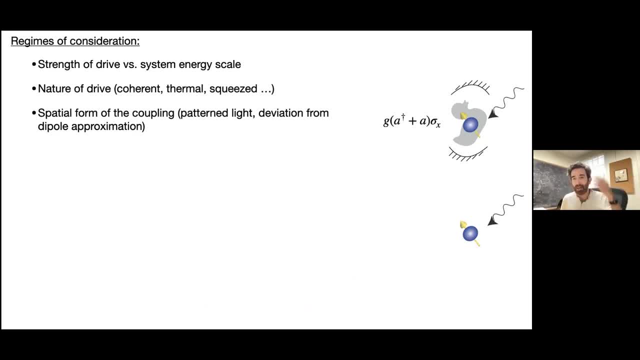 would like to kind of give a give an outlook here and then we'll come back to this outlook again. what kind of questions we are answering over here. so the regimes of considerations are the following: is that how strong the drive should be, should be, should it be a vacuum or a classical states, etc. 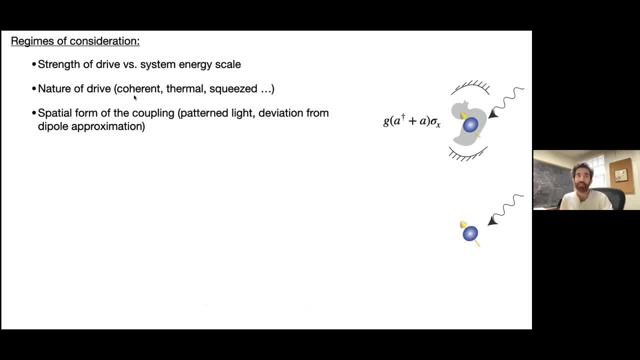 compared to the energy of the system. what's the form of the drive? as a coherent state, thermal state or squeezes states, would it matter? can we actually use the uh statistical statistics of light to achieve, uh, what we're looking for? can we, for example, induce some pair? 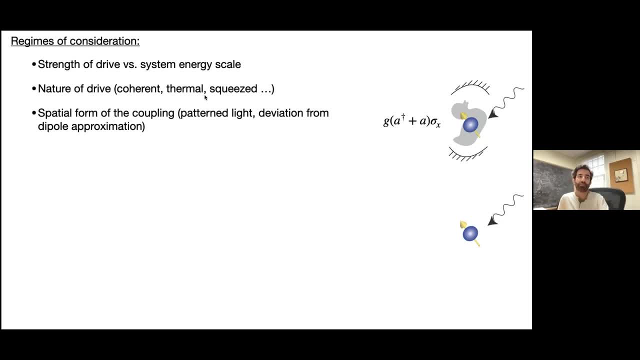 uh using a pairing of photons within squeezed photons, a special form of the coupling uh. we can actually shine light in many patterns, as we've learned, in particular in cold atom and rydberg arrays. can we use them for uh electronic systems as well? in many of the situations here we are? 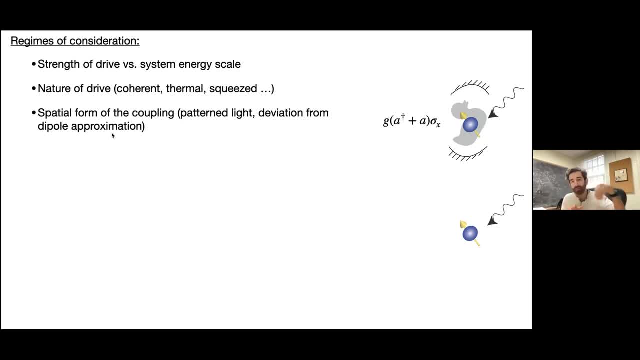 dealing with itinerant electrons, that the electron can actually move around the system rather than being localized in in, uh, in color centers. so then, uh, can we use a dipole approximation, and whether just some of the basic things that we know in quantum optics apply or not. so one of the questions, that again, what the 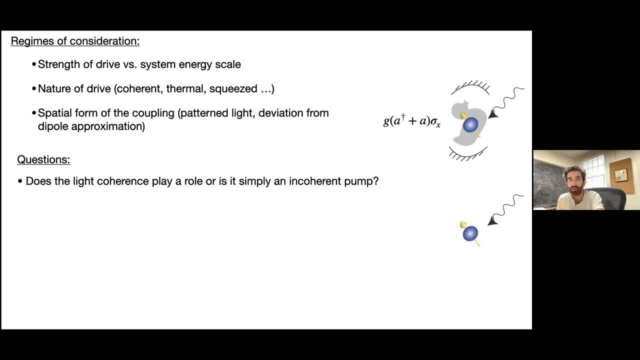 light coherent play a role or simply a incoherent pump is enough. breakdown of two level uh uh, two level atom picture. what is a strong uh light matter coupling limit? uh, we heard in the pre-talk that there is a very nice uh model, this called james cummings model, and it kind of captures most of the uh quantum optics. 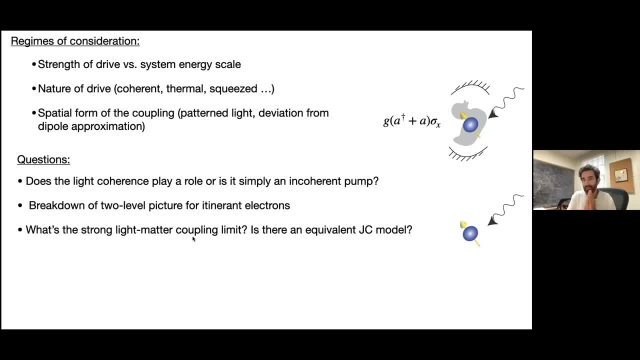 that we know we have a two level system and a cavity, and then this is actually very nice. it captures many of the physics. we unfortunately don't yet have such a thing for correlated electrons in particular, because they are moving around. what's, what do we mean by strong light? 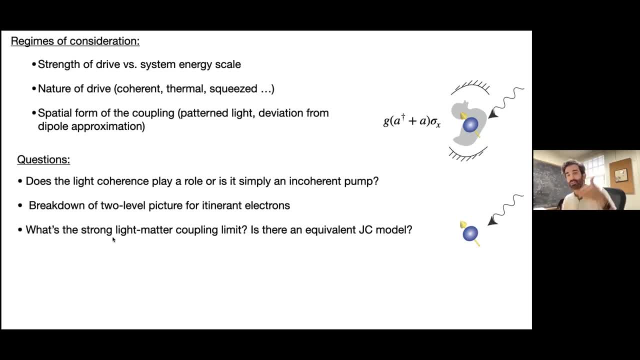 matter coupling. it was mentioned ultra strong coupling in the pre-talk. sometimes, actually, this ultra strong coupling- uh regime is clustered between the two levels of the system and the pre-talks, and so that's going to be the thing that we will talk about in the next talk. 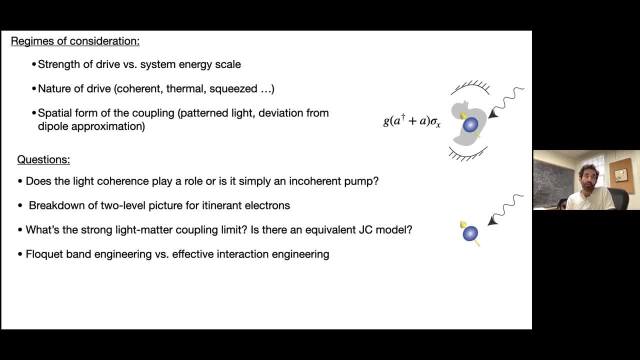 so were we. are we going to talk about the classical flow k band engineering? actually we're doing the real class blake and i want to point out that this is not a classical. we can talk about it in an almost not classical way. it's not classical and i don't get to it into. 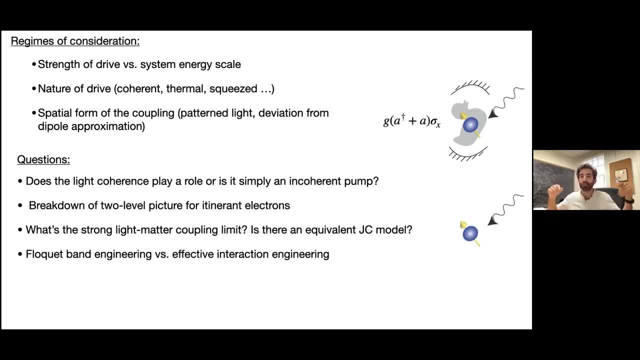 the talk, but then we can talk about it, why sometimes it's actually classical two-level systems that are in the momentum space. So basically, I start with some band structure in the brilliant zone, I couple light and I can change the band structure. Also, we can use this. 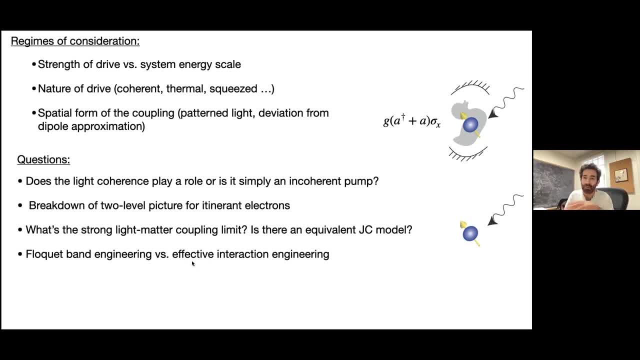 light coupling to change the effective interaction in the system. We always have Coulomb interaction in an electronic system. Can I use light to actually pick up specific part of the Coulomb interaction and tailor the form or strength of my Coulomb interaction? How does the drive compete with the formation of excellence? This is a little bit technical. 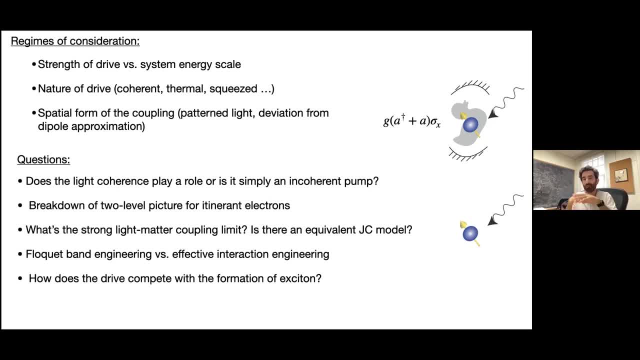 Most of the theories that has been developed. they are for free electron or correlated electron system And they do not really take into account that once we shine light, we actually the first thing that we create might be an exciton, Like in a semiconductor, for example. 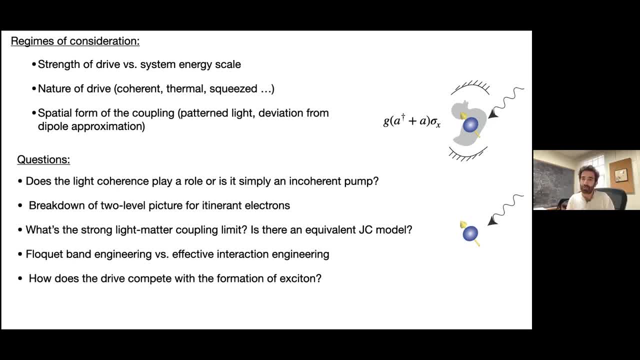 if you use just a free carrier picture, then you get everything wrong. You don't get the absorption lines, et cetera. You have to consider the Coulomb interaction and in particular, the formation of excitons. One kind of very important consideration is the situation of heating and disorder Once we shine light on a system. 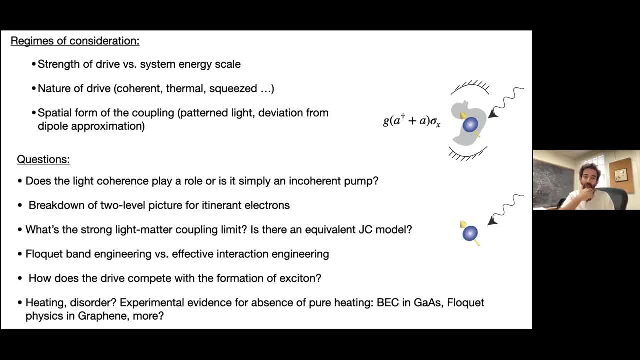 we may just heat it and do not see anything, But fortunately some recent experiments have shown us that this is actually possible. We can have a coherent light-matter interaction in a material like BEC in gallium arsenide or flow K physics in graphene. That shining light does not lead to heating and we can have some coherent 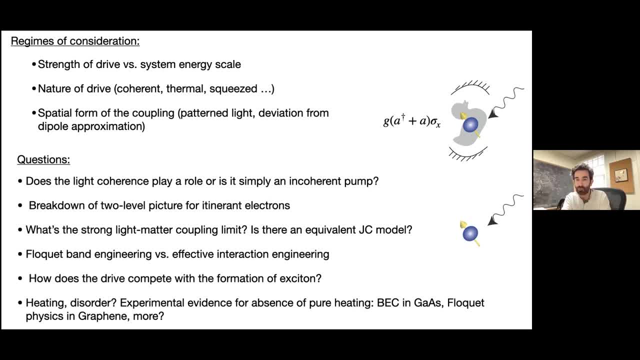 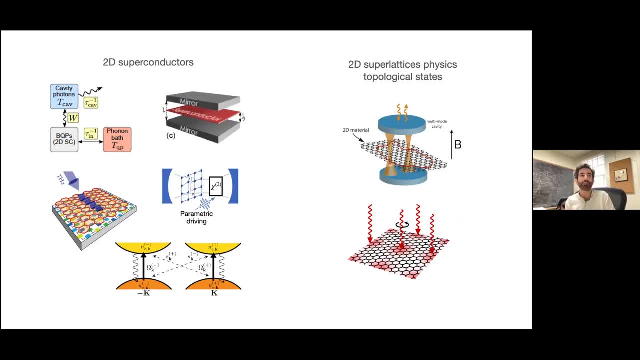 physics. So these are kind of the questions that I would like to talk about in the talk. The specific problems are in two categories. The first category is superconductors: How we can use some of these techniques like cavity QED, Optical pumping, squeezed light and selective coupling to play with the properties of the. 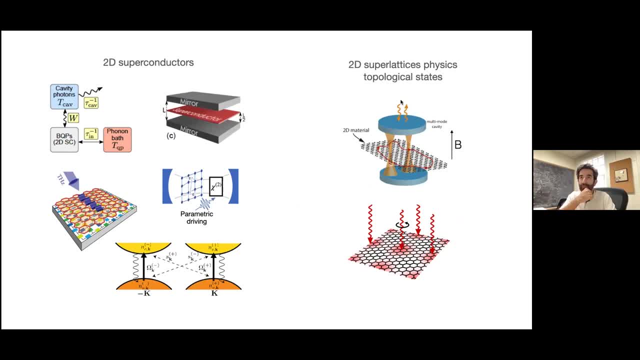 semiconductor, maybe enhance them or maybe induce them. And then second part is more how we can use patterned light or cavities to change and study some of the topological properties of the electronic states. So I don't know what the exact format is. Please jump in and ask questions as they. 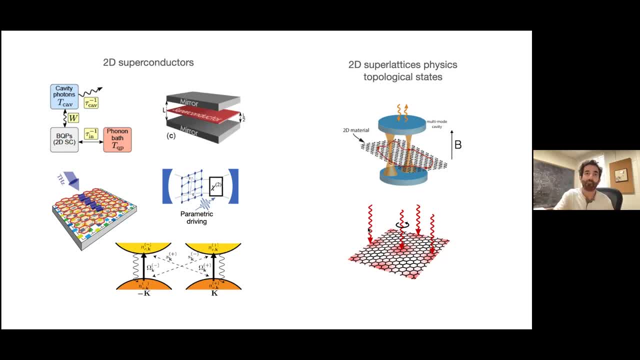 come in. Sounds good, Yeah, and if you would prefer to have your question asked anonymously, you can feel free to pass along to me in the chat and I will send it along to Mohammed, So that's also an option. Or if you prefer to just put it in the chat in public, I will also call it out and read it as: 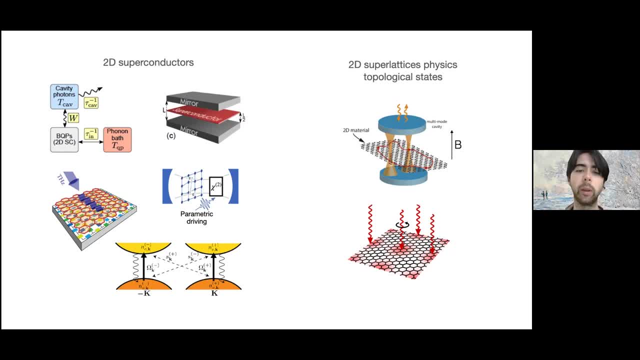 soon as I can. So yeah, feel free to ask questions in the chat, either publicly or privately. Yes, I would really appreciate it, because then I know how fast or how slow I'm going. So let's start with the first example of a superconductor in a cavity. 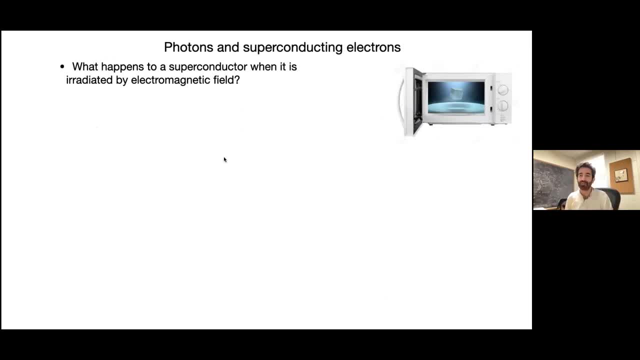 Okay, so you put the cavity in a microwave oven And what's going to happen to it? So it's going to kill the superconductivity, and this is not an experiment. It's not going to kill it. The naive guess is thatokayit's going to kill the superconductivity. 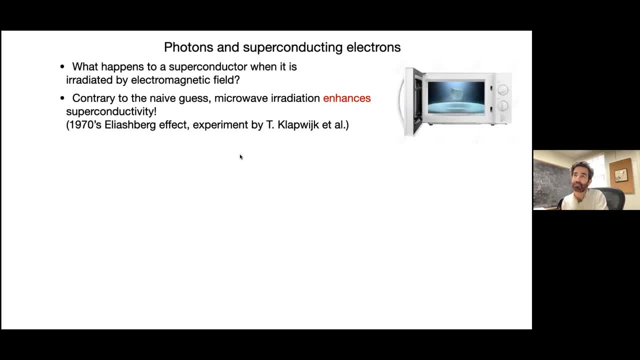 but it turned out that it's not the case. And then there's a theory and experiment from a long time ago that actually this is not always the case. We can actually enhance superconductivity by shining light, and the very simple picture to understanding this is the following: 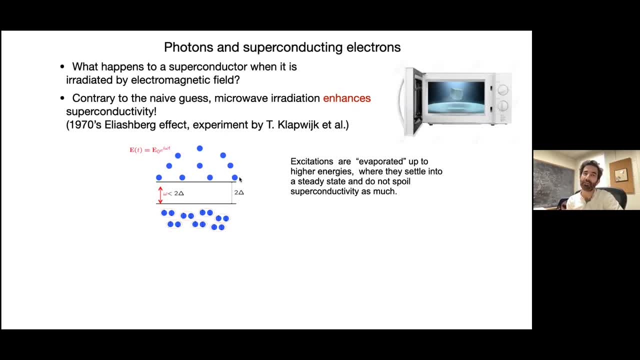 pairs and then you have the superconducting gap and then you have the Bougolev of quasi-particles on top. If you shine some light with some frequency- in this case with the microwave- less than this gap, then you cannot break any Cooper pair because you don't have the required. 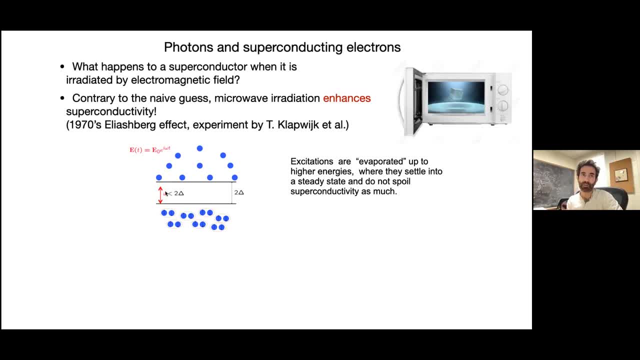 energy. Each photon does not have the required energy to break this Cooper pair. So instead, you're not going to touch these guys, Instead you're going to excite these Bougolev of quasi-particles that are close to the gap and then promote them, or kind of evaporate them, to higher energies. 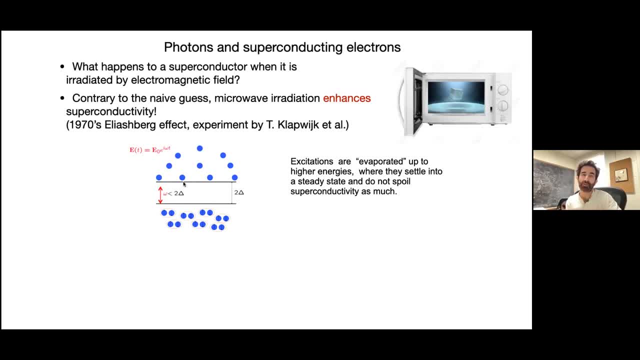 And the way that the BCS theory and the gap equation works is that you really care about these guys that are close to the gap. So if you put them away, then you effectively increase your gap by getting rid of them and then putting them at higher energy and hopefully they get. 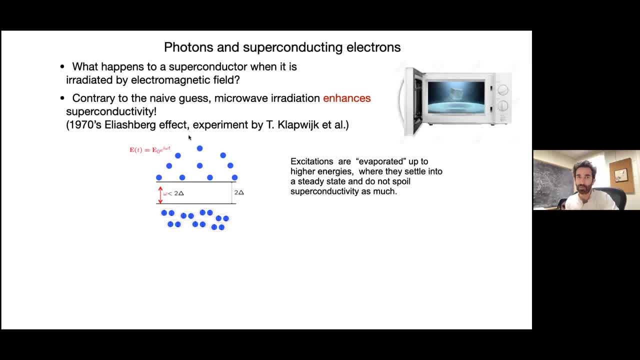 stuck and don't come back immediately, And that's how people kind of understand it in hand maybe. why? Why you can actually enhance it. And then there are also recent experimental groups in Cavalier's group that you can actually enhance it. So we asked the question: can we use the cavity QED? 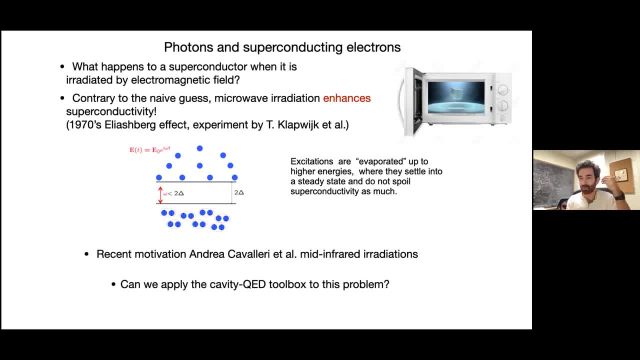 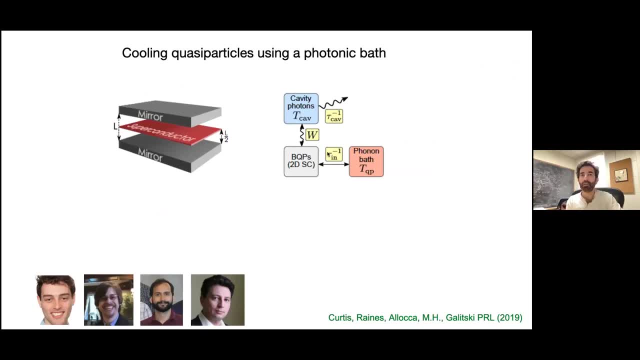 tools to enhance superconductivity, not just shine classical light, but if I just couple it to a cavity, and enhance it. So the idea is very simple. I have this Bougolev of quasi-particle that are thermally occupied. Usually my system is sit in a phonon bath at some temperature. But now, if I couple the system, 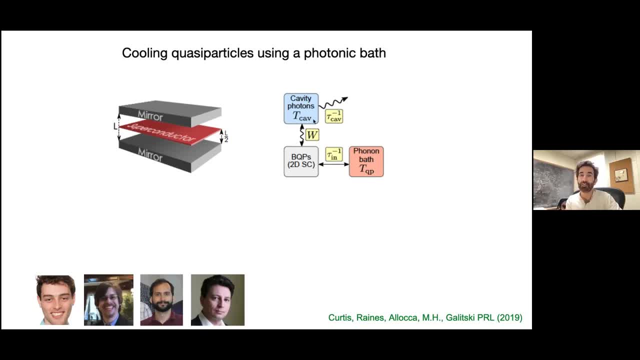 let's say very cartoon. I have a superconductor and I put it in the cavity to a bunch of photons that their frequency is held at some, their temperature is held at some temperature T cavity. So I have coupling to the photons and I have coupling to the phonons And this auxiliary bath. 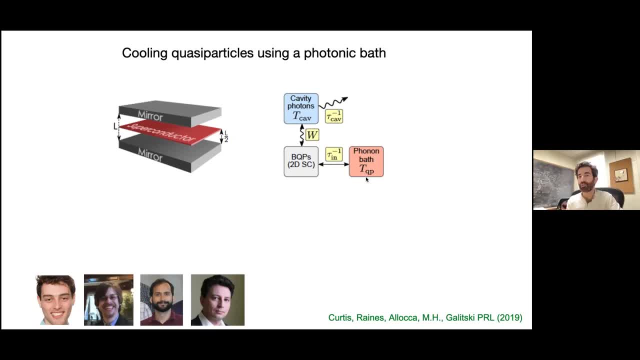 can cool the superconductor to a lower temperature than this T of the phonon, Then in principle I should be able to increase this gap. So that's a very high level way of understanding it. A little bit more technical, it would be that I have a gap. equation that comes. 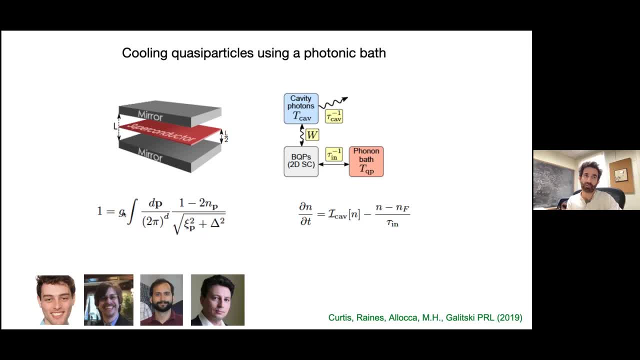 from the BCS theory. This is the strength of the coupling. This is the occupation of the Bougolev of quasi-particle And this is the gap. So by basically reducing the number of Bougolev of quasi-particle, by cooling them, then we effectively increase the gap. I have to solve this. 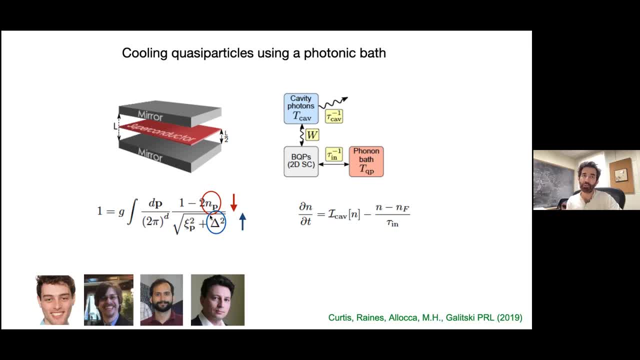 equation for delta. So by lowering this I can increase this. So this was a collaboration with my colleague, Victor Galitsky, and these gentlemen, who- none of them- are at JQI anymore. They're all graduated and left. So how can I understand it a little bit more systematically? is that I have to write the light? 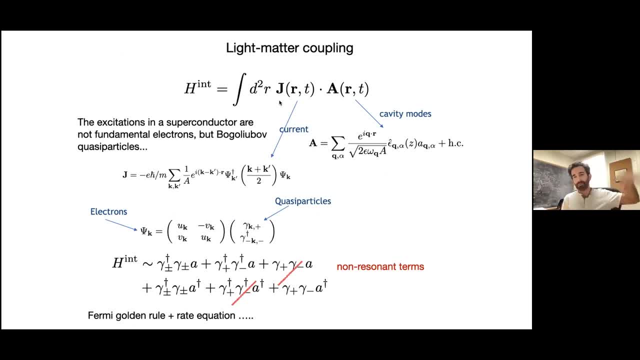 matter interaction. So this is a little bit technical, but I will zoom out again. Don't worry if you don't follow the details is that there is a current. there is the A modes. In the pre-talk we just we were dealing with one cavity mode. Now we are dealing with many cavity modes. 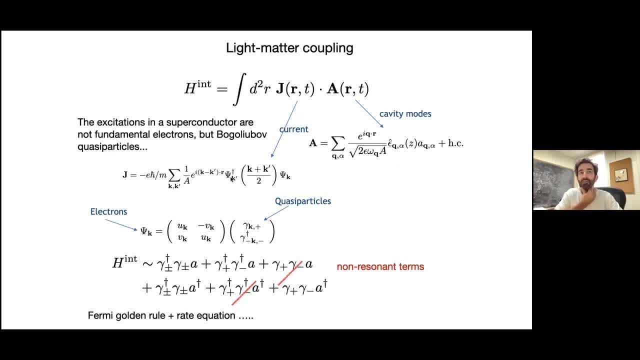 So I write it in terms of electronic creation and destruction operator. But I'm dealing with the superconductor, So I have to rotate it and then use this Bougolev of quasi-particle after a Bougolev of transformation, And then once you basically write the different 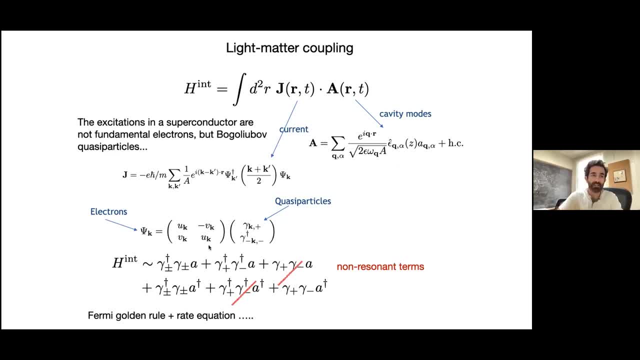 terms that come out. I have a six terms. One of them is the destruction of a photon and then creation of two quasi-particle, or scattering one, et cetera, And then some of them are just non-resistant, because this is destruction of a photon. there's also arowndal charge creation. 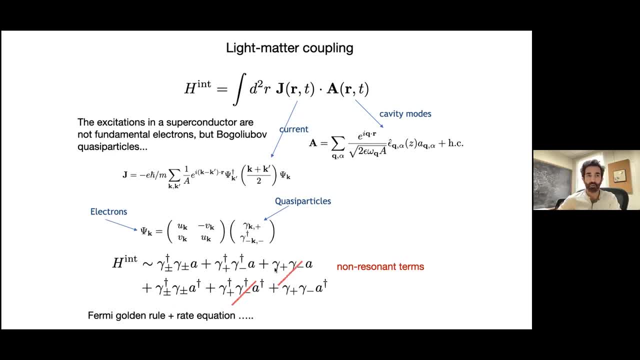 because this is destruction of a photon and then destroying two quasi particles as well. So these are non-resonant. So these two are non-resonant, We can neglect them, And the other four, we've taken them into account And then we just use Fermi-Golden-Ruhland rate equation. 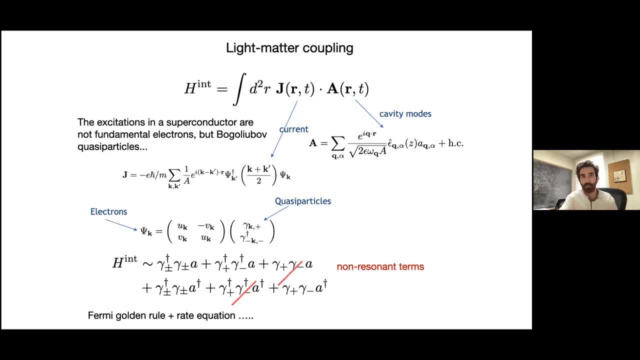 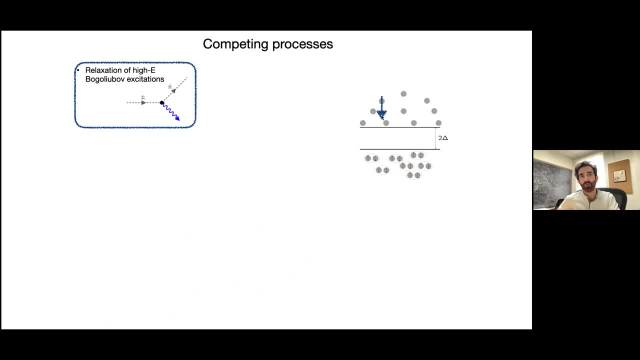 to find now what's the new distribution of the Bougliev of quasi particles. So one of them is that I emit a photon and I lower the energy of the Bougliev of quasi particle. The other one is that I absorb a photon and I increase the energy of the Bougliev of quasi particle. 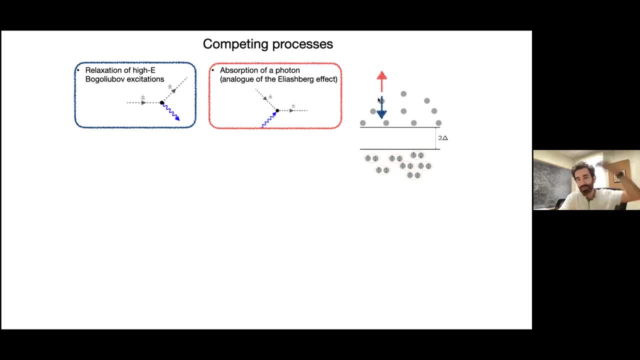 This is similar to the Eliashberg effect: that the photon is absorbed and I go to higher energy. I can also emit a photon and then form a pair, And this is good because I'm creating more pairs. Or the other way around, I am heating the system. 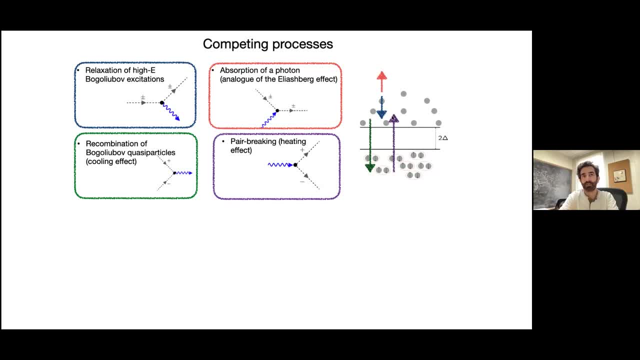 I'm destroying one of these Cooper pairs and creating two quasi particles. So these are all the form terms that I had in the previous slide And now, if I put everything together, calculate the new distribution of the Bougliev of quasi particle and then solve for my gap. 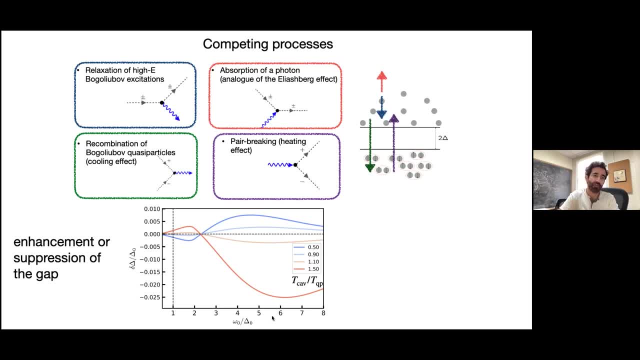 and look at the gap enhancement as a function of the frequency of the cavity. we see such a thing In particular. if the cavity is cool, is colder than the, than the temperature of your phonon, then you see an enhancement of these guys. 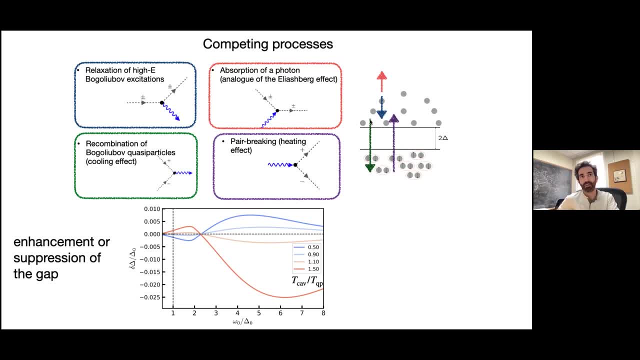 I have to say these are competing with each other. So red is good, green is good, but then blue and purple are bad. So one has to just solve it and then see what's going on If the temperature of the photons are higher. 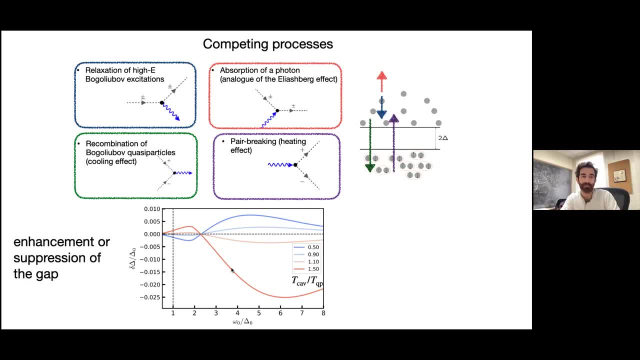 than the temperature of the phonons, then we don't see any enhancement, We see suppression. However, if the frequency of the photons that are very hot is lower than the uh, the gap of the superconductor, then you enhance it and that's basically ellie. 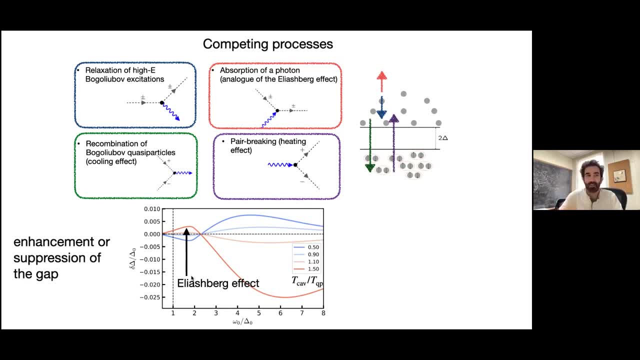 ashberg effect, because remember that the photon was below the gap, it would enhance it. but here i'm just thermally doing that. so in that theory of ellie ashberg that we were dealing with coherent photons, the coherence actually did not really matter, the number of photons. 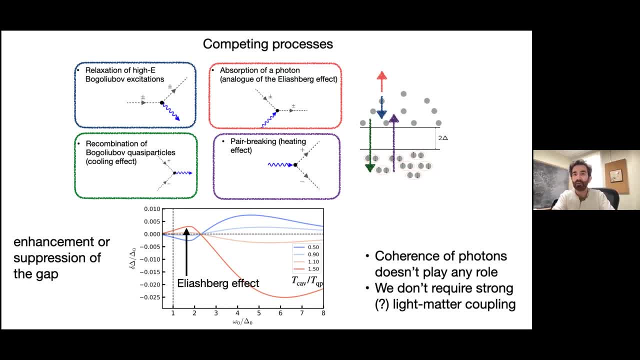 mattered over there. so what we have here is that coherence of the photon does not play a role and we didn't really require a strong light matter coupling. i have to say this is strong still, since we don't have is this two-level picture and james cummings, hamptonian, the 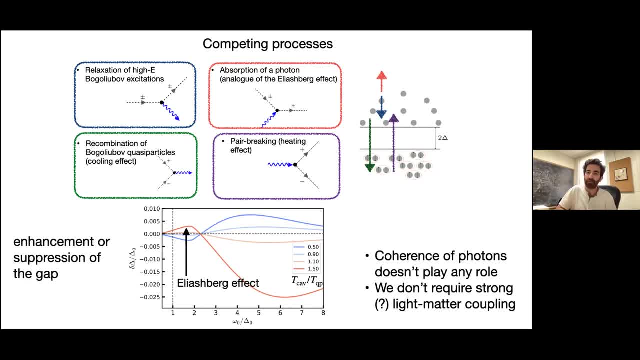 word of strong coupling. weak coupling should be taken with a grain of salt, and and we are still trying to understand what the strong coupling mean in this iternal electronic system. so now, yeah, uh, hi muhammad. so in in this plot, there's an interesting point where all 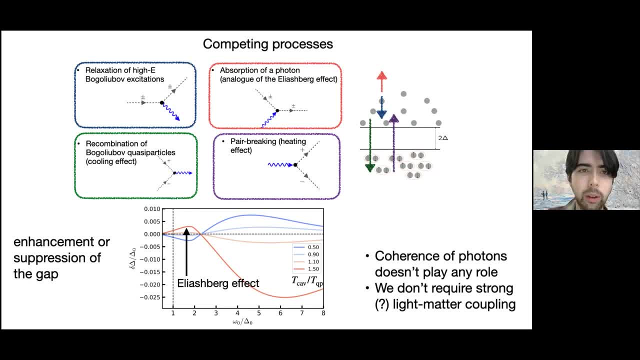 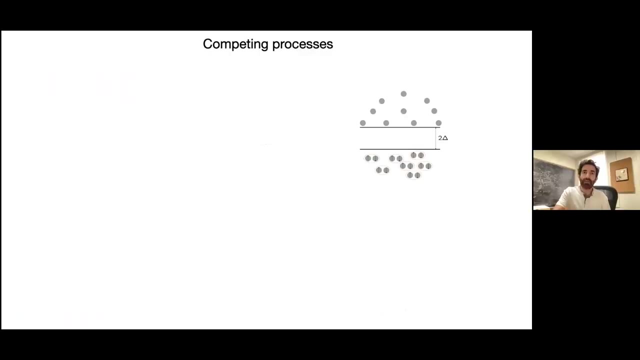 these temperature curves intersect at like omega, over delta, like 2.3 or so. is that, is that physics, or is that just some artifact? um, i think it's the art we have, because once you do it for a multimode, then things can can change. okay, so now, now that we have this, then we- i said that the 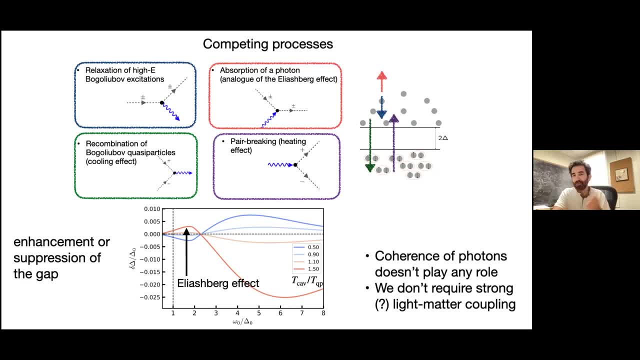 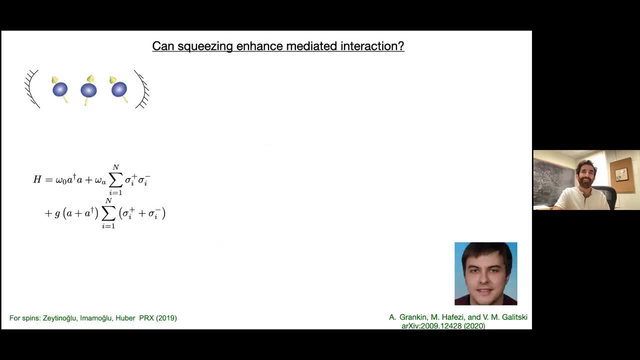 coherence of the photon does not matter. and now let's look at some other kinds of uh photons to squeeze the state, that's the, that's another type that we all know and like and um. and let's just assume like a vacuum squeezed state, uh, let's put the itinerant electron on the side. let's. 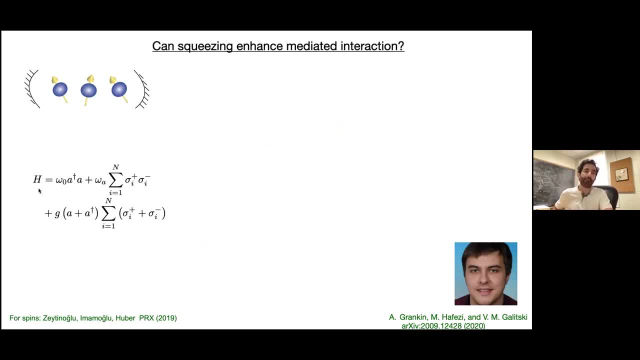 consider a bunch of spins, two level systems that are coupled to a cavity. so this is the energy of the cavity, this is the energy of the spins. you and i have the coupling of the spins to the cavity. now, if you look at this term, this is one. 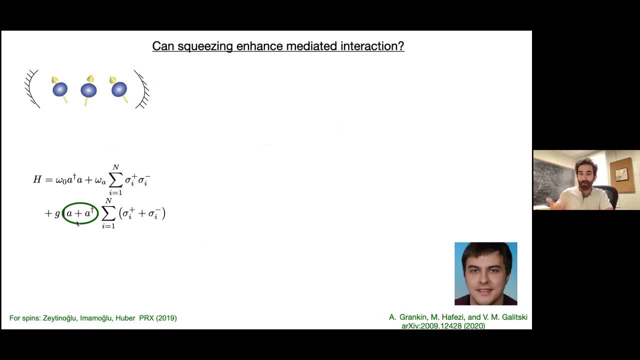 quadrature of the photon. this is the x quadrature. i'm coupling to the x quadrature another p quadrature. so if i somehow squeeze this x quadrature then i can effectively increase this coupling g. so that's basically the idea of uh, squeezing the light in the cavity to enhance. 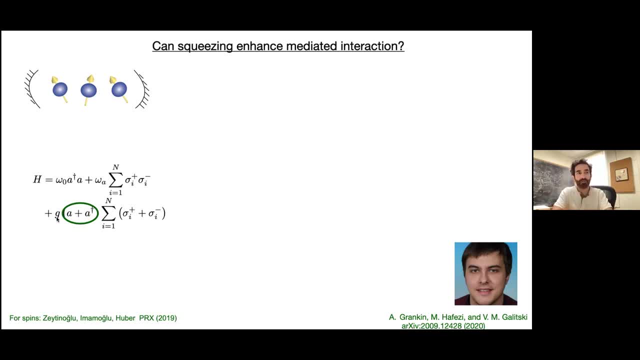 the g in the james cummings model. but one has to be careful, because uh, squeezing is always defined with respect to a local oscillator. so what do we mean here? and and unless some in some literature, it was actually uh ignored. so this is the cohere, this is the parametric drive that we need to to. 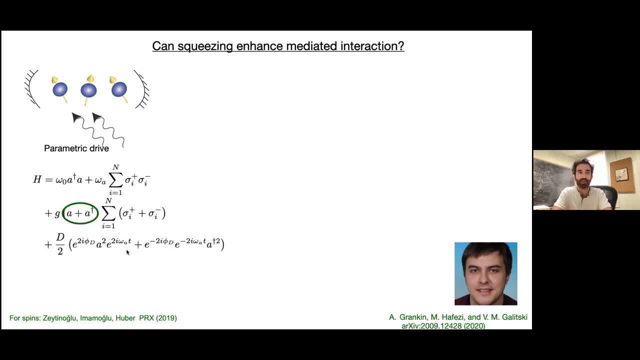 squeeze this quadrature. so this is the squeezing operator is a squared plus a dagger squared. if you apply this operator, it squeezes one quadrature of the photon and it squeezes the other quadrature versus the other quadrature and enhance the fluctuations of one quadrature versus the other. 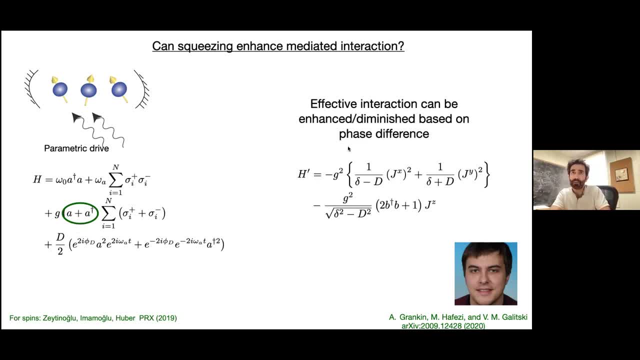 so now let's go back to the caveat that i said. if i now write the effective interaction, uh, so i integrate out the photonic degree of freedom and i look at what spin spin interaction i can mediate. you see that this is the detuning, this is the amount of uh squeezing that i have in the system. 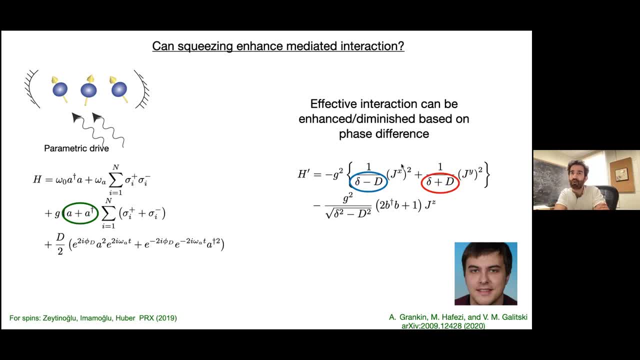 i'm enhancing the coupling for one uh type of interaction and then decreasing the interaction for the other one uh. that that's going to make sense now. if i choose chose a different uh quadrature, then i will do the same. so it's actually a phase sensitive way. 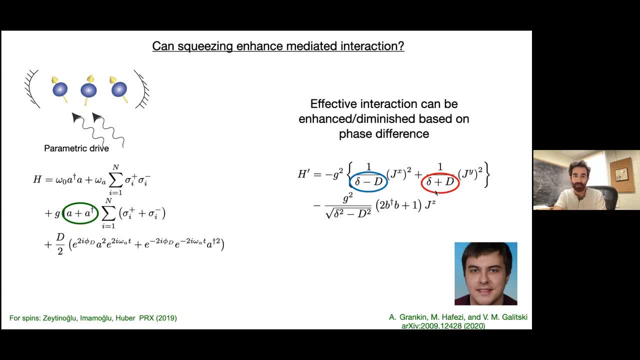 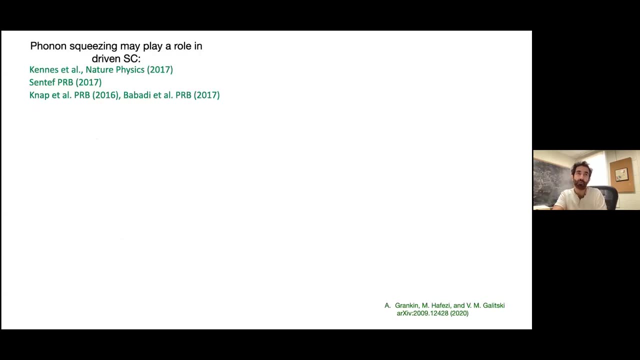 to enhance the interaction, and one has to be careful with that. okay, so now with this introduction, we can go and look at the internet electronic system and then look at superconductivity and uh, there was some work recently that, uh, experimental work and followed by some theoretical. 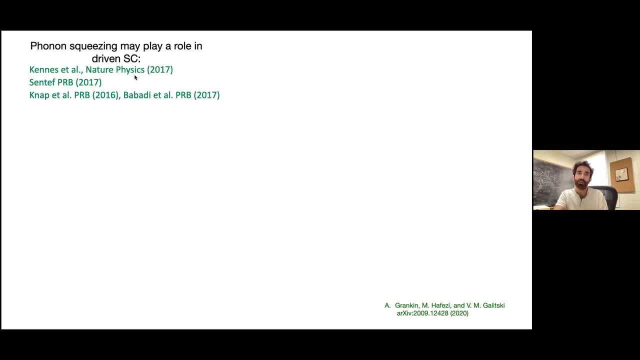 work that phonon squeezing actually may play, play a role in in these three and superconductors. then the question that we ask is that: can we inject the squeezing by hand so i have some light that has some squeezing? can i inject that, turn that squeezing into a phonon squeezing so that that's 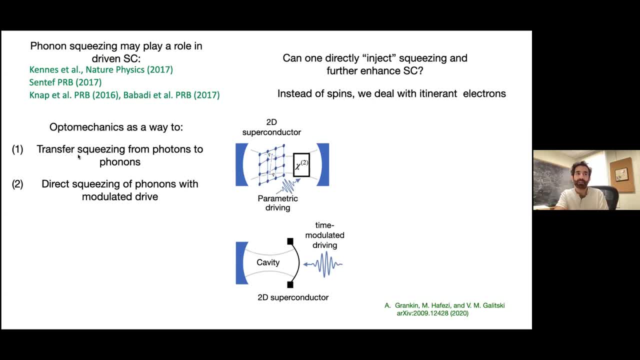 one option. so i use opto mechanics to transfer the squeezing of photons, phonons. let's say, I put the superconductor in a cavity with some parametric drive, so this will lead to squeezing of my cavity mode and then that squeezing because of I have optomechanical. 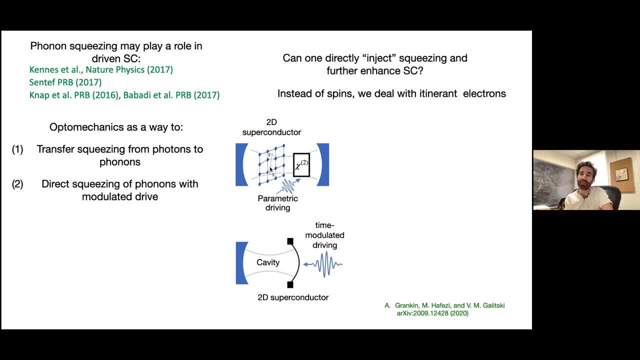 coupling, it will translate into squeezing the phonon and eventually that should enhance my superconductivity. the second option is that I squeeze the phonons directly through modulated drive. so this is my superconductor that forms also a mirror and a mirror of the cavity by 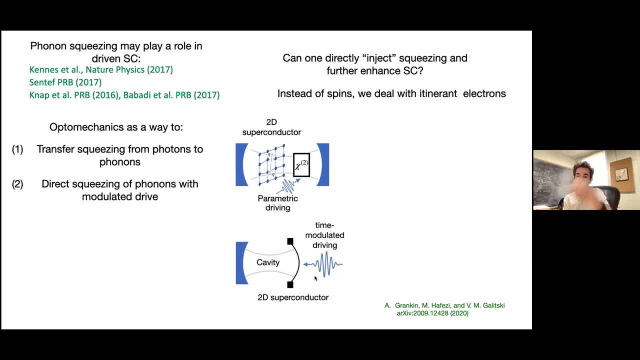 time modulating the drive, then you can squeeze its phonon and we may actually enhance the superconductivity. so the hamiltonian describing these, these two systems, is the same: you have a bunch of phonons and then you have a bunch of photons. the photons are driven from outside. 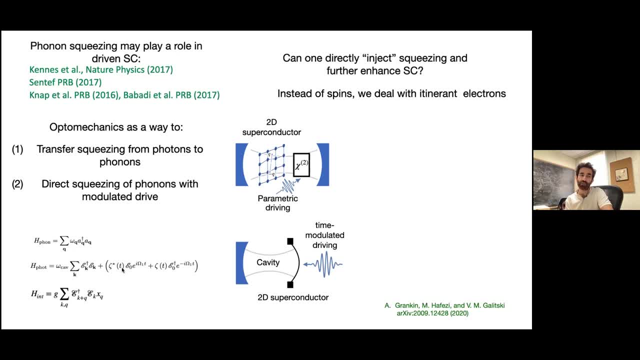 as a time modulator. this, this is the time modulation of the drive and this is the strength of the drive. and then you have some optomechanical coupling, which is basically the: the position of the mirror times the frequency of the cavity. once I move, I change the frequency of the cam. there is a 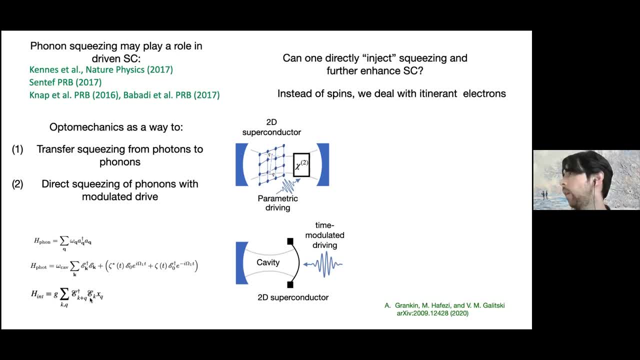 there is a question. yeah, so I think I didn't cover this in my introduction, the notion of photon quadratures or squeezed states of light, so could you just give like a few brief remarks to give some intuition on what, like this squeeze state is and then why it might be interesting? yeah, sure so. 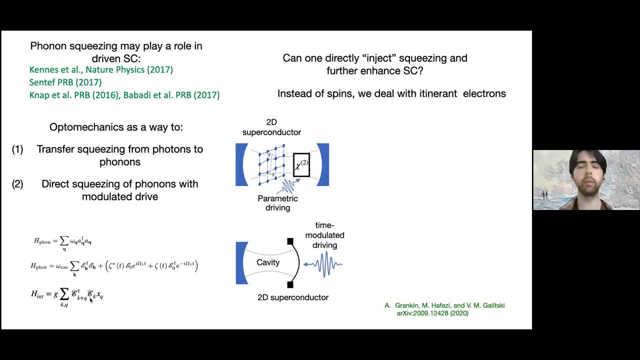 my cavity mode, a single mode, is described by a harmonic oscillator. so harmonic oscillator in a classical picture, we know that it has x and p and it oscillates as a function of time. now, this is the classical picture. the quantum picture is is the same. you have a bakelite so you get the state over here and this is the function of time and 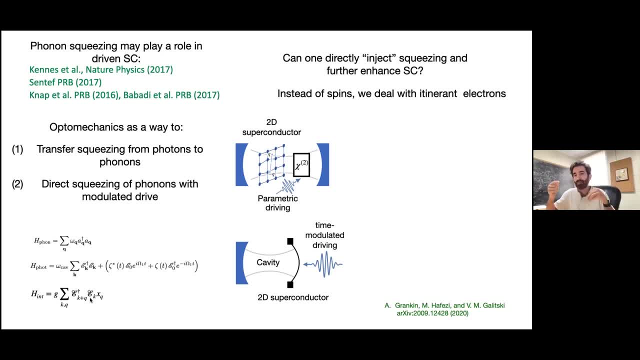 that's the play within that play within that playing around. and then in of half we have a Morganielen weak piece of solid and then in the second way this plays around, we have the taped. squeeze it in one direction, but it should go in the opposite direction. 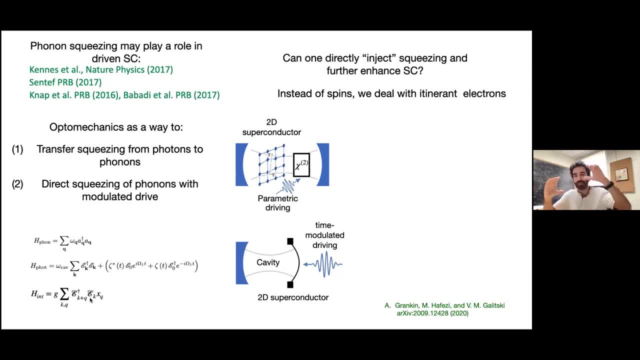 such that Heisenberg is satisfied And you can squeeze it in the X direction or you can squeeze it in the P direction. So what I was saying in the previous slide is that it really matters what quadrature we are squeezing, And I hope that brief introduction to squeezing was enough. 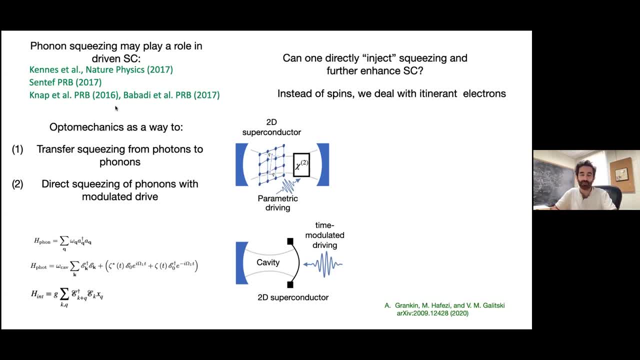 And these papers. they made use of the fact that the Hamiltonian had some specific form, So you would actually enhance the quadrature automatically that you want. But if you want to do it optically, then we really have to be careful with what phase we are coming into the system. 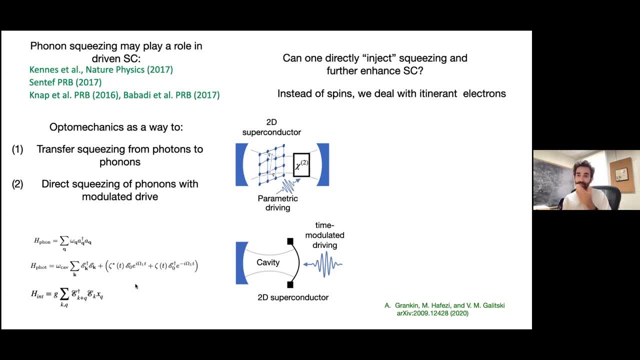 with respect to the local oscillator, And then that would. it's a little bit more complicated, But we have to determine whether we are enhancing or inhibiting superconductivity. Great, thank you so much. So now I can have this TC, the critical temperature. 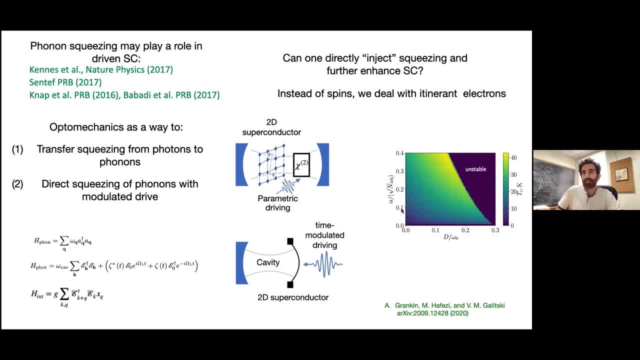 as a function of these two parameters. One is the classical drive and the other one is the amount of squeezing. If you squeeze too much, then the system can go unstable, But if you squeeze a little bit then you can actually enhance TC. 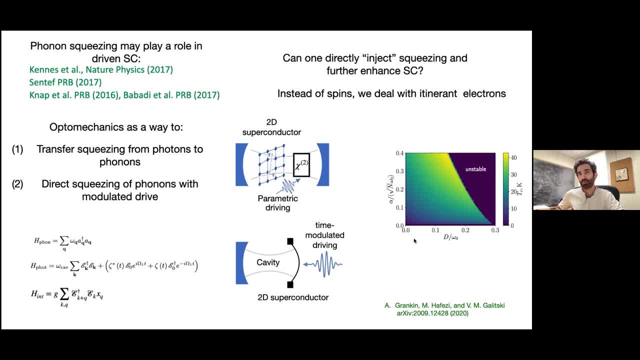 So what these works were before was just we were looking at the zero squeezing from outside and then doing this classical drive. Now we just added this access to it that we're using this squeezing can even further enhance it. So now, this concludes the squeezing part. 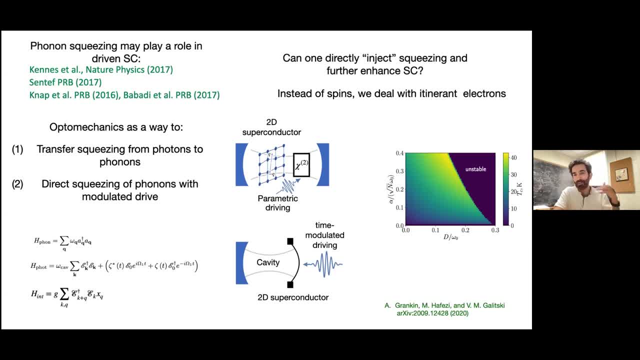 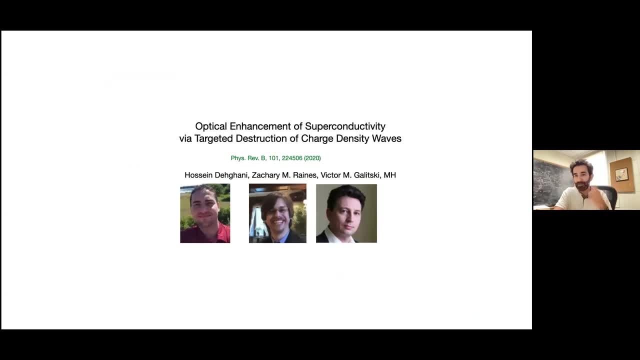 Now what if we just go a little bit step backward and then just use a classical drive as a way to optically pump the system in Sub более ven toute? This concludes this squeezing part in a regime that we want, And this is the work that was led by Hossein Dehani. 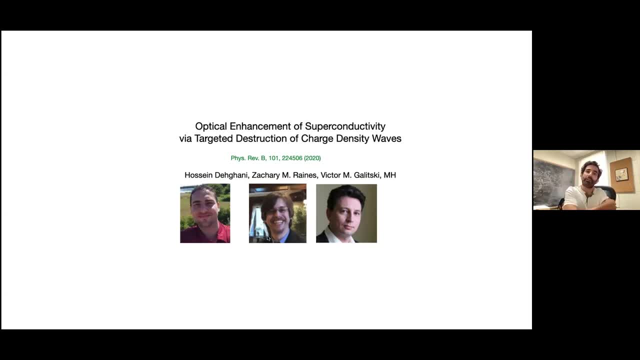 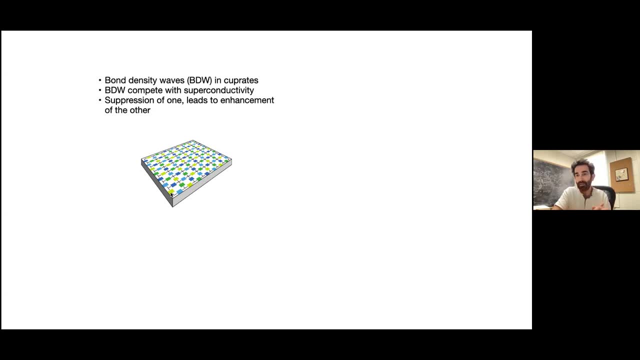 my postdoc in collaboration with Victor and then a former graduate student, Zach. So the idea is that in many superconductors they have competing order parameters. One is superconductivity, the other one is charge density wave or bond density waves. 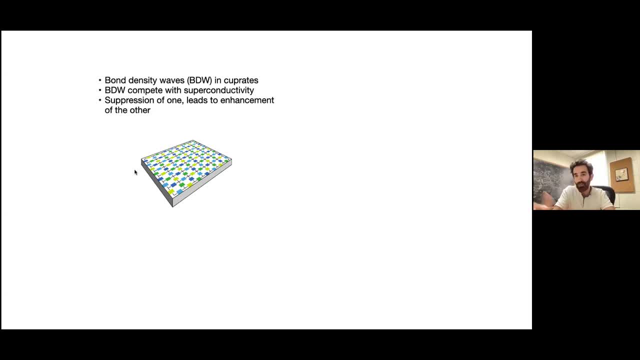 So, and then suppression of one would lead to the enhancement of the other one. So the idea we had was the following: is that if these charge density phases have some excitations that we can excite optically, and we'd send them somewhere like Eliashberg effect, 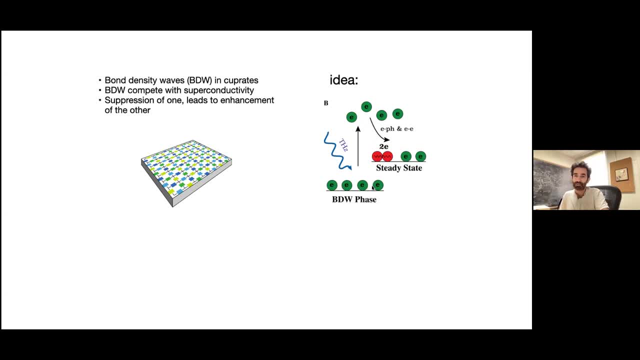 and hopefully they will settle in some steady state and don't bother us immediately. then we can enhance the superconductivity. So one issue here is that these bond density waves, they have some dispersion and the dispersion is dictated by the electronic degrees of freedom. 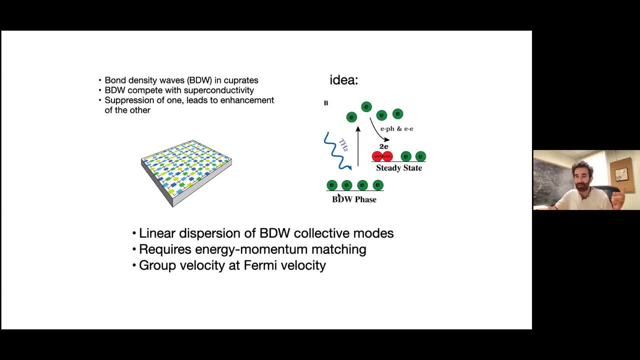 And the simplest model that you can write. it has a Fermi velocity in it, So that the Fermi velocity will just come as the dispersion of those collective modes. So now, if I want to couple something which has a dispersion with Fermi velocity, 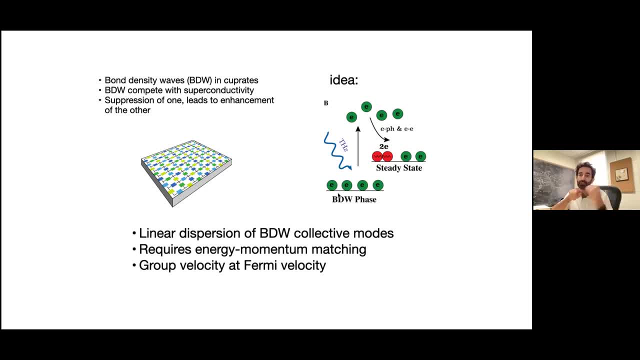 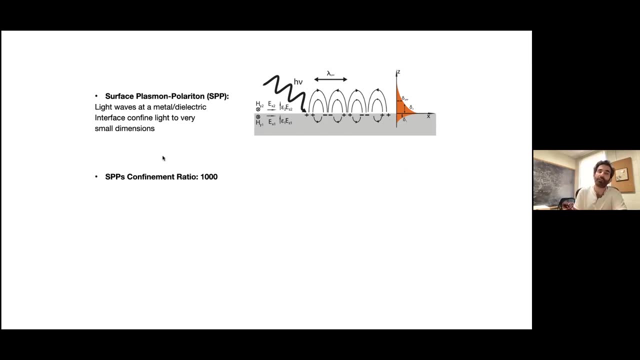 then I have to shrink the wavelength of my light such that they can resonantly couple to it. So the energy momentum, a matching here, requires me to really shrink the wavelength of light, And for that we came up with this idea to use the surface plasma polarity. 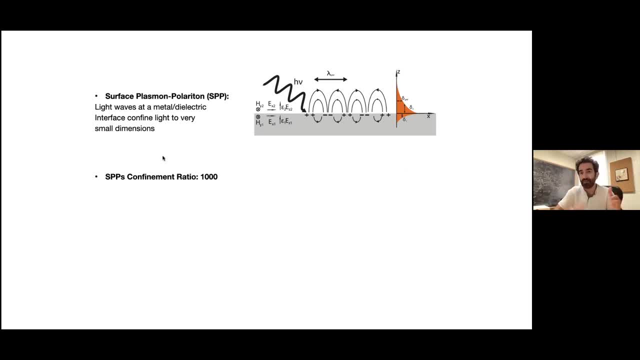 So you come with light from free space, that surface plasma polarity are a way to shrink the wavelength of light for the same frequency. You don't change the frequency, you just change the wavelength And then using that match that dispersion and then evaporate it. 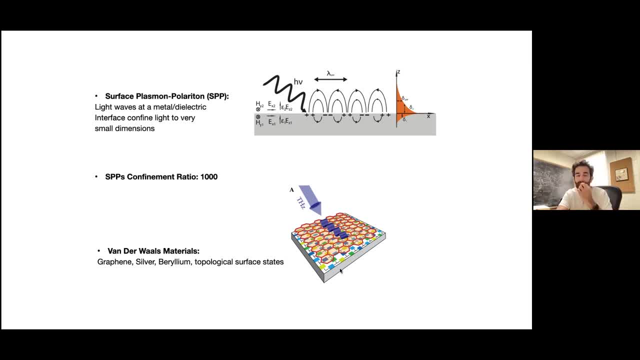 So that's kind of it. So that's kind of a theoretical proposal that we have put forward and might be interesting to pursue. So most of the things, everything I'm actually talking today, is all theoretical and proposals that we are working on. So now we can take one step even further. 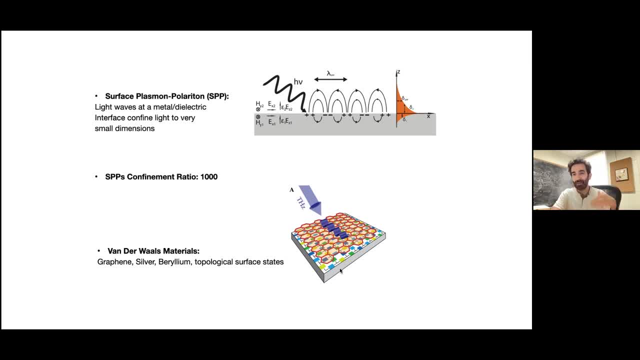 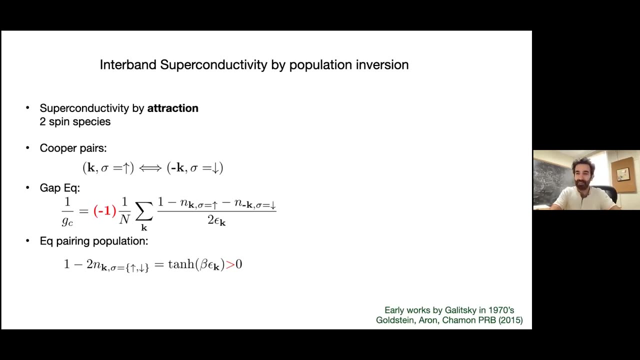 not look at light enhanced superconductivity. look at light induced superconductivity with light. I'm being redundant here, So this is an old story. of course, This goes back to many, many decades ago that I have a semiconductor. can you shine light and then making it superconducted? 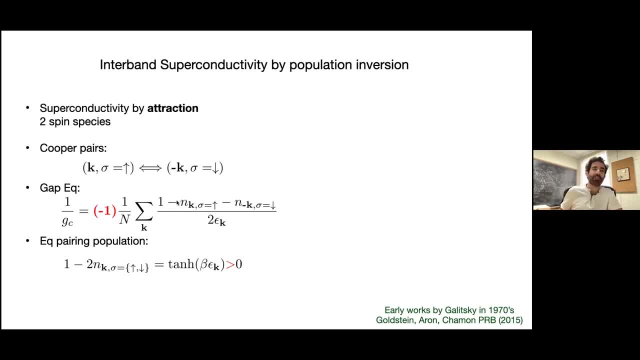 So the idea is kind of simple. If you go back to the BCS theory, you have this Cooper pair. you have two electrons with two opposite momenta and different spins and I can pair them And I write this gap equation, similar to the gap equation that I wrote in the beginning. 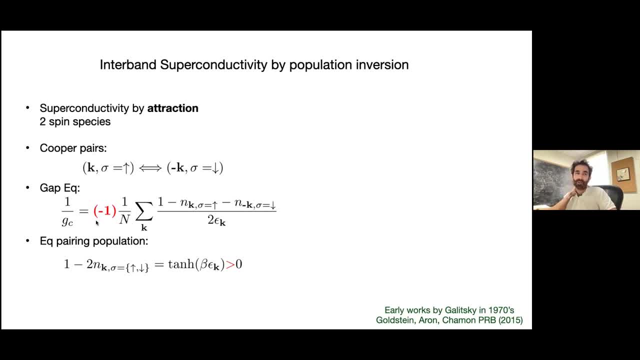 Here is the linearized version of it. Basically tells me that whenever I have a situation like this and I have a non-zero G, then I have non-zero pairing. The critical point in this equation is that I have to have this negative sign over here. 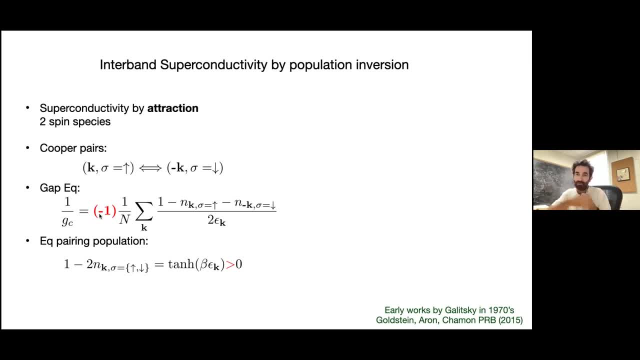 meaning that I need to have attraction- This in the BCS theory is coming from phonon- to get a non-zero pairing. Because if this boolean of quasiparticles of these original electrons are thermally occupied, then always the sign of this is positive. 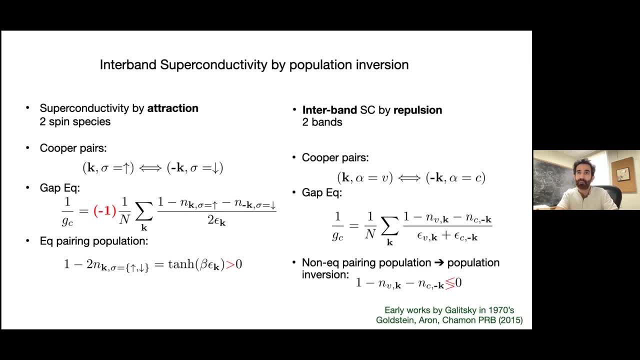 So I need a negative sign such that this works out. But now here, if I consider now the electrons are from two different valleys or from two different flavors. one is K, one is minus K, but one is coming from the balance band. 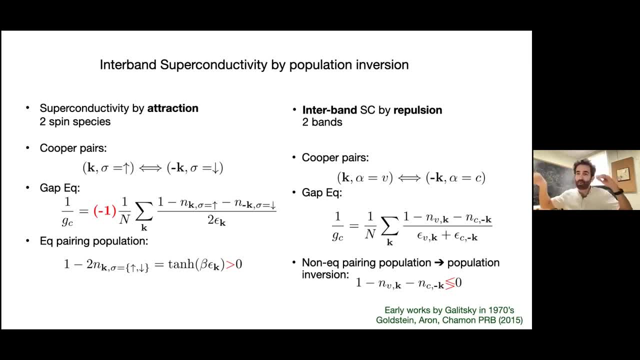 The other one is coming from the conduction band or from, like, two different flavors, And if I can prepare the distribution of these electrons in one of this flavor and the other flavor independent of each other, such that they can play with the overall sign of this expression? 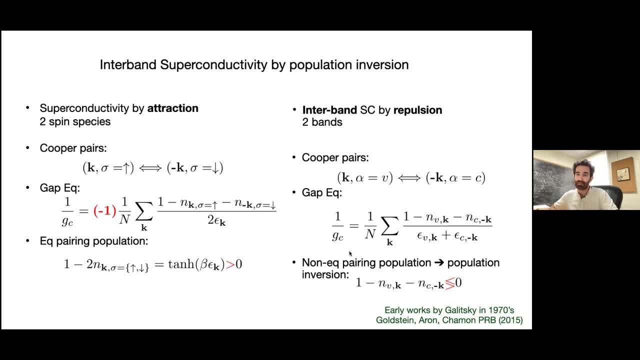 then I can have superconductivity with even attractive, with even repulsive interaction to start with. So that's the key idea. So now, how is it possible? The way to do it is to have these two flavors, to be able to optically select these two flavors. 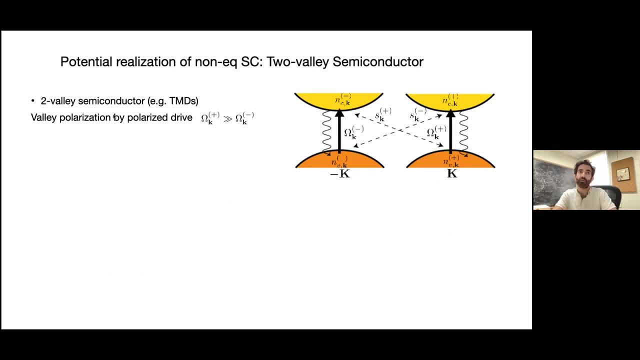 And that has been shown in many systems, including transition metal called galgenite, that you have two values. then, depending on the polarization of your light, you can talk to one value versus the other one. In particular, you have a K M N K, but one value versus one. Should I have a K M N K or M? I have a K M N K, I have a K M N K or M, And I have a K M N K and I have a K. It's not a K N and I have a K N K. 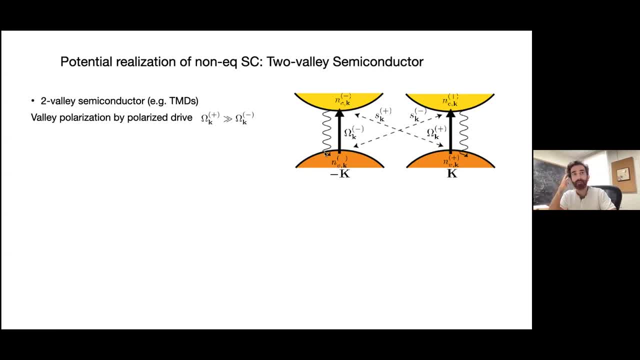 In particular, you have a K and K prime minus K or K value. One polarization- right circular polarized talks to one value and then sigma minus talks to the other value, the majority of it. At the center of the band. you have 100%. 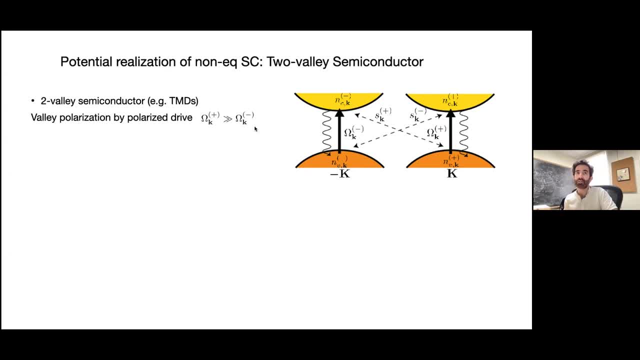 but when you deviate it changes, But that to a large extent you can assume that if you're shining sigma plus light it will couple to one value and not to the other value. So now I have prepared these states, these populations, kind of in an independent way. 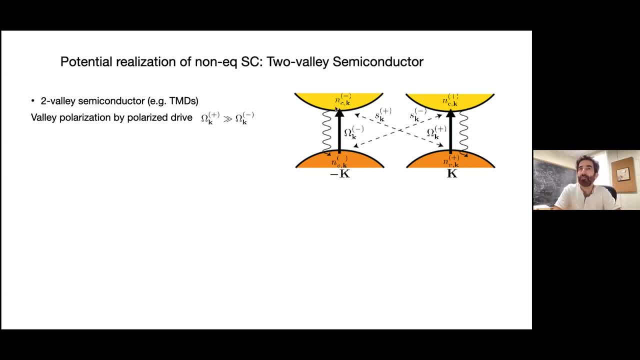 I talk to these guys and maybe do half half here and then zero one over here. So by coupling this now, this will be my new bands. So, depending on the frequency of your light, you will couple this band in the rotating frame. 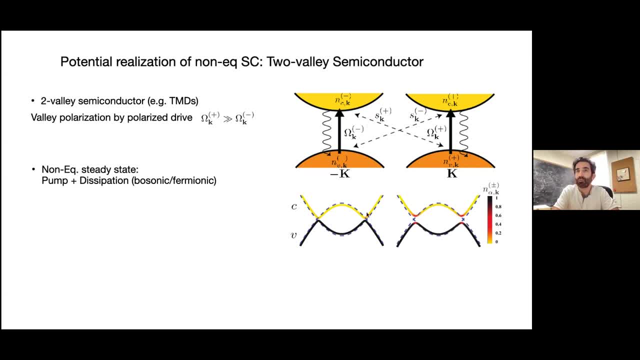 This band will come to this and then this band will come to this. In one of them you have some coupling, like the Robbie that we had in the pre-talk is probably. frequency is non-zero, So you open up a. you have a crossing over here. 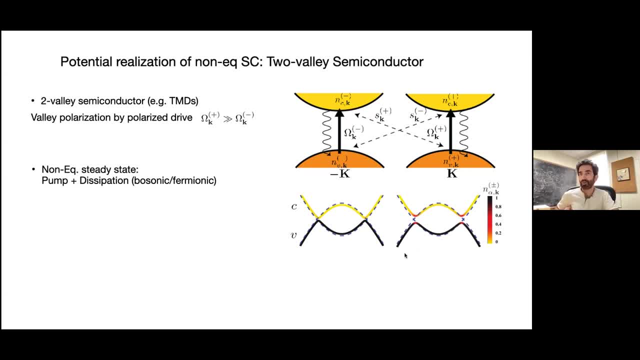 In the other one you don't, because this is very, very small. So if I plot the density that the population as a function of momentum, then in one value is different than the other one. Now I can consider the pairing across the value. 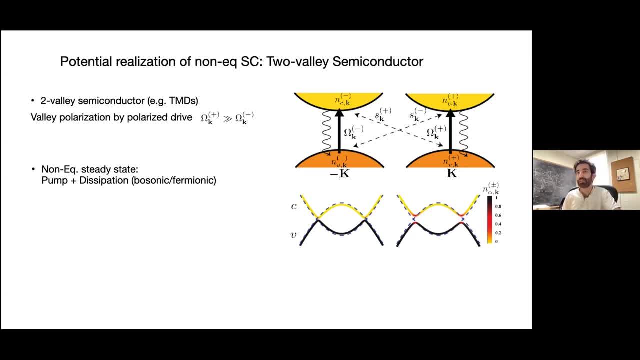 when electrons with different momentum that are coupled to each other and electron that are coupled to each other other, and indeed in some regimes I can have them to be positive or to be negative, that population term that I had in the previous slide. now, what about the interaction? now we have Coulomb. 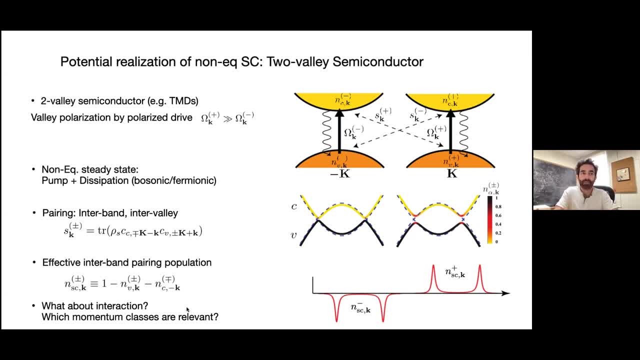 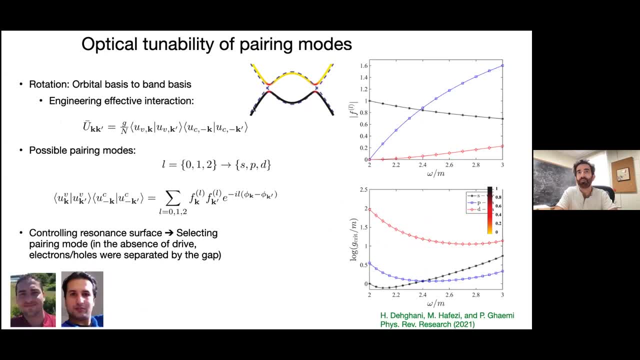 interaction and the interesting part is that the frequency of the light would determine where this crossing is happening. so this is the crossing and this is the frequency of the light. it can be it can cross at this point or it can cross at this point. so the now the, the electrons that are 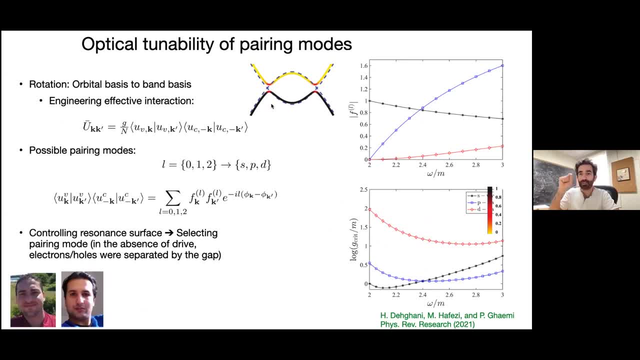 important are these electrons by? so, by choosing the frequency of the light, then the momentum classes I need to consider to put back into my equation to get the non-zero pairing, are coming from here, or maybe coming from here if my light was coupled at the lower frequency. so, depending on the frequency of the light, I can look at the different forms of. 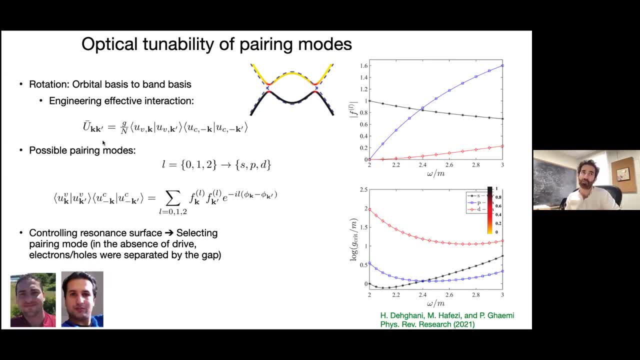 different parts of coulomb interaction that enter my equation. in particular. I have to write my coulomb interaction in this band. I have to project it in this band and then look at different different channels. that is like s wave or a p wave or a d wave. just I'm not going into the details of it. 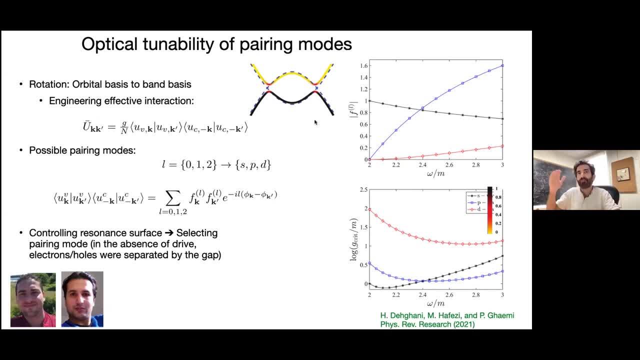 just the fact that the, the frequency of my light, would determine which momentum class is relevant, and then that frequency will tell me which mode is more favorable. so this is the critical- uh, critical- coupling as a function of frequency. you see that here it has a lower value and then 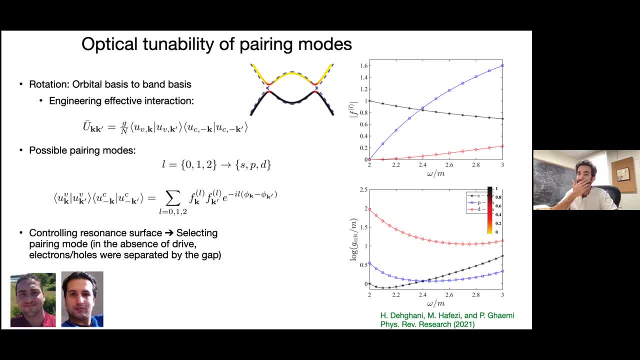 here the s wave has a lower value. p here has a p wave as a lower value. so what we did in this uh, in this work, is that not only we use light to selectively have this population, but also the frequency of the light can determine what form of interaction becomes more relevant. so it's a way to 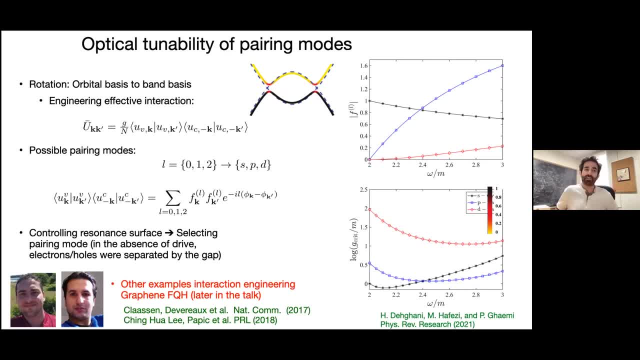 change the frequency of the light so we can use light to selectively have a more linear reaction and then use this interaction engineering- I have another example of it using in the fraction of quantum hull case in graphene, and then there are also some other works from other groups- how we can use this drive to have different forms of interaction. so, Marcus, how much? 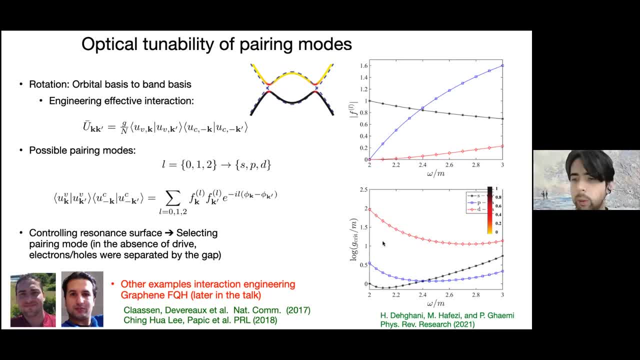 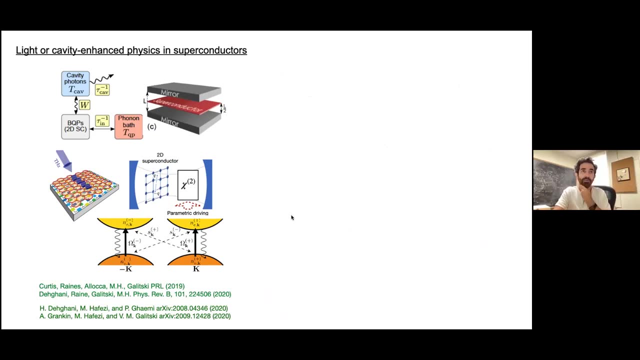 time do I have? because I it's a non-conventional right, so I think I passed it over to you at. you have about 20 minutes left, very cool, okay. so that's the. that's the first part that we looked at various ways of playing with light matter interaction: to, to enhance or to induce. 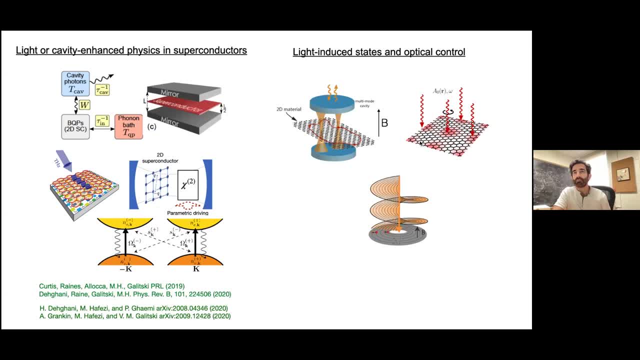 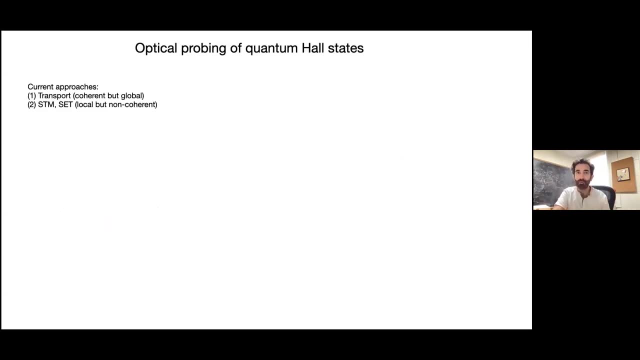 superconductivity. in the second part we will explore, like topological states of electronic systems, how we can use light to make some of them or to measure some of them. so this requires a little bit of a background in in quantum hall so i will very briefly go over it. so most of the probes 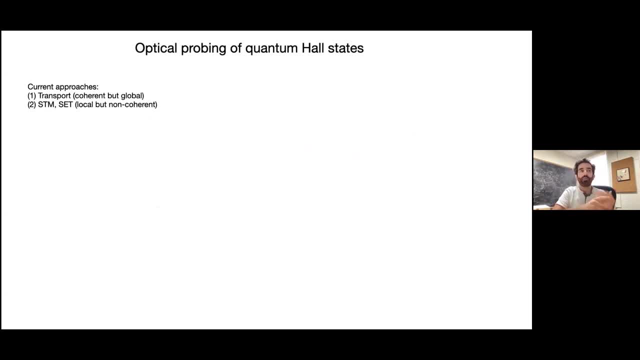 in in quantum hall. the electronic ones are in two form. one of them is transport and it's global. you look at the conductance and you can have global properties of the system, but it's not local. you don't know what's happening in the system and you can't see it. you can't see it. you can't see it. 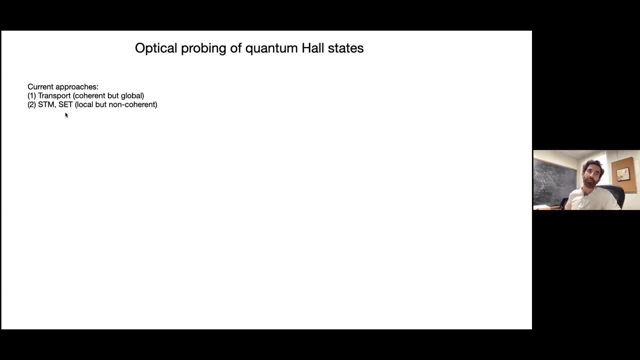 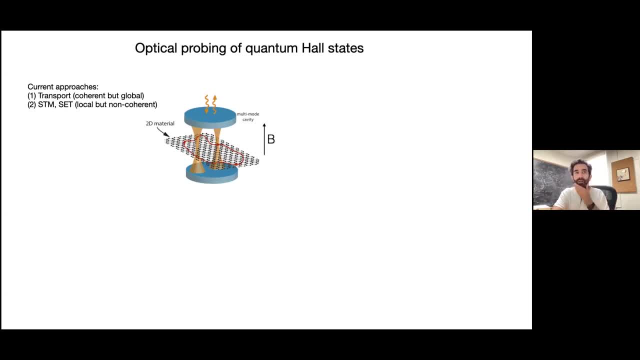 the idea is that: can these optical techniques be like a complementary way to uh to measure them in the first space, in the first step, and then later to manipulate them? uh, so in a particular case, you can An었어요 look at this kind of problem. you have the quantum. 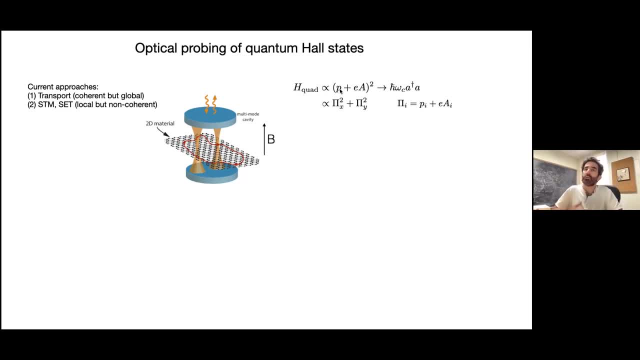 trope here, where you you also might be interested- by the elliptic scale, when you have some such magnetic fields in to a quadratic field like the x 조 of quantum venir. and now, when we, when we have a, a quadratically dispersive electronic system, we have like a p squared for the dispersion of the electron, when you apply, uh, some electromagnetic 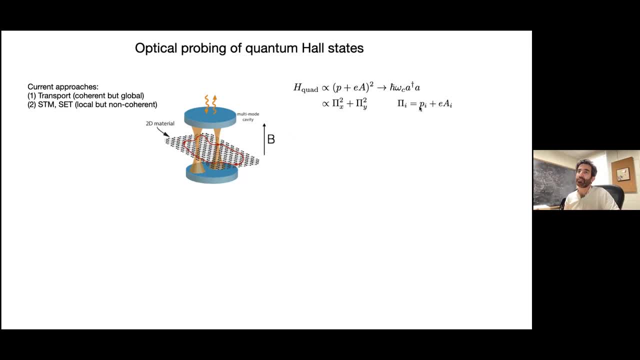 fields, in this case a static magnetic field, then you do minimal coupling, you have you have something x, x and y direction and you immediately see that when you look at the commutation relation of this pi x and pi y, if the magnetic field is uniform then they satisfy the commutation relation of a. 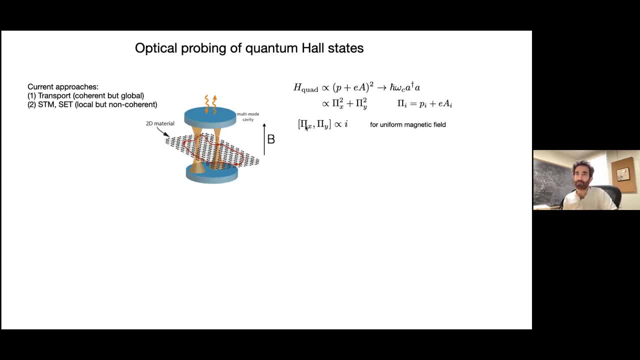 of a harmonic oscillator, so like an x and p of a harmonic oscillator. so then you can actually define the ladder operators etc and then write your hamiltonian as a harmonic oscillator. so this is actually what leads to london levels. so if you have two-dimensional electron gas and you put a 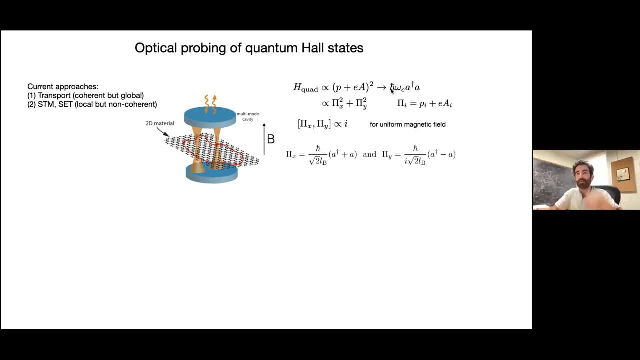 magnetic field. you know that you get this equally spaced london levels. a very quick way to understand it is actually to do this two-line math. now, hi, mohammed, sorry, uh, i misspoke. the organizers reminded me that we want to leave plenty of time, uh, for discussion at the end, so could? 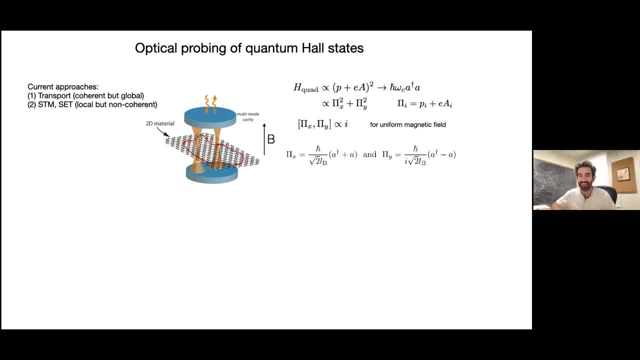 we do. instead of 20 minutes, could you do 10 minutes? ah, okay, sorry, so then say 10 minutes, okay, good, no, no, i, i keep the same speed. it doesn't matter. i don't have to finish all the slides. so the key here is that if you start with graphene, that is, linear dispersive, then your 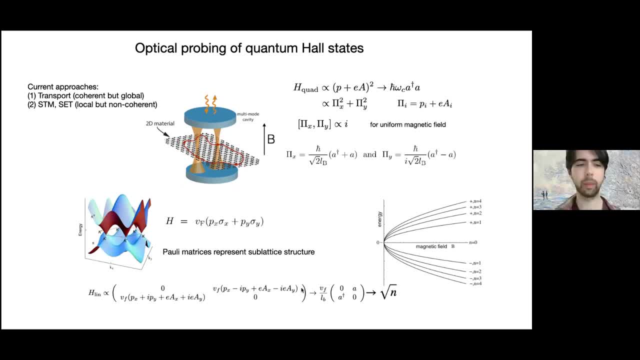 form of coupling is different. uh, you have, uh, you have this, uh pseudo spin structure, and then you end up with this hemi. you do the same uh, you get the same uh replacement, and then you have to square this such that you get your harmonic oscillator. that's why, instead, 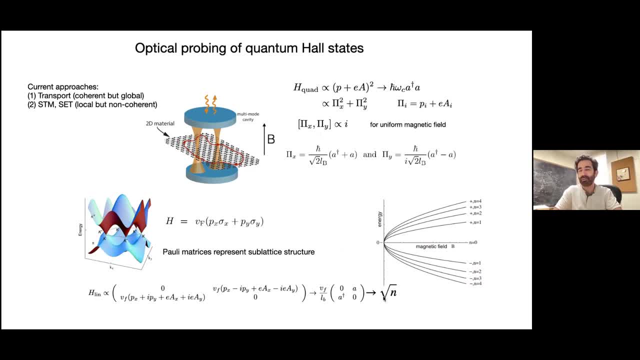 of now, having equidistant londo levels, you get the londo levels that go at the square root of n. so as a function of magnetic field, the londo levels are not linear function of magnetic field but they bend like this. why this is important? because it allows us to selectively- uh, uncouple. 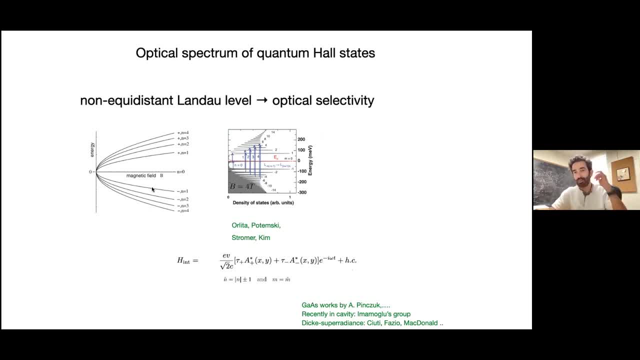 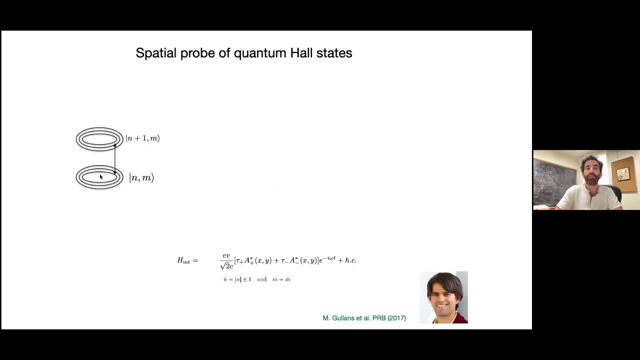 to them. if it was a linear uh situation, then you could not selectively couple to one londo level 2 londo instead, and you could know basically in a r legs group and you could detect this, in this case your spitting unit and the next Ref. 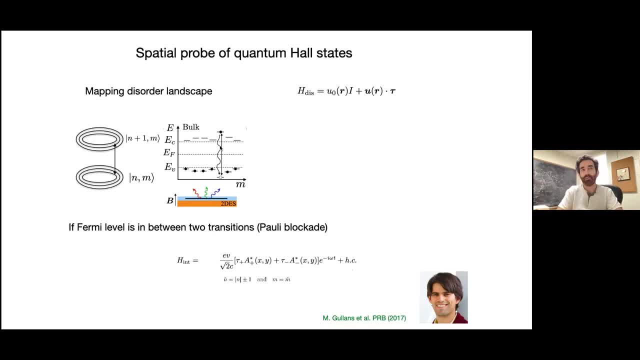 over there london orbits, you excite them and then you look at the photoluminescence and say then, by monitoring that this is a simulation, not by michael collins- is that if you have such such disorder in the system and if you resolve it, then you can reconstruct the, the the disorder map. now 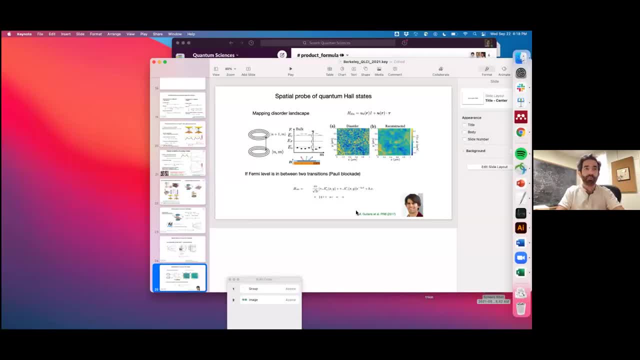 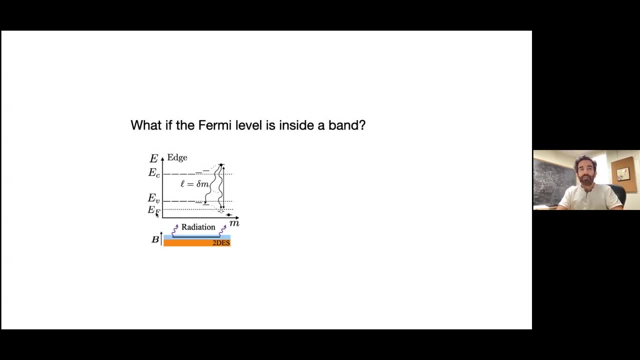 uh, i, i jump over this now. uh, what if i put my family level inside the the valence band, not in the middle of the gap inside the valence band? then i can actually excite the photon over here. the photon can come back and recombine with the electron, can come back and combine with the hole. 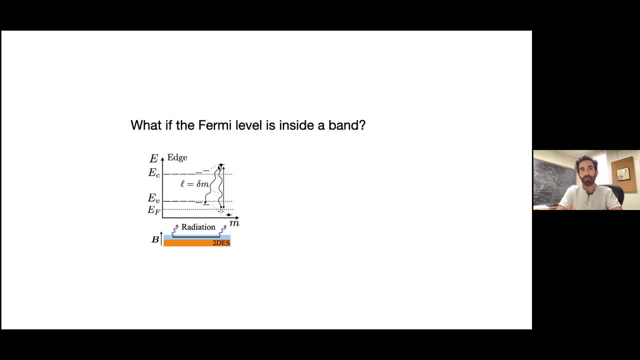 but it can also go to the other states. in principle they are allowed, and so you can see that the valence band is not in the middle of the gap, but it's in the middle of the gap. can it actually happen? and we know that these states can be actually very large in principle. 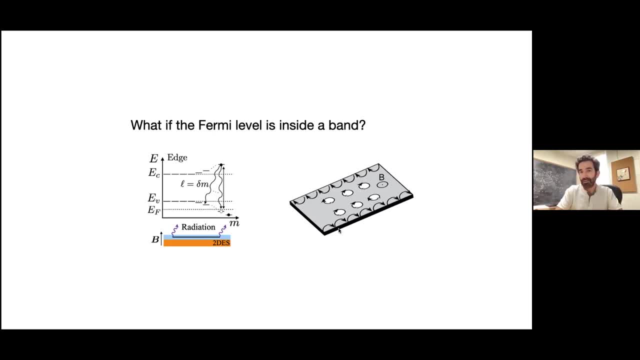 so you have some edge states that are very large in the system and is does it become a problem at some point? in most cases in quantum optics the electronic wave function is much smaller than the wavelength of light. so you do the ipol approximation and everything is fine. but if 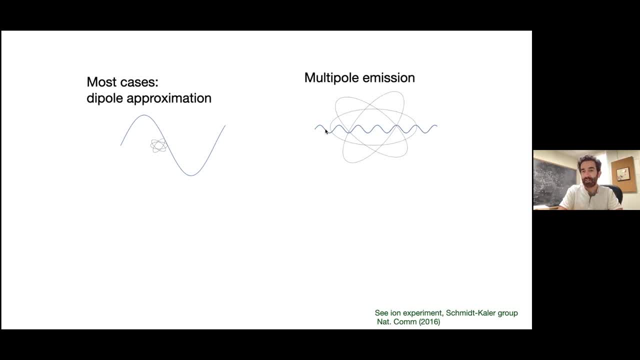 the electronic wave function is large. then you have higher order transitions, transitions that are not usually allowed. so you usually have the s to p transition. but s to d transitions are allowed, uh, it's just they're very, very weak and experimental. actually they have been observed, uh, but they're just weak. so now, in this quantum, 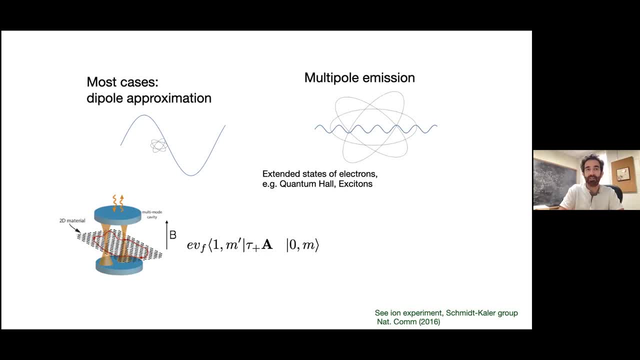 hall systems. they're very large, so there should be some manifestation of it. a very easy way to see them is to just look at the fermi goals. we have some initial state and final state and your interaction in between, so these are concentric orbits coming from the londo levels. 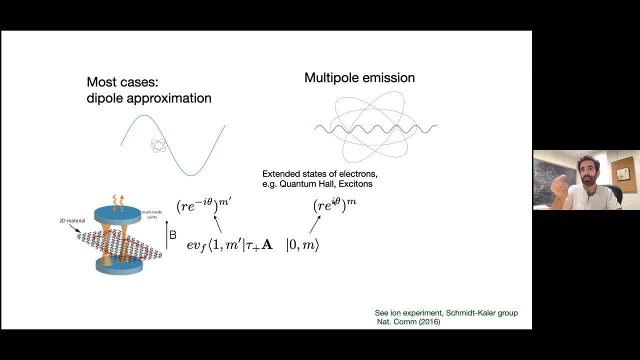 and the zeta levels, and the zeta is the radial position and theta is the angular degree of freedom, and m is some integer the same for the excited state, they're just the same. and then the a can be described by some bezel function or laguerre-gaucian field that has the right. 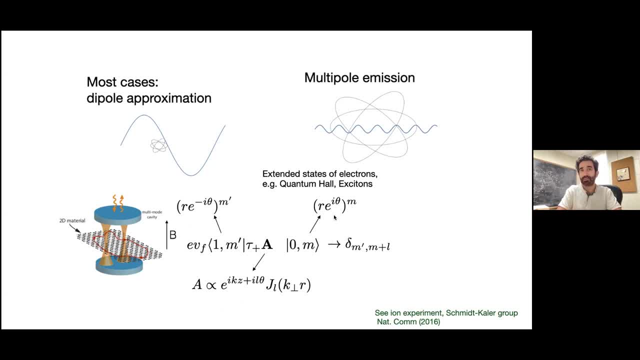 symmetry, you see that you have immediately dipole selection. this is a transition selection rule that m over here can absorb a non-zero orbital angular momentum of light and then go to another m, which is uh. m prime should be m plus l, and usually this l if. 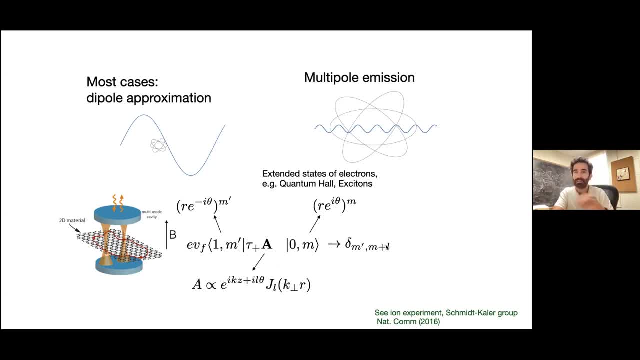 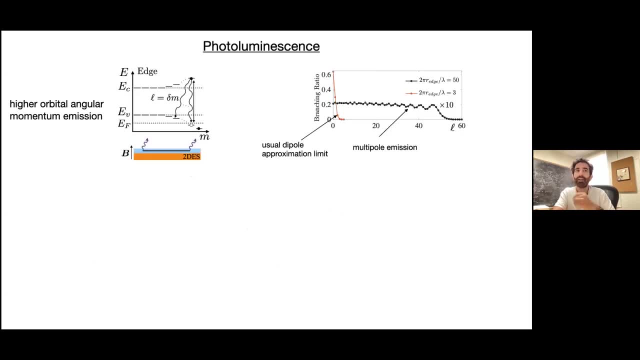 it's non-zero, if it's sorry, if it's uh, if it's one or two or three, this expression becomes very, very small, because the radial overlap is very, very small. but it turned out that once we calculate this, you get the branching ratio as a function of this multiple, this, this orbital angular momentum. 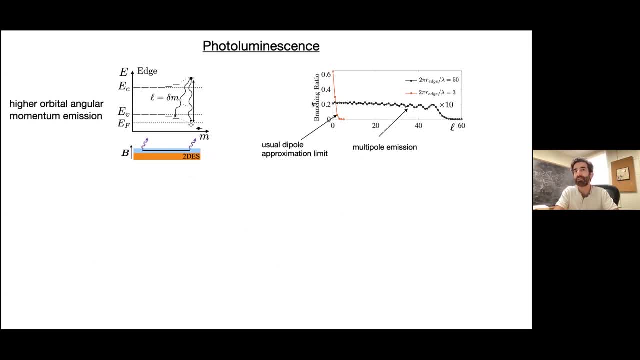 of light, and then you can see that it kind of stays flat and then at some point it decreases. so in a usual case, when you have your sample much smaller than the wavelength of light, you only get the l0 term, but then uh, and then it immediately goes down. if your sample size is is comparable to 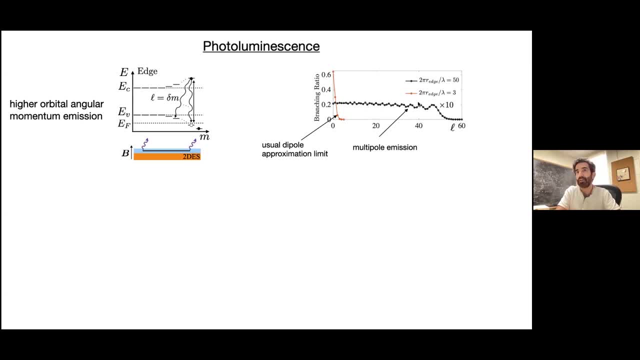 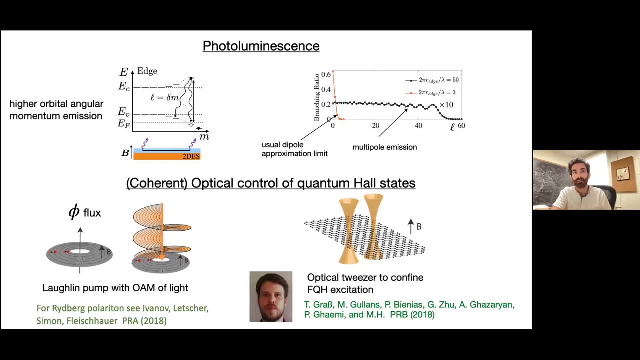 the wavelength of light. but if your sample size is larger than the wavelength of light, then you can actually have this non-zero orbital angular momentum transition and you should deviate from dipole approximation and this should be seen in an experimental setting so that more carefully we have looked into the system. 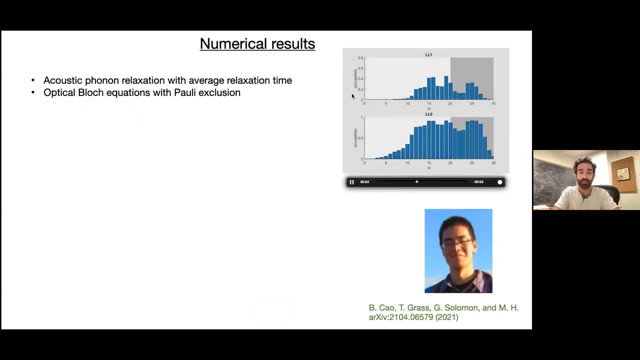 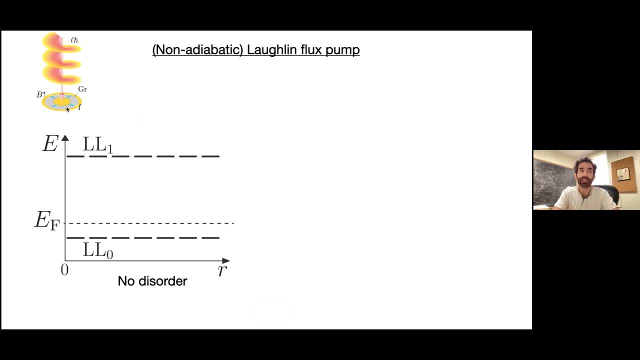 whether this one can actually do a photocurrent measurement by basically shining an orbital angular momentum of light to a sample and then look at the radial current that it's produced in the absence of any bias, because photons impart, are imparting their orbital angular momentum, and then 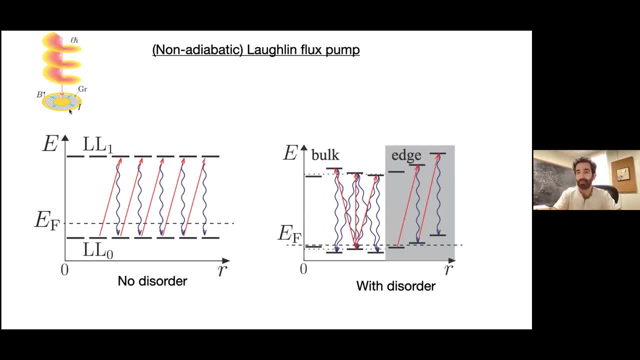 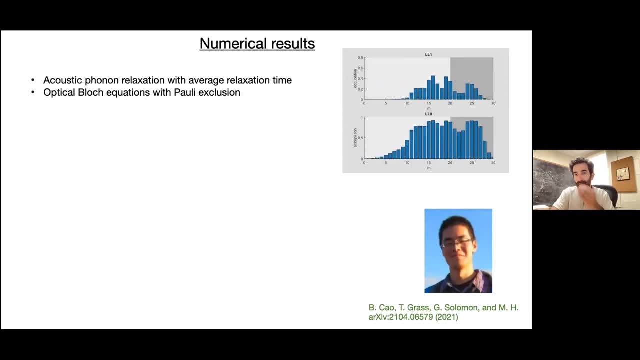 increasing the size, the radius of the electronic wave function. so this would be like a very macroscopically uh manifestation of uh how we can deviate from doppel approximation. and then our understanding of light matter coupling is- is not as, as we thought, another one that we was. 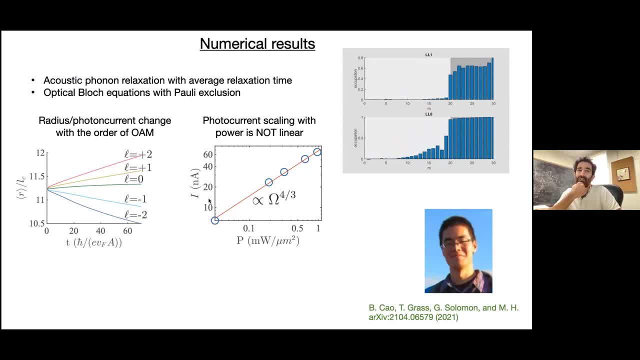 confusing was that the, the observed photocurrent as a function of the power, should not be just our unusual pump, optical pumping rule, which is which scales with the square of the robbie frequency. it squares, actually, it scales with four, um, uh, four over three, and then we understand why this is, and so hopefully there will be an 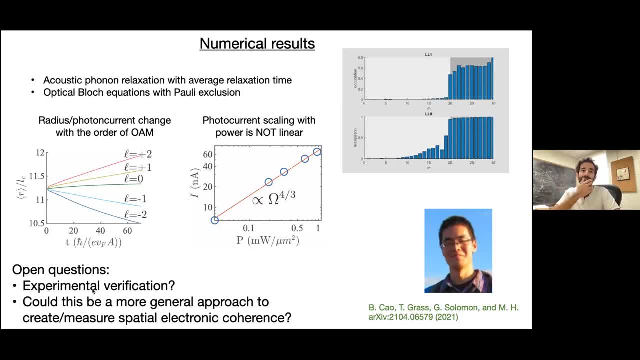 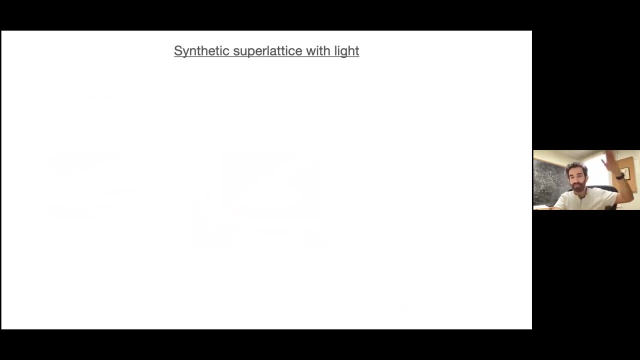 experimental verification of this uh and uh and even more general approach to measure this. maybe this could be kind of generalized. it's an optical way to measure and control the spatial electronic code. it's just sort of looking at what what thisけど says, exactly how many my 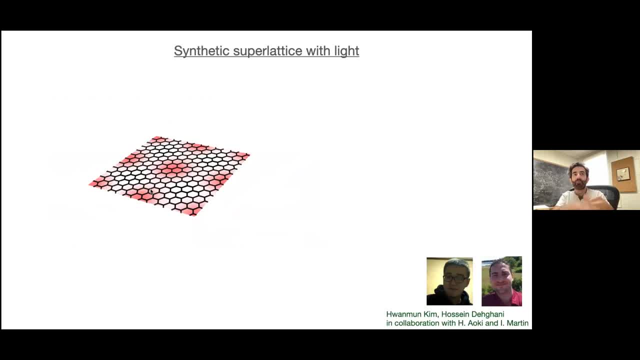 uh are passively made and we were wondering whether light can actually create them, because some of these super lattices are large like 10 nanometer, 50 nanometer, maybe even 100 nanometer, and even optical field can be something like a 200 nanometer is not crazy, it's still. 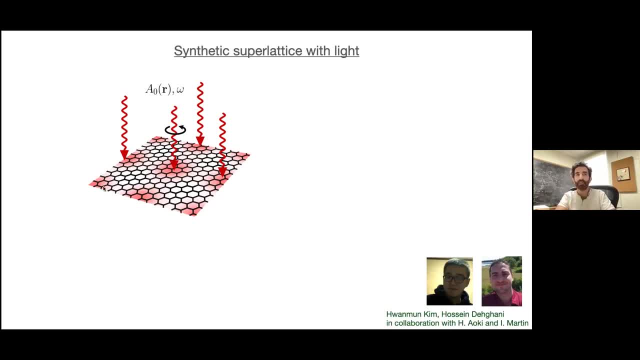 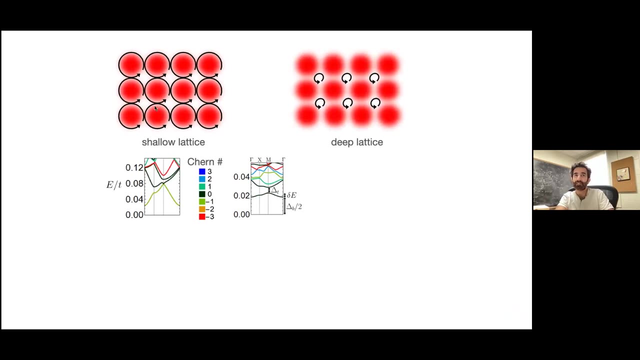 sub wavelength limited but 200 nanometer is not crazy. and we were thinking how we can use pattern light to change the underlying Hamiltonian of the system and then look at different properties, basically having like a square lattice changing the intensity of light, going to a topological insulator or not topological insulator depending on the intensity of the light, or making 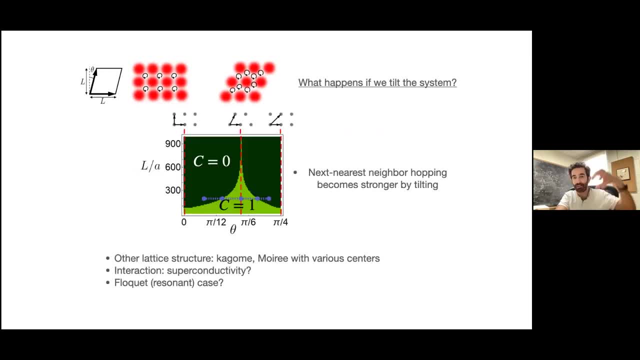 making a tilted lattice or a Kagome lattice, etc. basically was inspired by this experiment that people have been doing on Rydberg and called at them: using a special light modulator or any kind of light patterning, can we import them to, to electronic systems? and 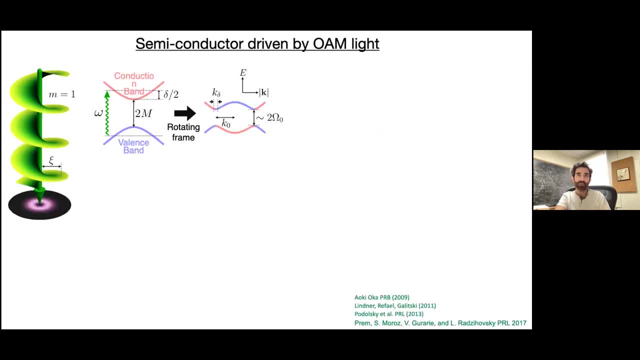 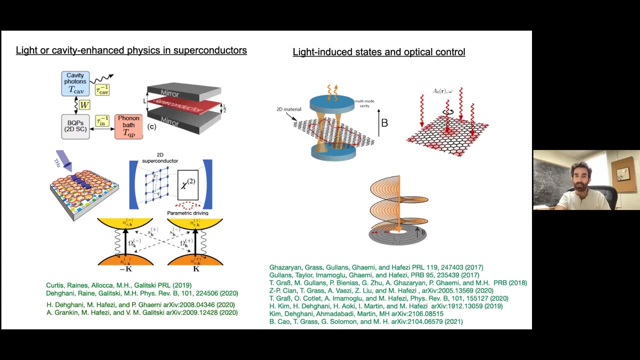 and make them happen. so with this, I would like to thank you for your attention and summarize: this is some bunch of the references that we've been working on and then we can. we can chat about, like the future, and I was given a list of things that I have to. 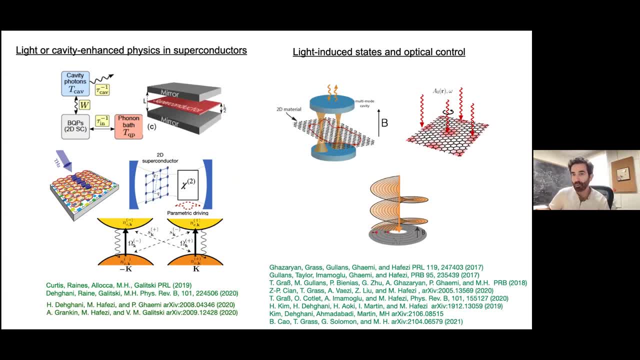 think about the near near-term goal and the future goals, etc. and I have some slides on that we can chat. thank you all right. thank you very much, Mohammad, it was a wonderful talk. do we have questions from the audience? so what can you maybe come back on the? I'm not sure I understood the platform on which you are. 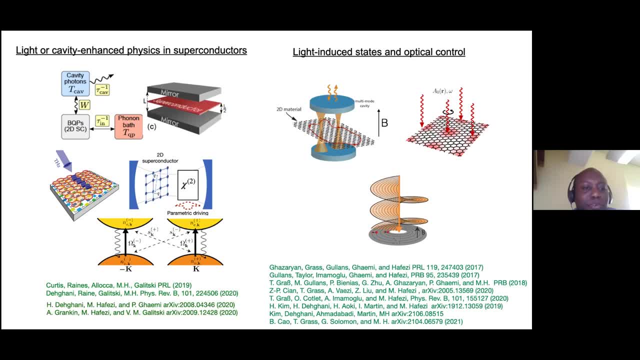 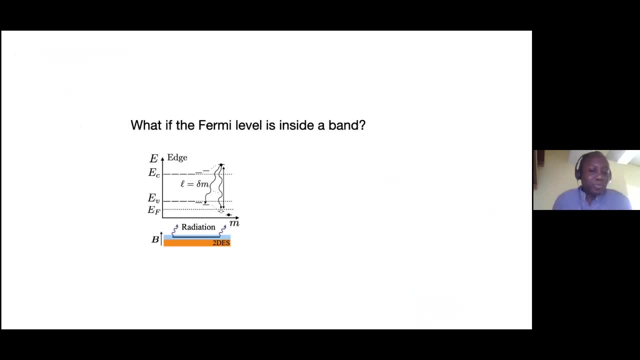 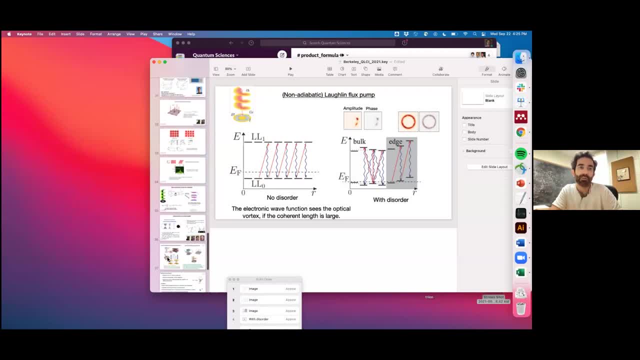 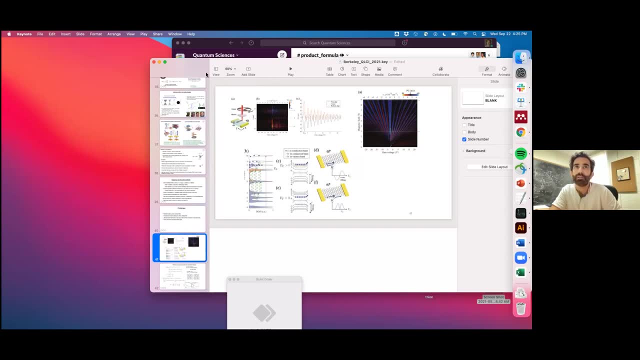 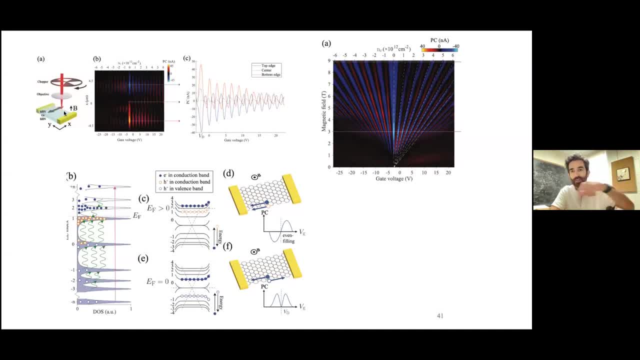 light, uh, in the quantum hall regime, depending on which part you're actually shining light, the the current can go in one direction versus the other. yeah, this is polarity. so that that was kind of understood and we kind of did that experiment to to, yeah, warm up as a kind of as a warm-up, but then, uh, the idea would be, do it with you know what is the. 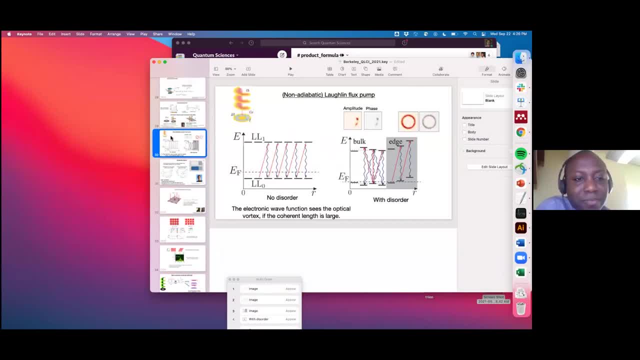 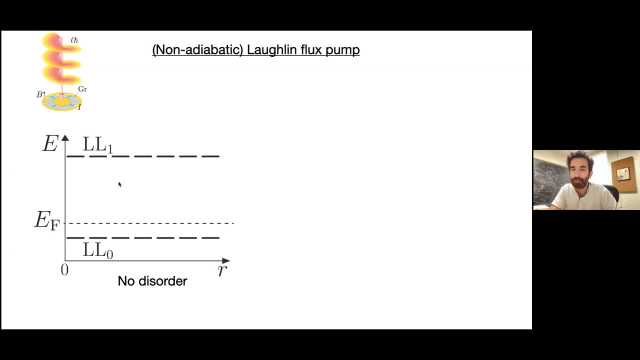 value of the b uh. in the experiment it can go from zero to uh 12 tesla. yeah, bigger is better, um, but that's so. this one will be similar, but in a corvino geometry, such that the whole point is that the electron should appreciate the orbital angular momentum of light. 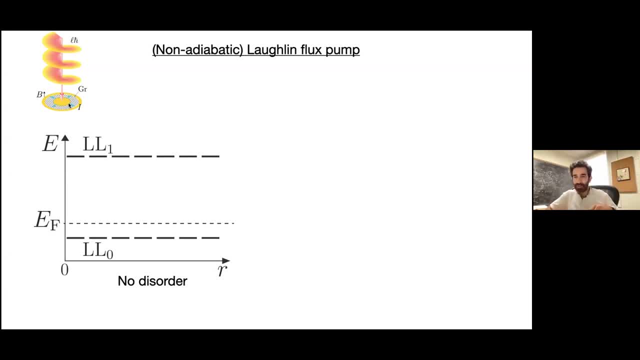 so um you're. you're an expert of orbital angular momentum, so, like I, I have this zero uh um. so if, if my electronic wave function winds around this orbital angular momentum, it is uh light. with OAM, I can actually appreciate its, its vortex. otherwise, if I have an OAM, 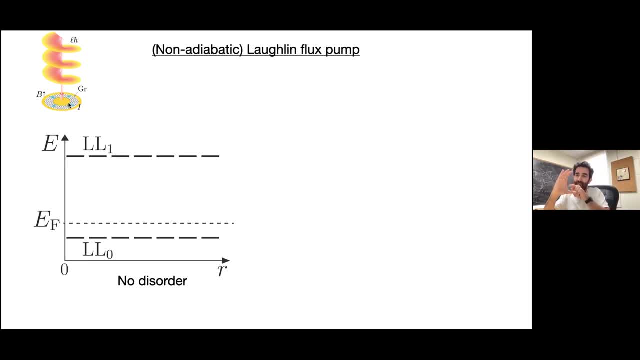 I like a larger gaussian field like this and my electronic wave function is circulating on the tip of this. it should not care about the orbital angular. orbital angular momentum is is origin dependent. it's not not like momentum. so it really matters that the whole of the orbital 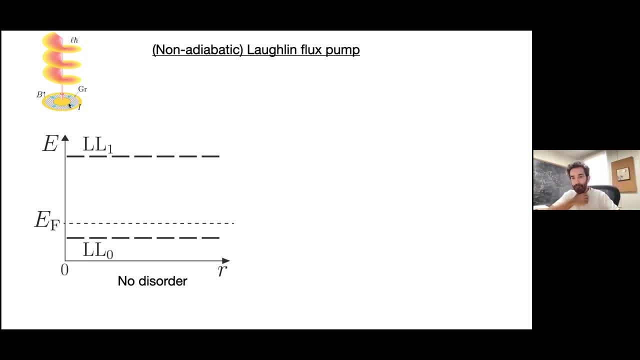 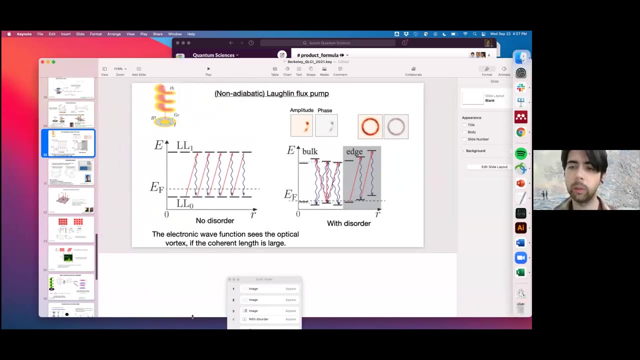 angular momentum and whole of the electronic wave function coincide, and one just way to do it is to do the corvino um. so we have one question in the chat which is from uh um, and the question is: uh, has there been uh experimental implementation of the induced superconductivity? 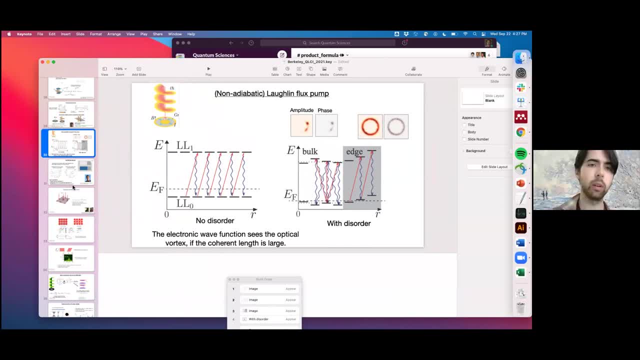 and if not, what are some of the limiting factor? factors, uh, against realizing this? uh, the limiting factor is: uh is not known. so these are the kind of the challenges. so one is the one question is also that there are some proposals to make pairing, but pairing doesn't necessarily mean superconductivity. 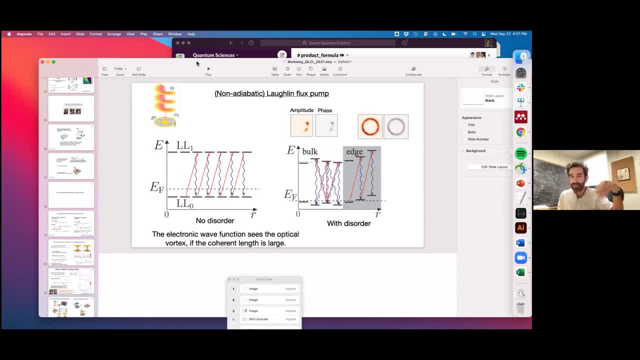 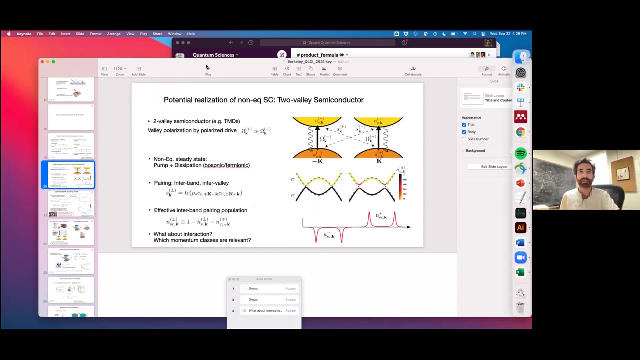 so maybe maybe pairing exists and people have have not been able to to measure it, uh, but that's kind of one of the issues is that there are these, uh, these proposals. I can actually tell you one of the problems, potential problems, with our proposal: maybe that makes it, that makes it more concrete, and that's the question of excitons. 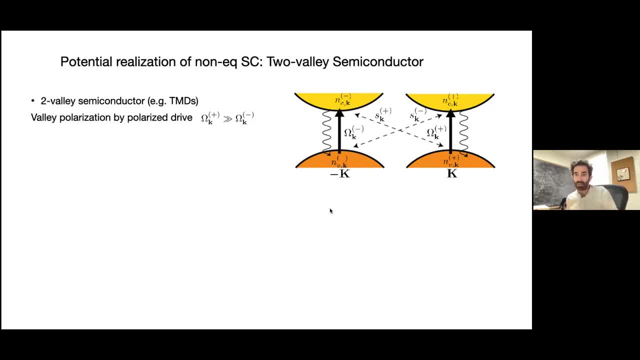 here we ignore the formation of excitons might be. uh, it might be. we might be competing with the creation of the superconductor. and also in the previous work it was also ignored in the uh in the proposal to make uh floquet topological insulator in uh. 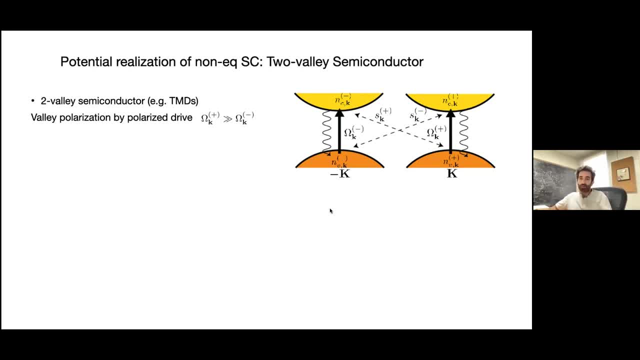 in semiconductors. the formation of accident was also ignored. uh, and that that's another problem. and now I mentioned the beginning of the talk- is that if you just look at the semiconductor and ignore coulomb interaction based on free carrier, uh, then you should not have any absorption below the band gap. but we all know. 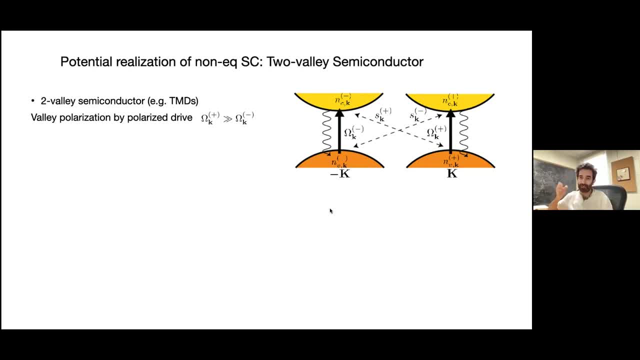 that below the band gap you have all these Rydberg series of excitons. you have to include the coulomb interaction. so then one uh at least with this proposal, would be that one has to compare the exciton channel and the pairing channel and then see which one would be more relevant. 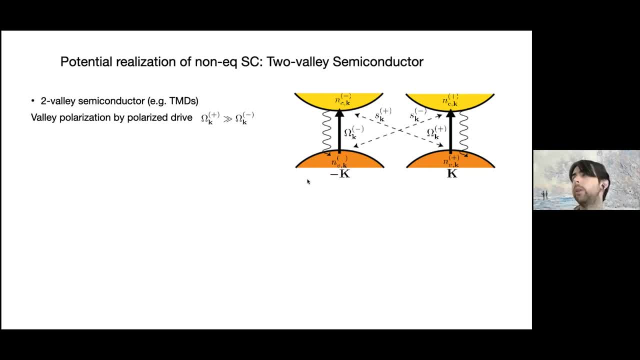 yeah, thank you. so I guess, along those lines, um so you have given a number of, you know, very inspiring, uh theoretical proposals, uh, over the course of your talk, do you have a sense of which of these is like the closest to to happening in in reality? sure, um so the, the, the deviation from doppler approximation, and this OEM, I think. 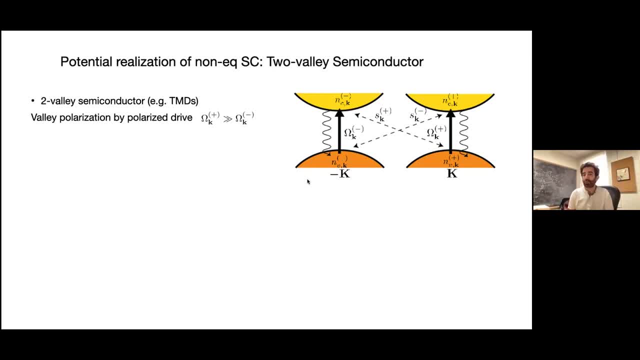 it's the one. I just uh chatted with, bubaker. I think that that's the closest one to the one that we're talking about. okay, so, yeah, um answer on the observation point. um, I think that's. uh, that's what i was asking for. my question is in the on the 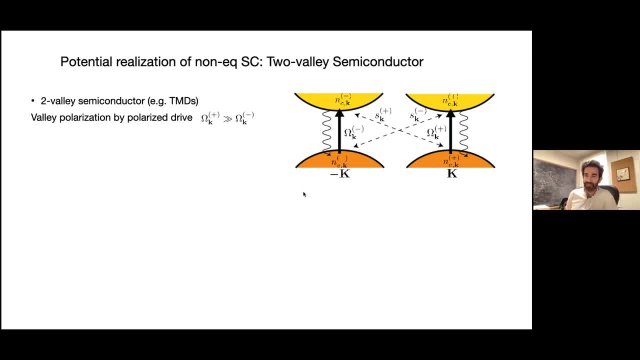 question: um what? how can we say that this is really the first program, um, that we're considering? and also, how does this work? is it possible that that, uh, this is a a problem where, if I said that in the end, you're going to have to do something different or you've got to, 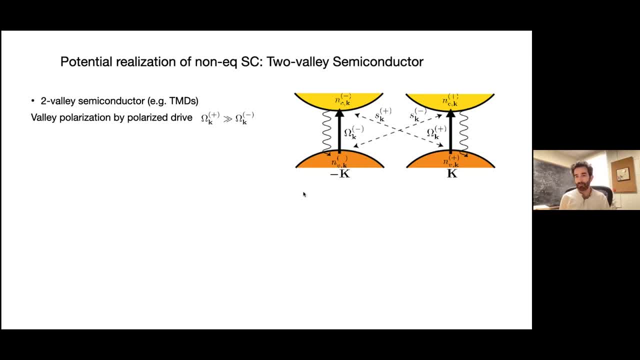 theoretical proposal from many, many folks, including Peter Zoller, Ignacio Sirac and company, And it was kind of go back and forth. I know there was this interesting theoretical proposal and then people will follow. So I think there should be a healthy amount of theoretical proposal- healthy. 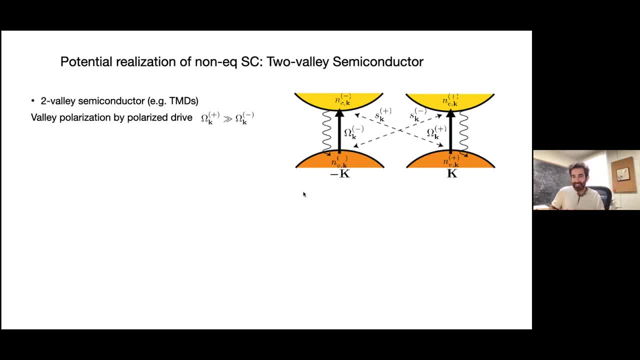 What amount is healthy? This is, of course, the community should decide. And I go back to the first slide that I have. We are now dealing with real material In cold atom. we are dealing with atoms, alkaline atoms, that we know them very well. 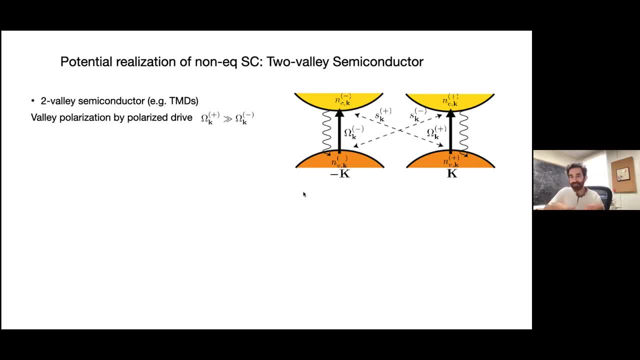 Their spectrum is very well known. Here we are dealing with electrons in a mess, So one has to be more patient. I mean, as you say, the problem is there are lots of competing phenomena And which one is happening first. So that's the old question. 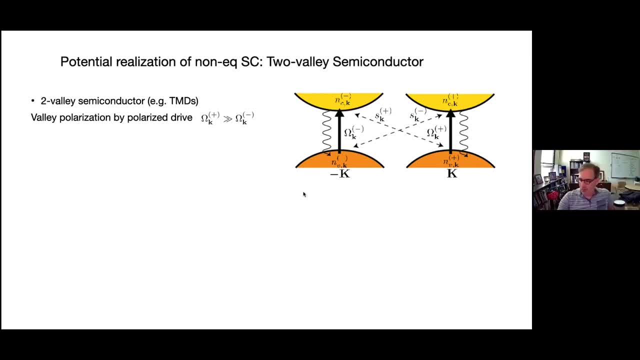 Mohamed, I have a question about like an intermediate topic which I've been trying to understand and read about, And then you mentioned Thomas Ebbesen, So that made me think of this. There's this: you know, in chemistry there are a number of experiments. 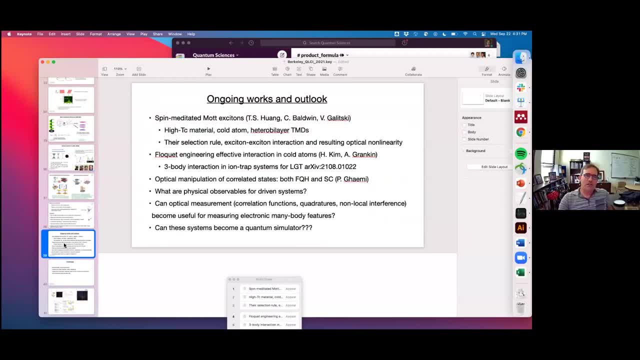 that consider whether chemical reactions inside of optical resonators, driven or undriven, might be modified in some fundamental way. Well, I guess what's your take on that body of work Like? is it kind of clear what's going on in there? 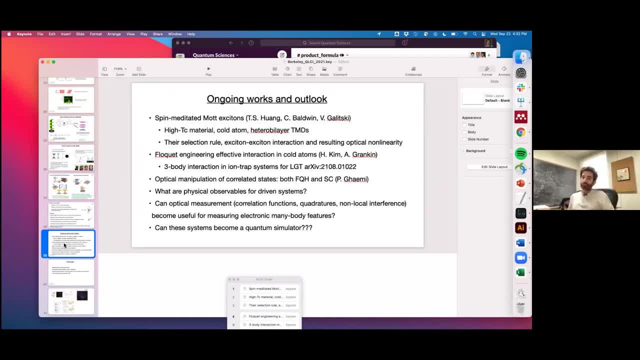 To me it's kind of unclear. And then is there a way to think of that as like a useful stepping stone to the kind of experiments you're looking at? Maybe what you're looking for is more robust in a large bulk system than it is in a 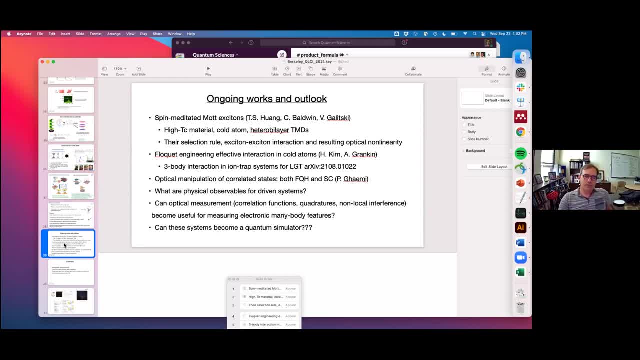 a mesoscopic molecular system. No, I think it's a beautiful experiment and a topic to work on Theoretically. I have not followed up very closely, but one bunch of theoretical words that I read and I could not understand was related to the fact. 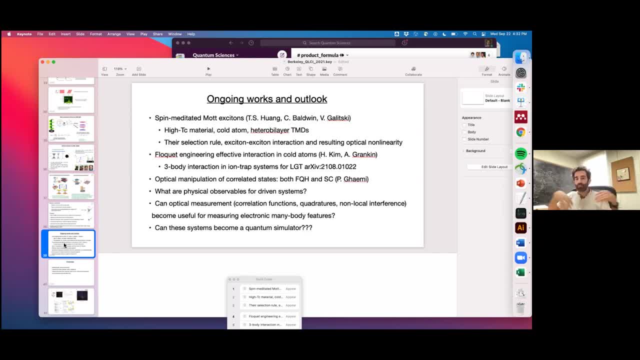 that we model it as a bunch of two-level systems that are coupled to a cavity. So this is my understanding. experts should comment: is that a bunch of atoms? so the transport is modeled by the following: I have a bunch of two-level systems. 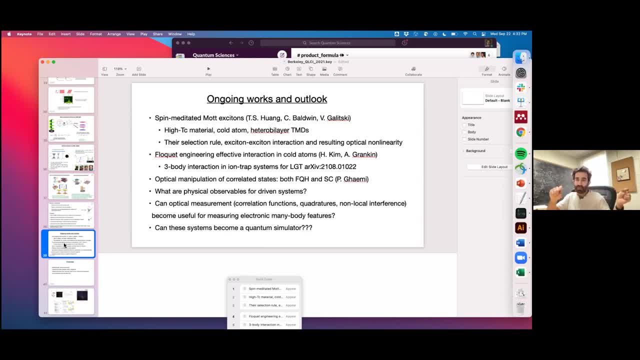 that are coupled to each other with some flip-flop, interaction, And now I coupled them to an overall cavity And now the electron would not be trapped because of the Anderson localization of these two-level systems. It would talk to this global guy, the photon mode. 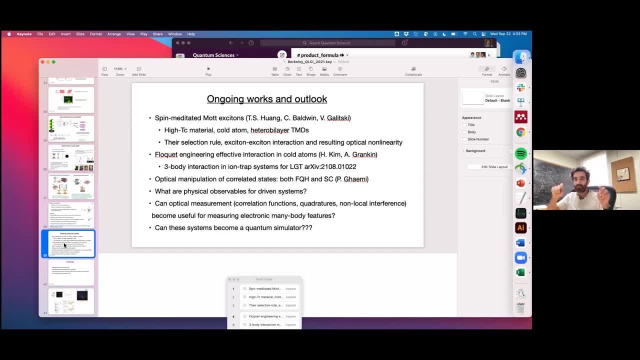 and then it would be enhanced. But then here we are ignoring the fact that this electron, if it's itinerant, it cannot be described by just these two-level systems that are talking to a cavity mode, Basically James Cummings model. it might not be actually the right model. 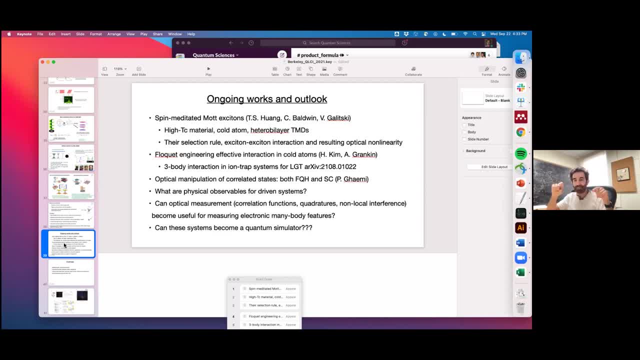 to think about that. I have to think about, then, a current that is coupled to the cavity, rather than a bunch of two-level systems, Right which you had that JA expression, so that would be kind of a right way to parameterize it. 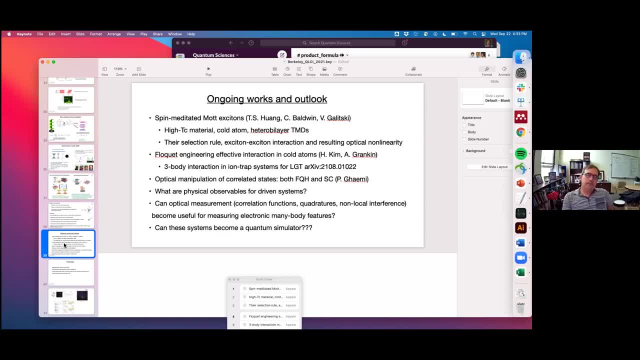 so I can see that Exactly exactly Now. can we have a toy model of the James Cummings Hamiltonian for currents, such that we can make sense of bad cavity with cavity limit et cetera? That's still missing. And no, those experiments are certainly useful. 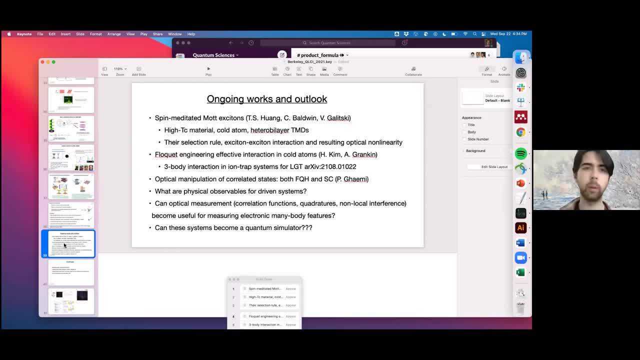 Are there more questions from the audience? I think I have a couple I can go into if there aren't One in the chat. I think nothing in the chat. So yeah, so this seminar is part of the CIQC colloquium. 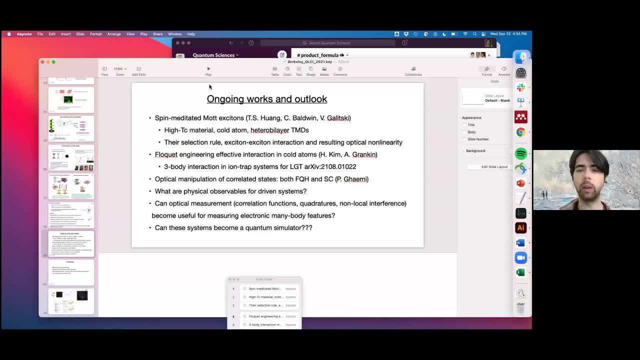 And the CIQC mission, as I understand it, is to address fundamental challenges for the development of the quantum computer. So could you remark, maybe, on how maybe some of these approaches might lead to new problems? Yeah, There are two ways of approaching a quantum computer. 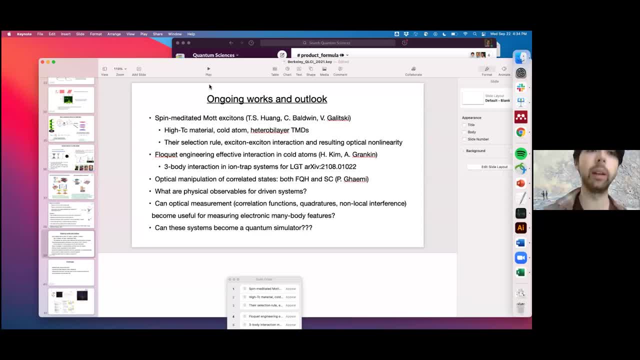 or maybe overcoming existing challenges in current approaches for quantum computer. How does this cavity plus correlated electron physics fit into this sort of picture? Yeah, so I don't usually have a mission-oriented research. whenever a problem is interesting, I will think about it. 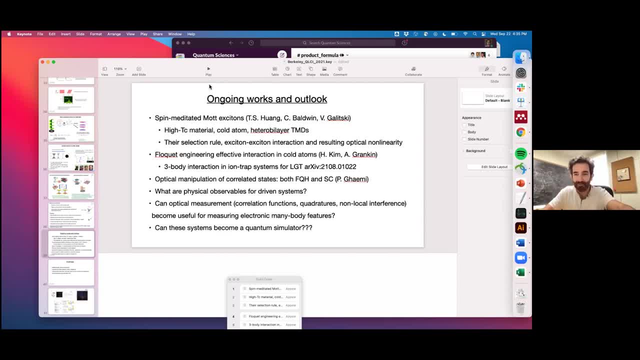 And although my name, my first name, suggests that I might have some prophetic vision, but that's not the case. I don't know how this will have an effect, But at least I can tell you some of the stuff that happened, Like this: three-body interaction in ion trap. 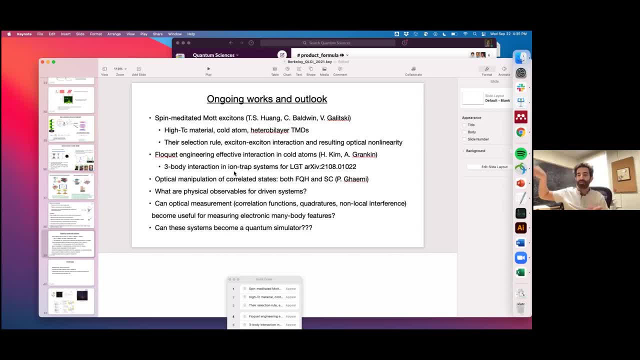 was something that we were thinking about like floquet, driving the system and then effectively making three-body interaction. But then I realized, with my colleagues Zohreh Daudi and company, that well, it actually can be done with ion traps And it might be useful for some lattice case theory. 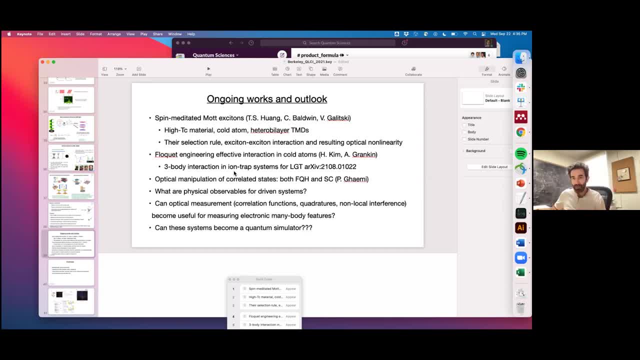 implementation. So some of it might be actually at intellectual level, not necessarily at an experimental level, That some of these techniques that we want to use- how to use light to manipulate the non-interacting and interacting part of my lab, My Hamiltonians- directly has an effect on quantum simulator. 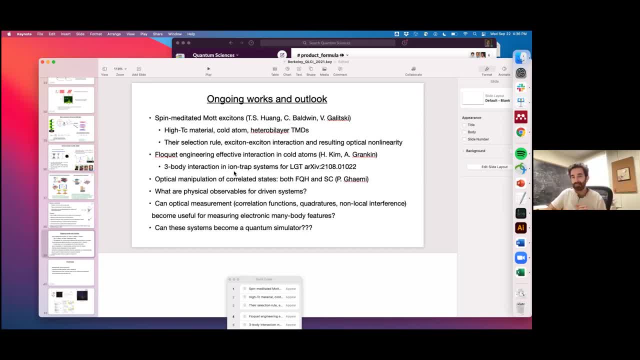 If we learn how to do them with atoms in a cavity, in the cold atom, we might be able to learn something from that for electrons in a cavity. So that's kind of one thing. The last one that I put is that: can this system? 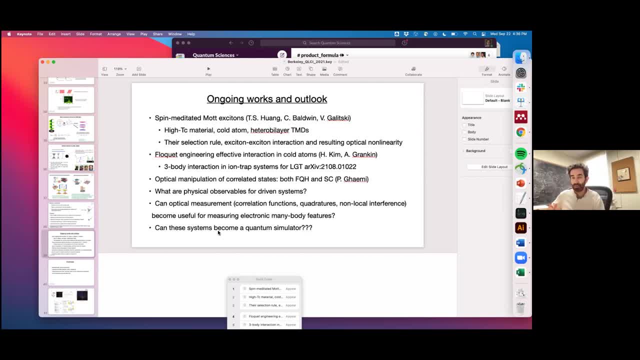 become a quantum simulator at some point? We don't know. I mean now we have a huge body of work on moiré physics, a new development Just in the past five, 10 years, And it has exploded. Can the purity and the disorder and the quality. 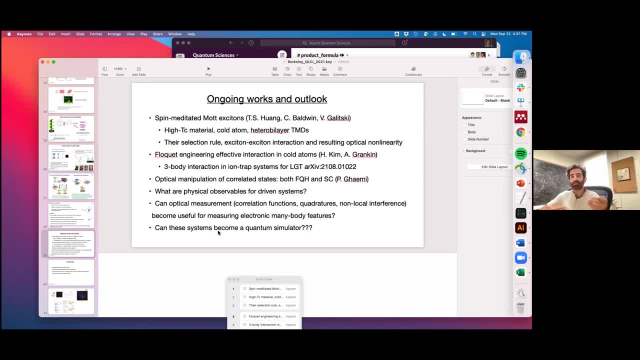 of the material come to a level that we can treat them as individual states and manipulate them and look at the collective effects. Maybe, maybe not. Another intellectual one I would say is: I said the one third of my group are working. 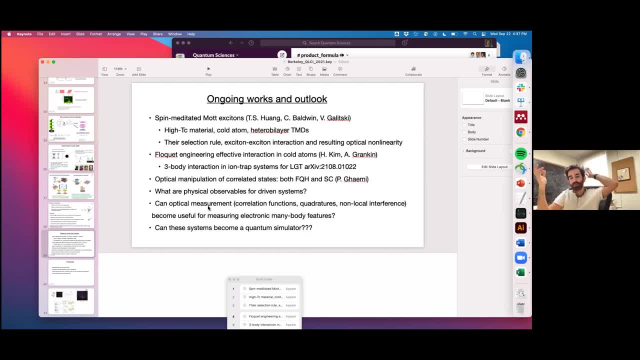 on how to measure, How to measure many body features in a quantum simulator in an efficient way. You don't want to do full state tomography every time and we had to spend an exponential amount of time measuring it. If I'm interested in some order parameter, 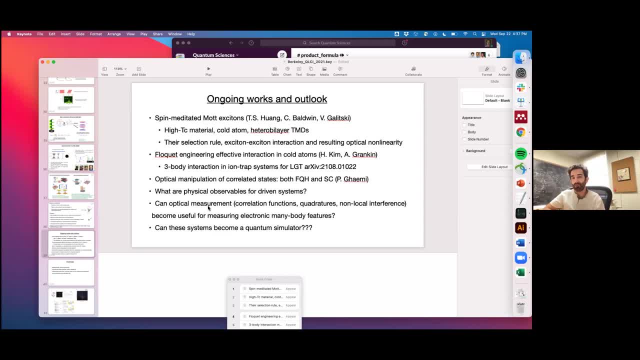 if I'm interested in some topological invariant, can I measure it more efficiently? I think answering those might be related to answering whether we can do it with photons in an electronic way, If I have a bunch of spins in a quantum simulator and I want to measure them collectively. 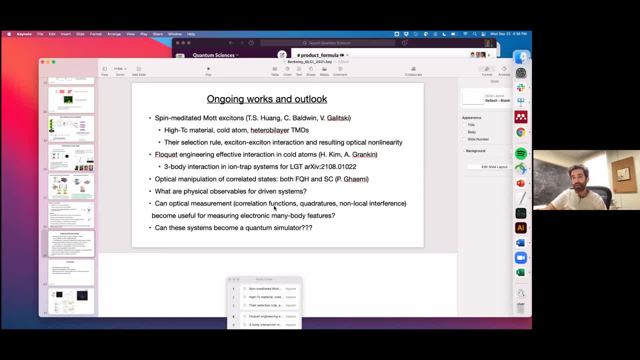 maybe we can do it with the same electrons. I decided not to give the quantum verification and measurement talk for the QLCI because I thought that it would be a nice semi-orthogonal topic. This topic would be a semi-orthogonal topic. 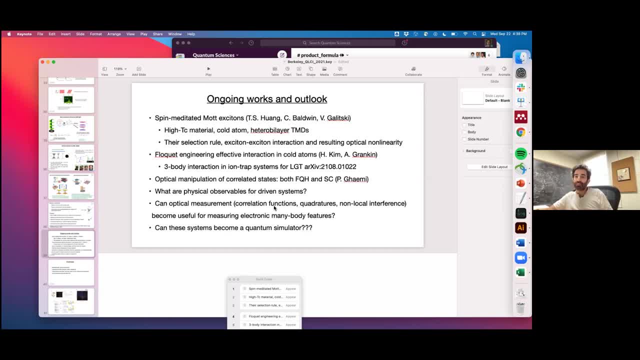 to the QLCI, But it is not really So. Yeah, So in that part we have a lot of ideas how to use an ancilla like a global mode to prepare and measure many body states, And they're kind of the same thing. 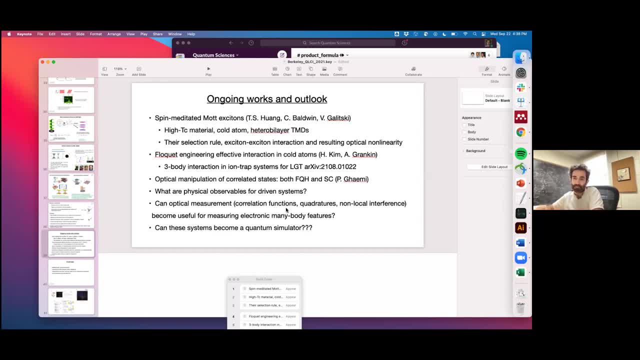 when you might apply them over here, I guess. just one last question for me. So you mentioned very briefly this light patterning on top of the graphene and how you can make various lattices like square, triangle or cognate.